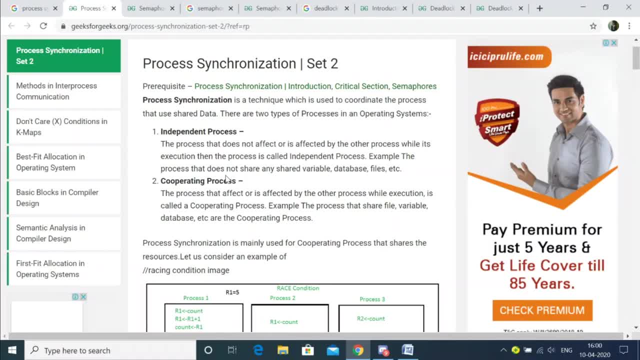 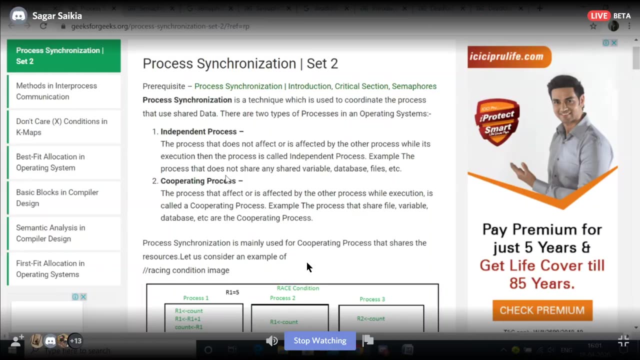 Now, in case of co-operating process, it is a kind of process where the execution of one process will affect the other, So there is a dependency among Okay. So whenever we are, whenever a process, one process is executed, so that execution will have an impact on some certain other process. 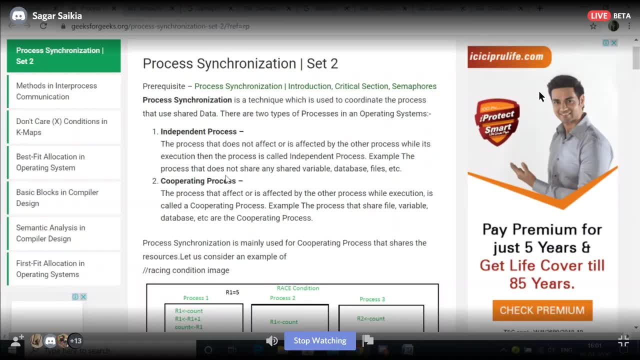 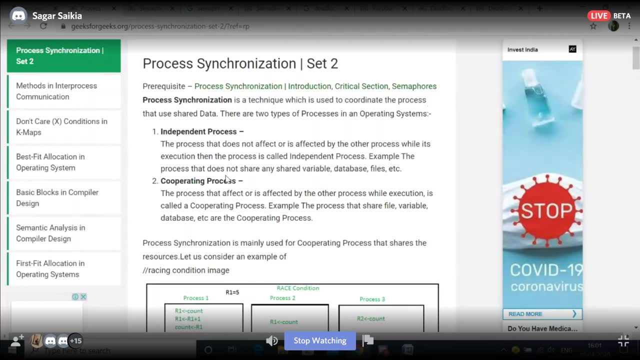 Now why is it so? The main reason for this is because they share various elements like variables. It can be memory, It can be a part of the code of the program. That means a program A part of the code of the program. 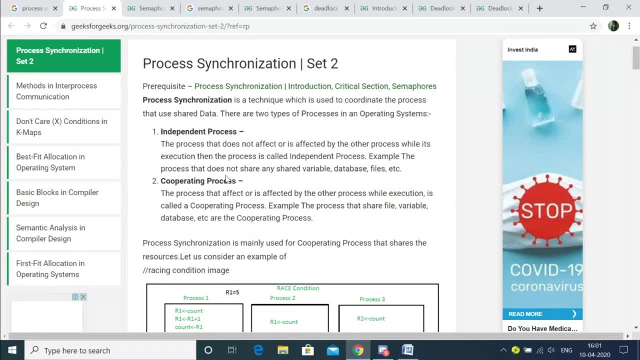 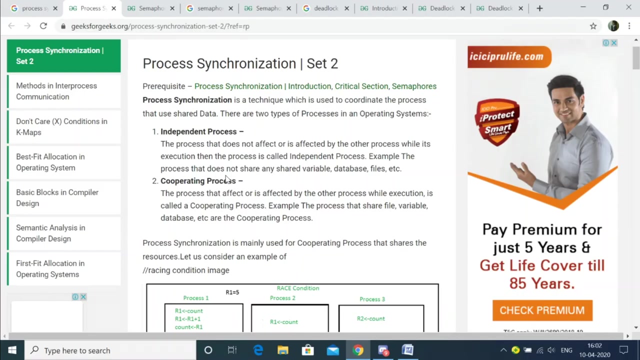 Okay, A part of the code of a particular program may be common for two different processes, So that may occur some kind of inconsistency, So that basically we have to overcome okay. Also, sometimes if we are sharing certain resources, like for example CPU, printer or hardware elements, then that time also there has to be a synchronization among the processes. 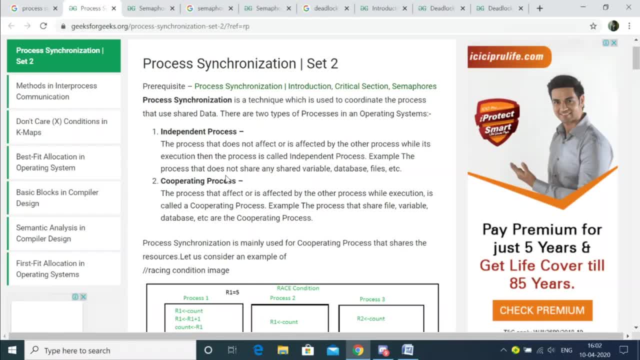 Okay, Otherwise, whatever the output we are supposed to get, that will not be achieved. Okay. So, for example, here they have given a code. So this code I have simplified and written here. So let us say that we are having two processes, P1 and P2.. 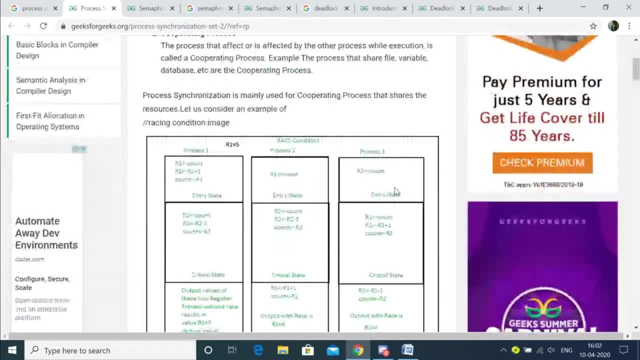 Okay, So this kind of a code snippet, Now here at the, at the top, if you can see, here there is a code snippet And now what we are not going to do is we are going to do a single code snippet. 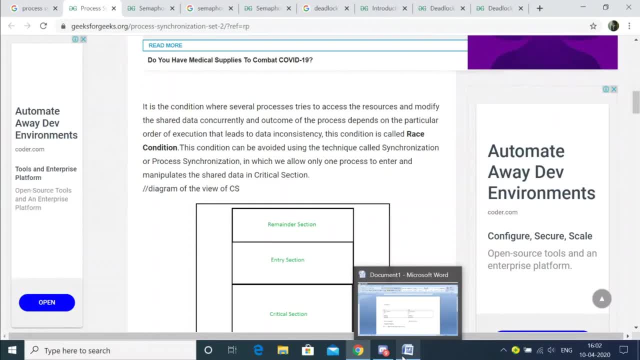 Now let us say that the code that we are adding here to the result is not equal to the code that we have added. We have added thehelping. I will pause it. We are adding a single code snippet here Now. let us now look at the code snippet. 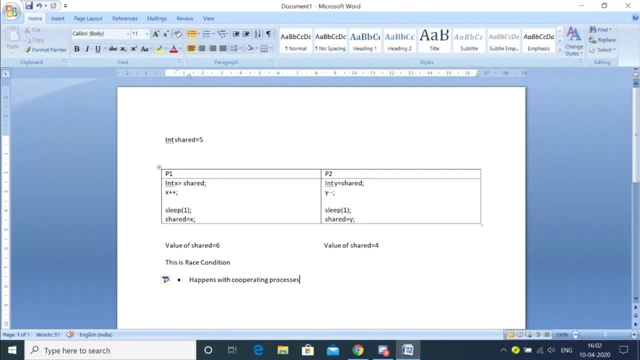 So the code snippet two processes, p1 and p2. okay, so it is kind of a code snippet now here at the top, if you can see, here there is a global variable. this is a global variable. so we have a global variable, shared, called shared, and its value is assigned to be equal to five. okay, now, at this situation, let's. 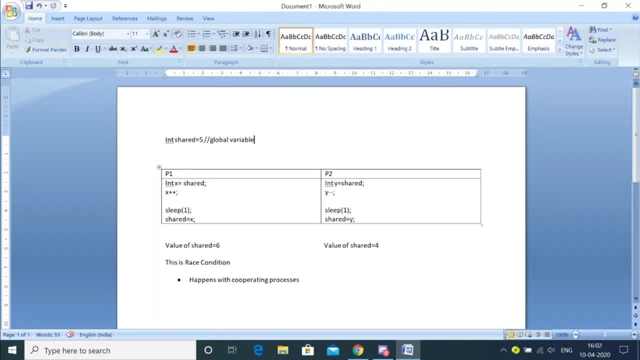 see for process p1. what is it happening in process p1? so here, x is a local variable under p1 and it is getting the value of shared. so what is the value of shared? what is the value of shared? we know that shared is a global variable and it is having value five. so under this, under process p1, we 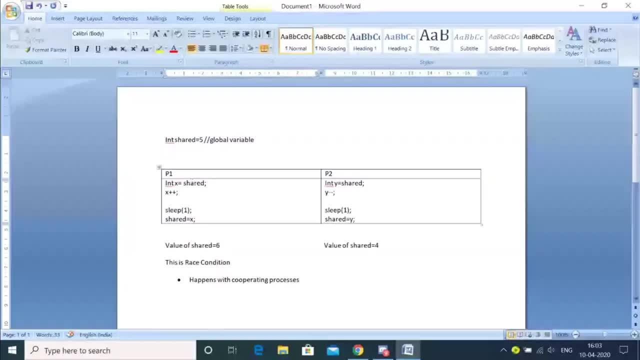 we are having certain codes. so first instruction: what do we have? we have int, so x is a local variable and it is assigned the value of shared. so shared, we already know from here what is the value of shared. the value of shared is five, so five will be assigned in x. so x here is equal to five. so i can comment maybe, so here i can say x is equal to five. okay, now in the second line of instruction, what do i have? i say x plus plus. 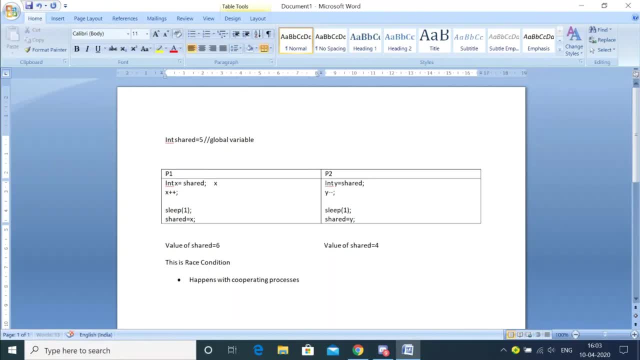 that means x will be incremented, right, isn't it? so the new value after si, after incrementing, what will we have? x is equal to six. okay, so let me comment here. okay now, third instruction. that means i'm calling a function which will basically suspend this process. p1 for maybe. 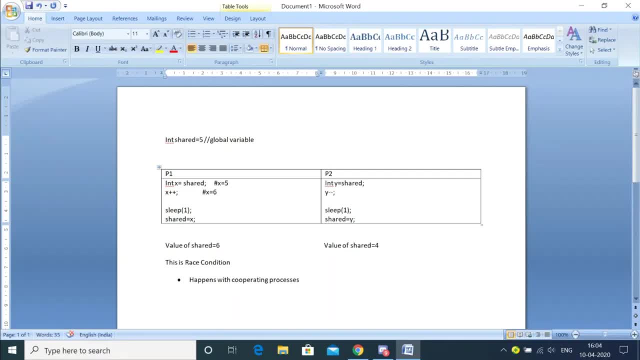 for one unit, others time it may be one minute or one second, and then if this part of the process will be sleeping, that means process p1 will go for sleep. it will be uh preempted, there will be a suspension. so the moment uh, this is uh executed, the moment this, the third line, is executed, so what will happen is uh, basically. 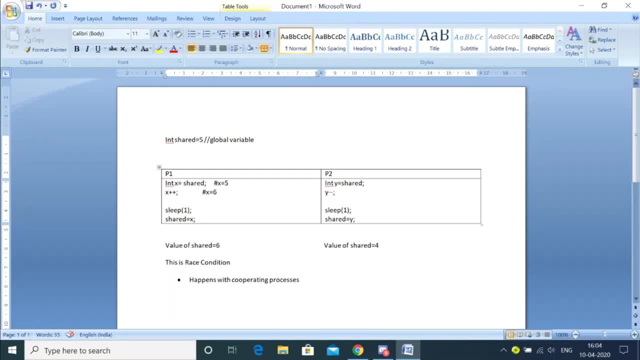 there will be a kind of suspension. so that means process p1 will be halted for some time. suspension of p1 for one second, okay, so after this, what will happen then? the uh operating system will check that. do we have any alternate process which is waiting? yes, we do have. so what? 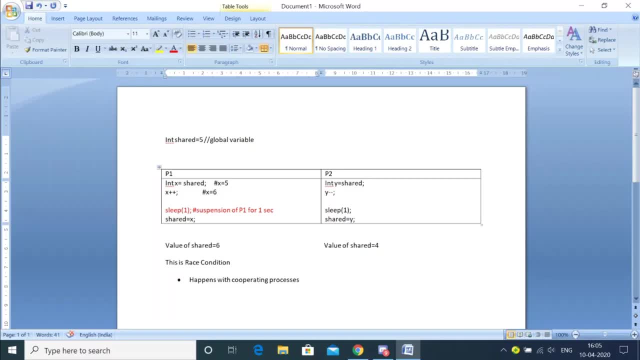 is the uh alternate process, p2, so the control will come here. that means this p1 is suspended and we are giving the control to p2. okay, so this switching from one process to another is known as context switching. now again here, the first line of instruction. what does it say? 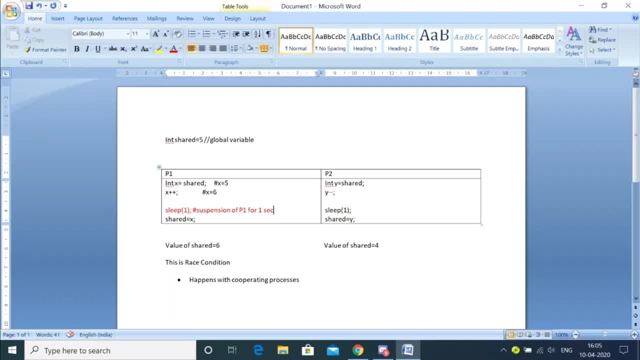 integer y is equal to share. that means y will be assigned the value of shared. but shared. i already know what is the global variable of shared five. so here i'll have: y is a. y is assigned the value of shared, so y's value will be how much five? okay, then y is decremented. y is decremented, so. 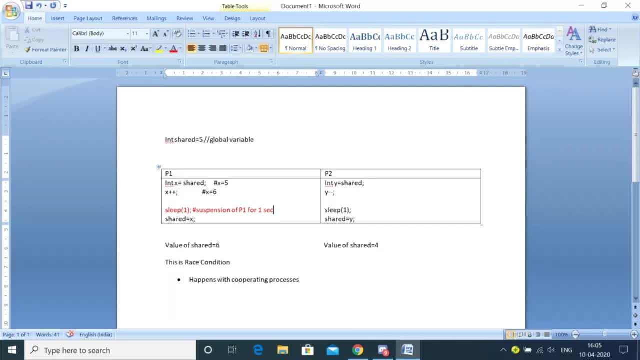 y's value will be 5.. so the function of y is 5.. that's, the function of y is 5, and then y will be given the value of five. so y is given the value of five. so now, what will be the value of five? y value will be four. okay, then again in the third. 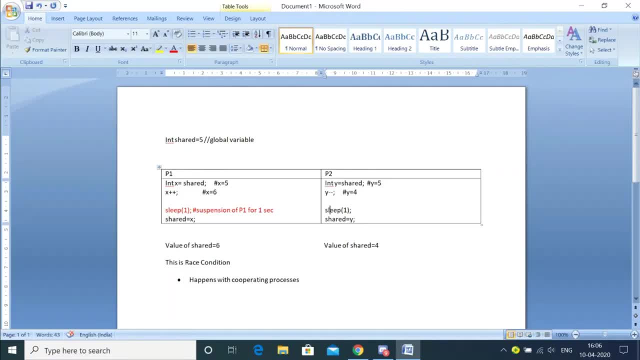 line of instruction. what will happen? uh, we will encounter sleep function which will suspend p2. so this again same thing. so it will suspend p2. for how much? for maybe one second or one minute, and depending upon the unit. so this will again go for suspension of the function. 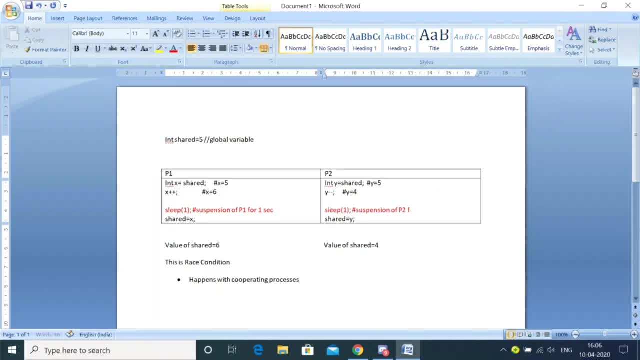 of P2 for, let's say, one second. So this is suspended. that means P2 will not be executed. So again, there will be a context switch. that means it will come here to the fourth line, because the other three lines of P1 are already. 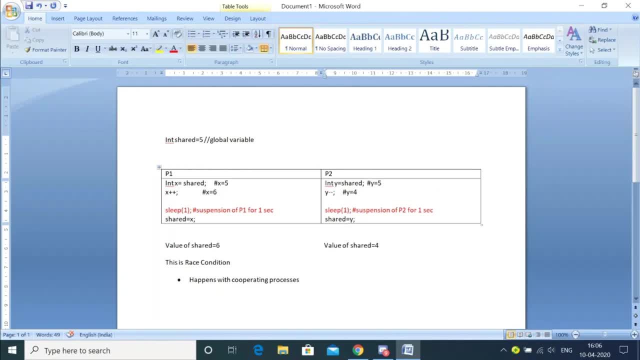 executed. So now, what is the fourth line saying? It is saying that share will be assigned to the value of 6.. So that means what will be the value of share now after the after this execution of statement So X? we already found What is the value. 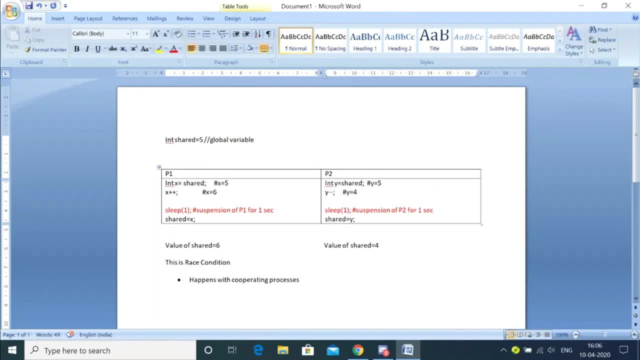 of X here 6.. So 6 will be stored inside this one. So we got from this first instruction said that the value of share now has become how much From 5? what did we get? 6.. So this line is: 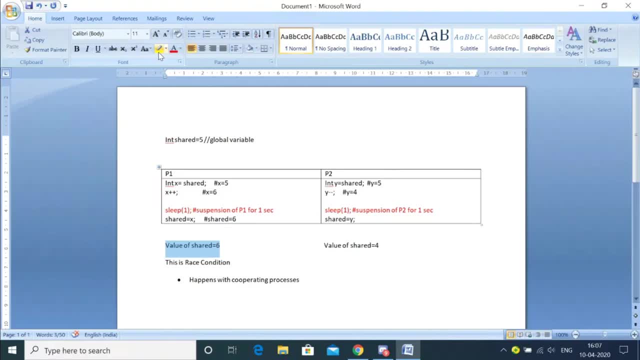 executed Now. when this is over, then P2 is still yet to be done. It has not finished. So what will it do Again? there will be a context switch here. This is done now. P1 will not come anymore. So shared is assigned to Y. 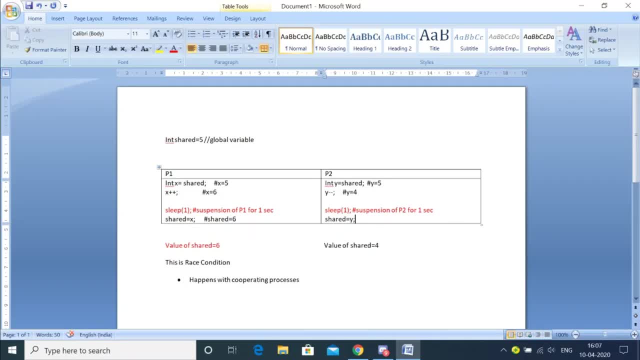 So that means again shared in P2. shared is updated with something else, So is it the same or different? Let us see. So shared is equal to what is it? Shared is equal to Y, But what is my Y? So Y is 4.. 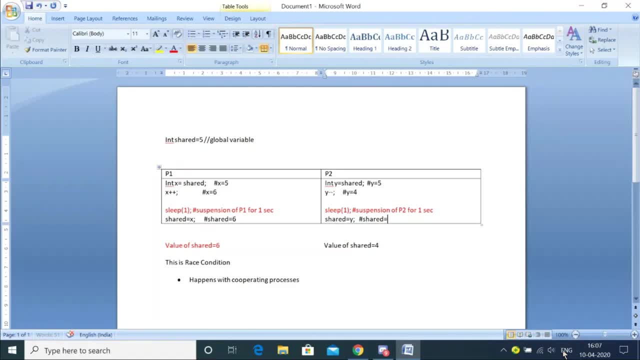 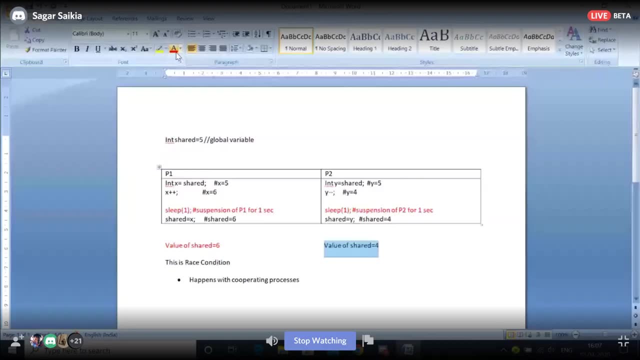 So ultimately, from here, we are getting the value of shared to be equal to 4.. Okay, Now, what is the problem here? When I compare, this results: Okay, So what will happen is, first of all, this value 4, this value 4. 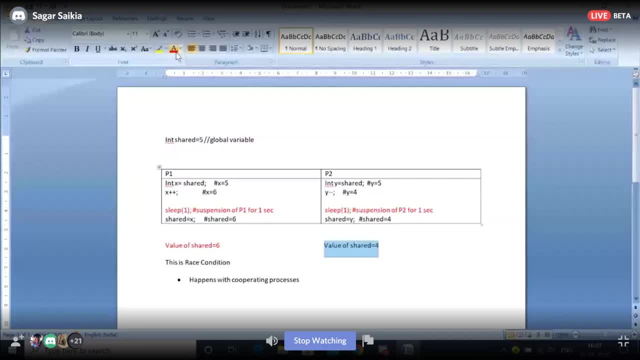 is it correct, This value 4. Is it correct? No, Why? Because initially we were having 5.. 5, if we see here, 5 plus 1 is how much 6.. There was a context switch. It went. 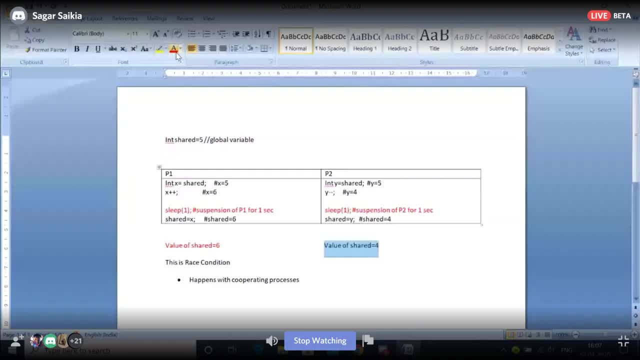 there, Okay, And there was a decrement of 1.. So 6 minus 1, it should have been 5.. Okay, That means this should have been 5.. But we are getting 4., Isn't it? So now what will be? 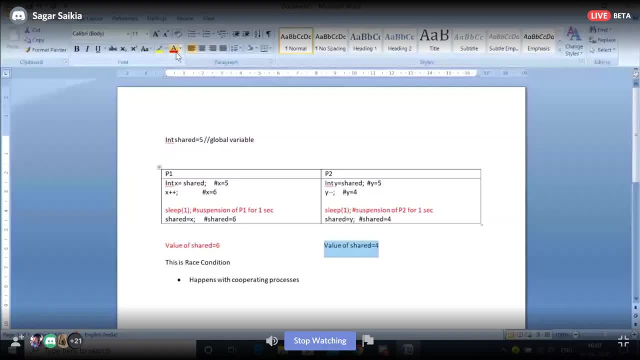 there There will be an anomaly because correct result was not found. So why this happened? Because there was no synchronization between the two processes. Okay, One is sleeping, The other is coming, The other is sleeping, The other is going, But there is no coordination. 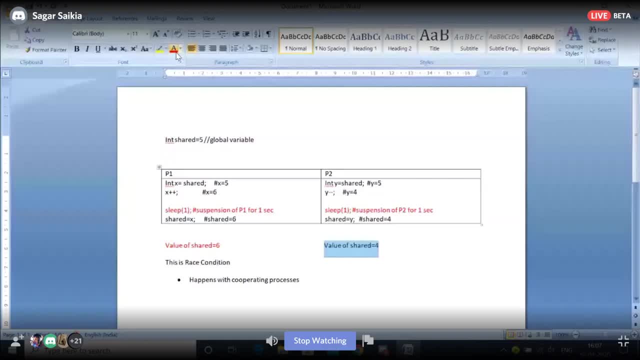 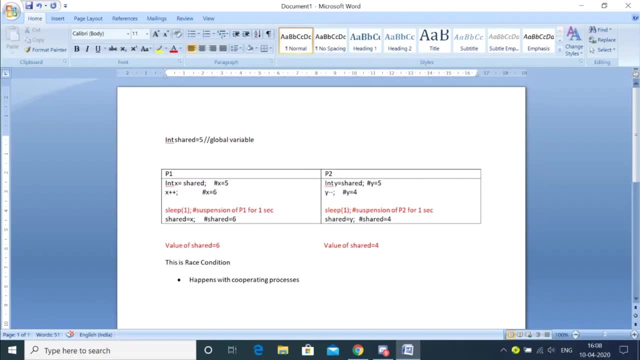 among the two What is happening? The two they don't know, Or there is no synchronization. Okay, So such kind of situation where if you see here both 4, 6 and 4.. The value of share That is 6 and 4.. 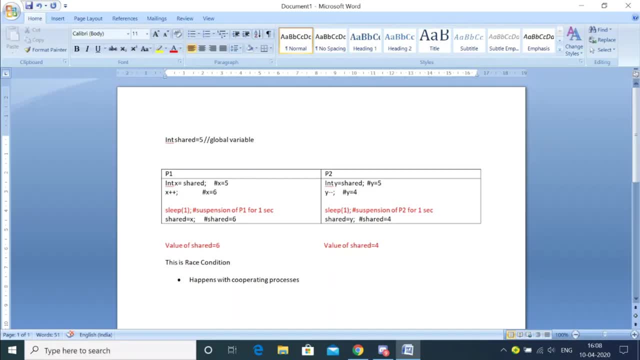 Both are competing, Or you can say are racing. Okay, Like who will be getting the ultimate? you can say who will be considered as the ultimate output. So this condition is known as race condition. Okay, So this basically happens only with cooperating processes. Why? Because 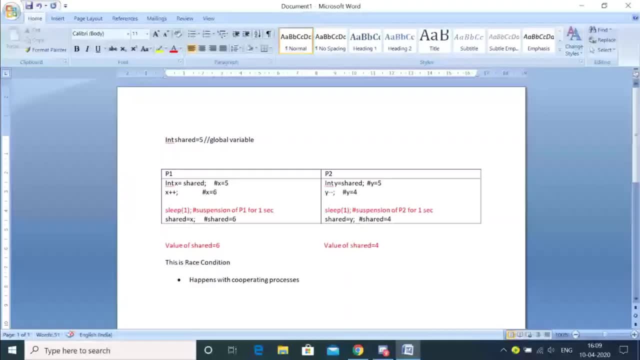 there are certain things which are common. So here what was common, that shared variable was common. So that's why, whenever we are dealing with common things, then that time, whenever updation takes place, there may be an anomaly, Like in this case it happens. 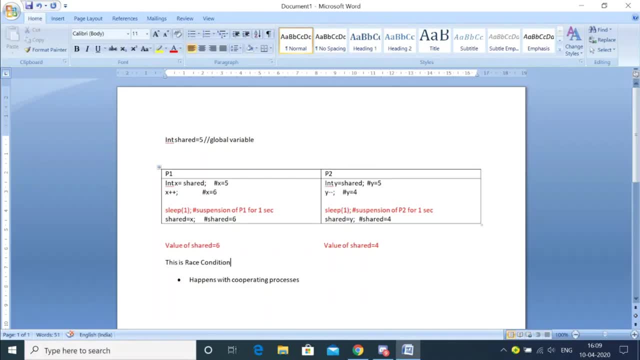 Okay. So if we execute such kind of program, So we will see that in certain operating system we are getting value 4. In certain cases we are getting 6.. Okay, So this is basically why, Because there is no synchronization between the two processes. Okay. 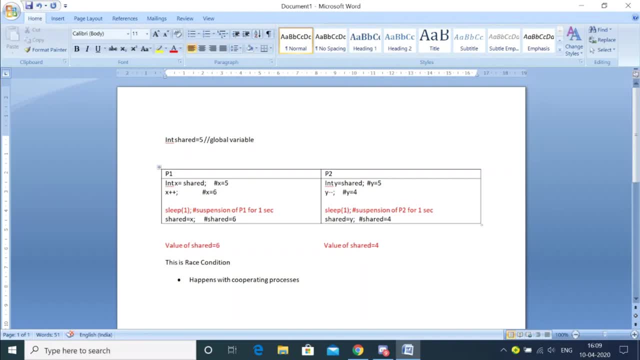 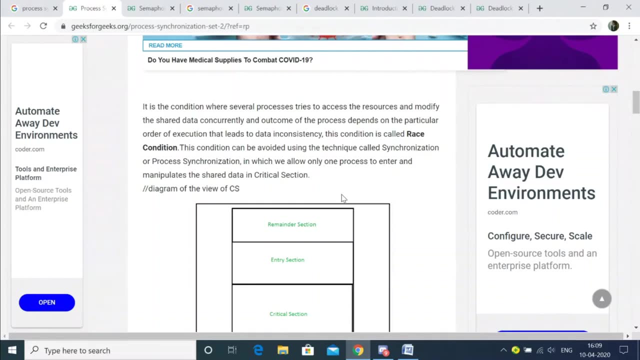 So to overcome that, basically we have process synchronization. Alright, Now, whenever, like, a code is being executed, Okay, So let's see. Okay, This is race condition. Okay Now, whenever we are, then certain things we are going to do. So let's. 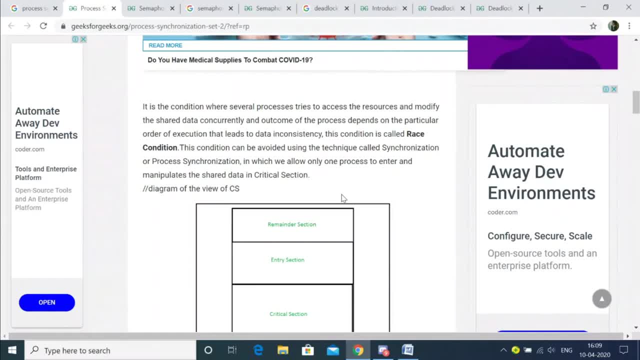 look at the next process. First of all, the documentation is the action resource, and the process and the outcome of the process depends on the particular order of execution. Here also, whatever value we got here- 6- and whatever value we got here for it was dependent upon the order. first it incremented, it went to a sleep mode, then 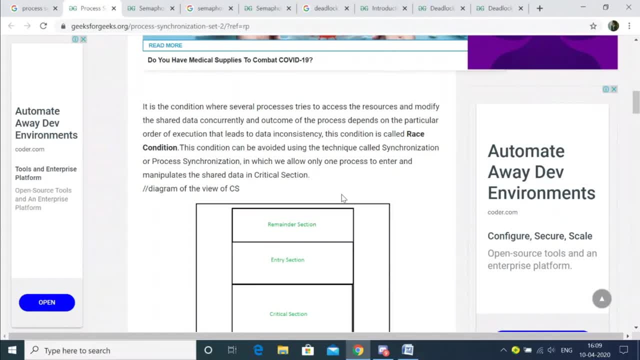 it came here, it was decremented. okay, so that order depends. suppose if sleep would have occurred at the, at the second line only, and this one would have been in the third line, then this value would have been different that time. so every code that we write in a program like in, especially in case 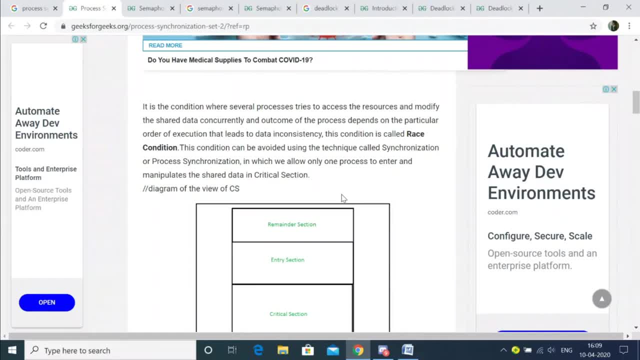 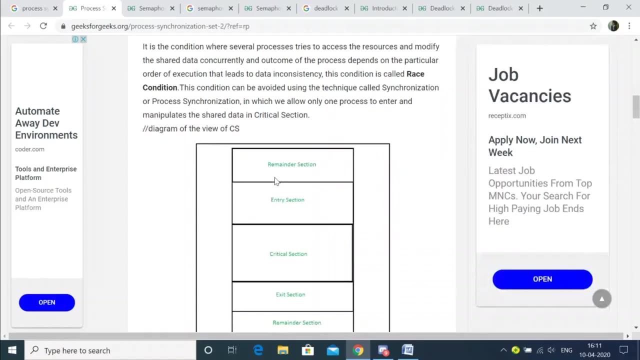 of cooperating process. the order of the code is very, very important, okay, otherwise it will lead to data inconsistency and this kind of situation. basically, we call it as a race condition. so this condition, as we said, we can avoid it by using process synchronization. so, in process synchronization, what do we do? we allow only one process, okay. so in process synchronization, what? 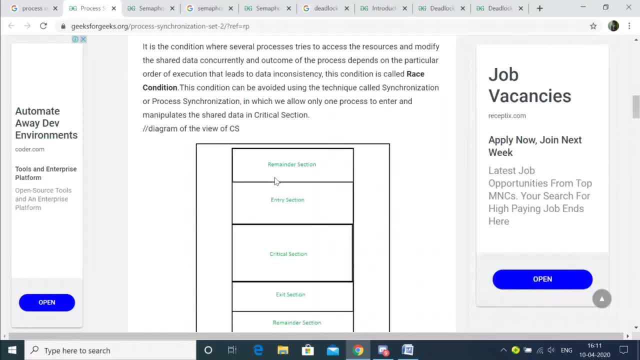 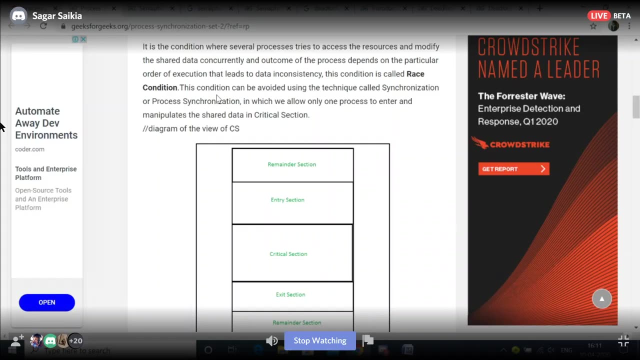 do we? do we allow only one process to enter and change that shared data in critical section? okay, so again i'm saying race synchronization condition. we already have seen that it leads to data inconsistency for shared variable or shared part of the coding. okay, so to overcome that, we have what process synchronization? so how do we? 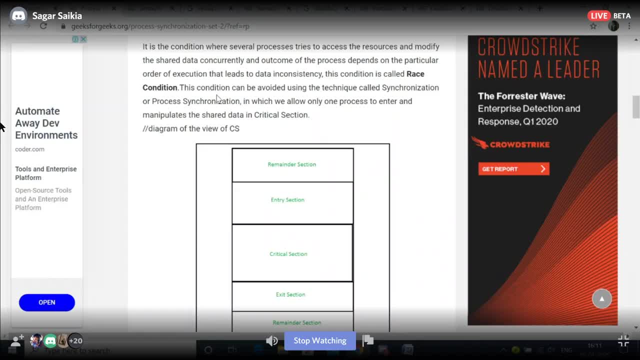 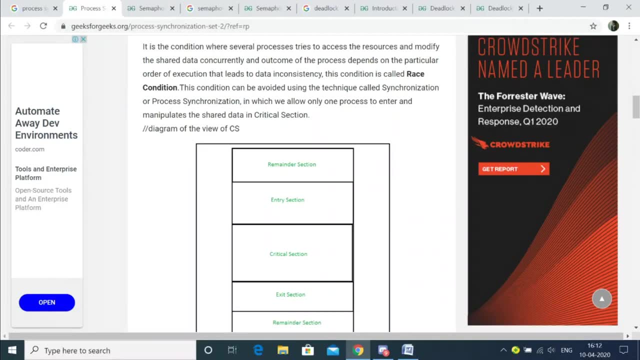 synchronize or arrange the processes okay, in execute while executing. what we do is, whenever the processes are executing, only one process is allowed to enter and update the shared part of the data inappropriate on state深 of code or positive code that we have already ordered on state of code. see because, also now, when we move in the code, we can runhall live services. 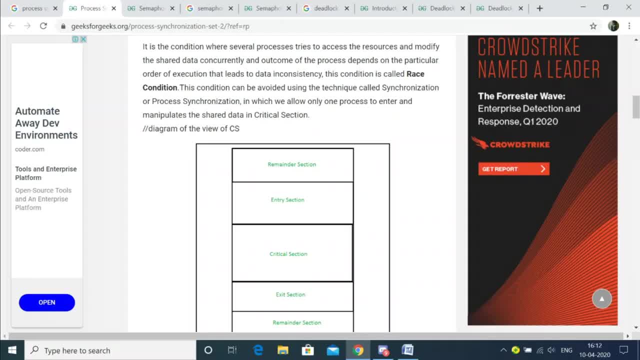 and also on state of code. see, because also now we can run stable of code only, not run aggot. we want not hand out but hand out, but achieve only the full desktop animation. if we want toソ, okay, in the other side, only one process right now. we've been talking about that, so it may lead to. 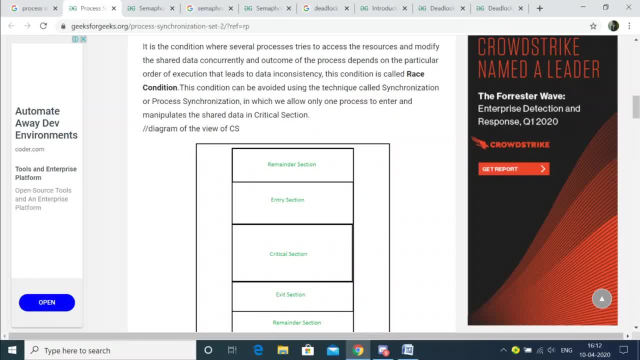 we actually have to suggest that, according to this, that state of code, even if we live in track, that is, we have to change. if we'm going to use sm最先 step, then we have to component to adapter this one part to this. one does not know which is the int and option one, and also 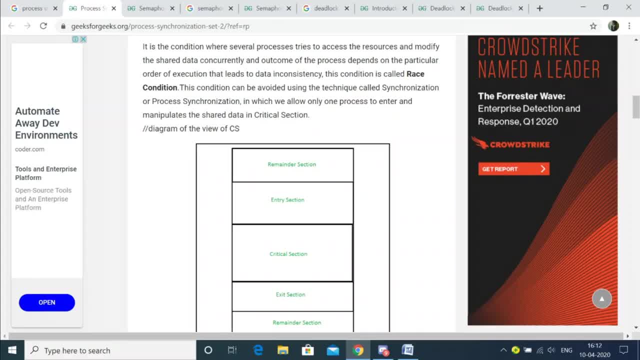 Floyd Weeks the yes take to use, which is part sets, okay, but but ideally actually up gets open. you are involved in some way. yes, whatever can happen, the program we'll act like a. that's not a problem. okay, but the only problem will arise only for the shared data. so if suppose 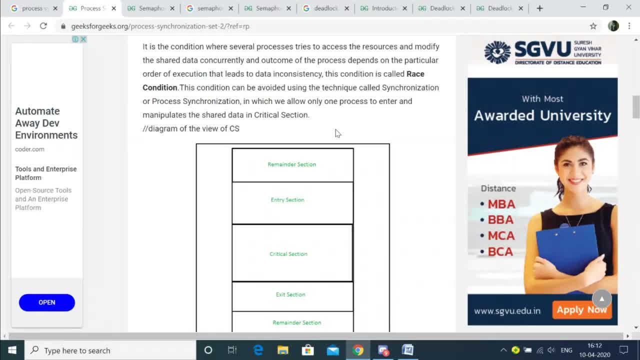 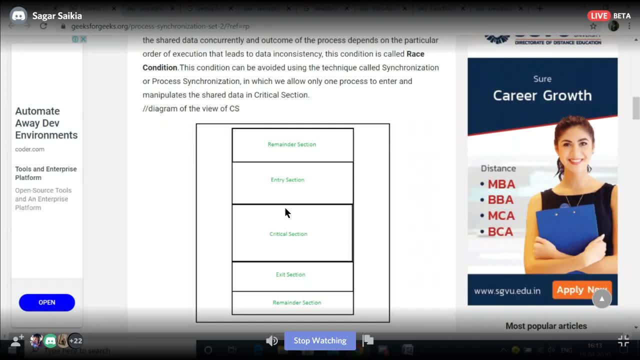 we have certain like this, then we will allow only one process out of all the processes. we will allow only one process to enter the data and change or update the data in the critical section. okay, so like for example here: uh, uh, we are having there how many uh? sections one, two, three, four. 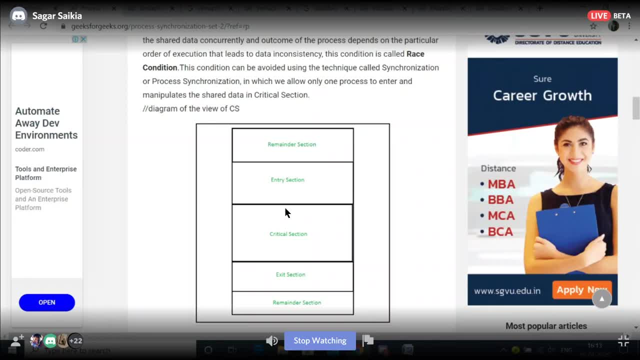 five and critical section is like the core. okay, so, uh, in critical section what happens is, uh, critical section, it's a part of the program where shared resources are accessed by various processes, so it is a place where shared variable resources are placed. okay, so in the critical section i can also say what they have written here. 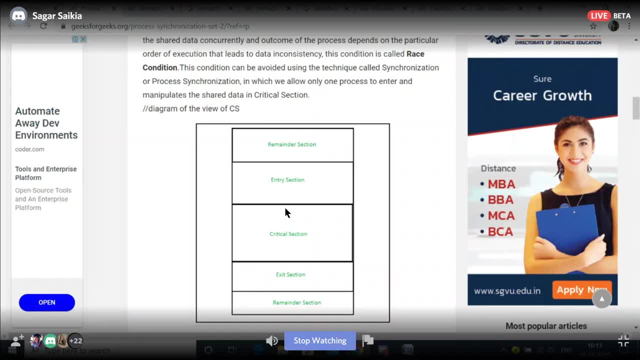 it is a part in which only one process is allowed to enter. that means in this critical section only one process can enter, like for example here: how many processes were there two? so out of the two process, if suppose someone has to enter into the critical section, then only one can enter in. 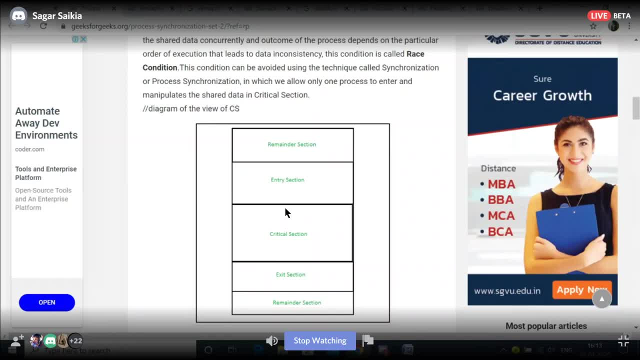 in one particular instant of time. okay, so it is a part in which only one process is allowed to enter and modify the shared variable. So here also we have seen there was shared variable. This was the shared variable, called shared only, okay, because it was shared. 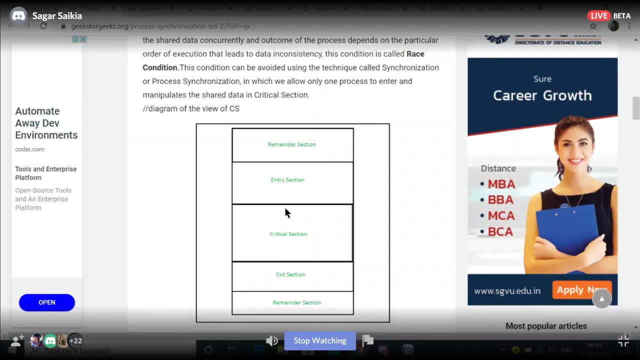 among the two processes, So only the shared variable, only one process allowed to enter and that process will be able to change or modify or update the shared variable. This part of the process ensures that only no other process can access the resource of the shared data. 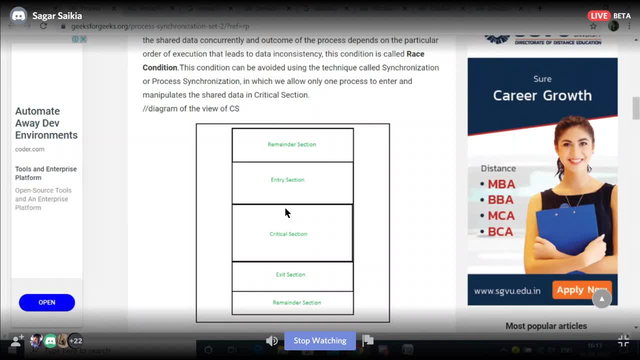 So until and unless the shared process is inside the critical section, so other processes will not be allowed to access that shared data at that period of time. It will be locked, something like that. Are you getting the point? Okay, But then how do we decide? Like there may be two, 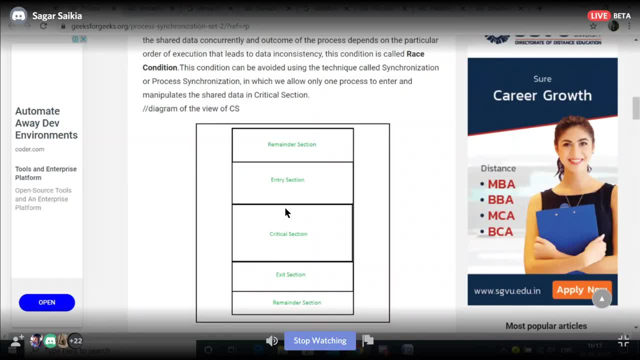 processes. there may be three processes. So how do we decide? So what we do is we may have in a program or, let's say for example, in a process, let's say for example in a code, like for example here: okay, there will be a section, like for: there will be a section. 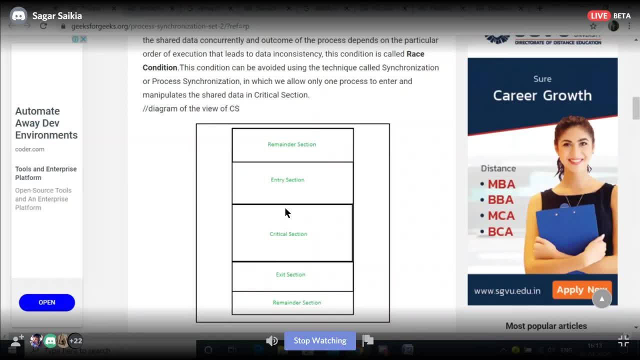 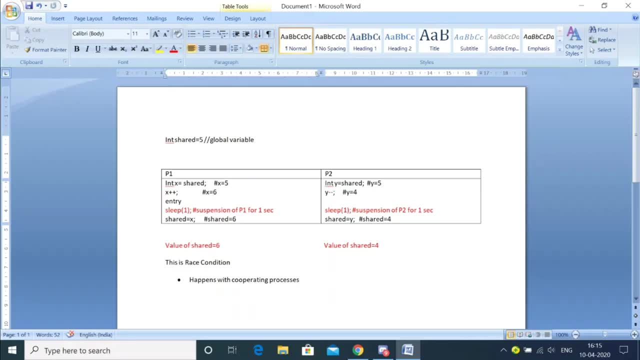 called entry. Let's say I'm just writing here. Let's say there is a function called entry. Okay, So what is the role of this entry function? Basically, it will tell the operating system like which it will basically hint, or it will prompt the operating system that once we reach that part. 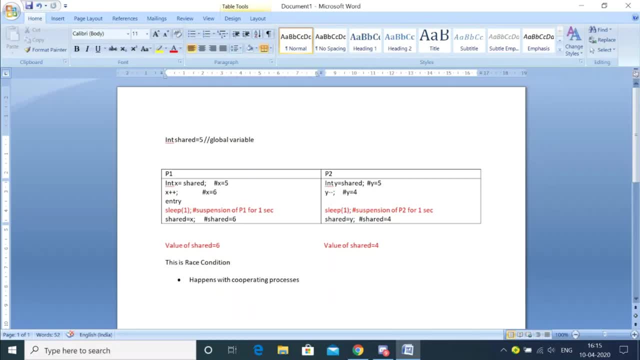 of the code, then the entry of a particular process in the critical section must be done out of many other processes, Like for example, here, let's say, the entries here: Okay, And suppose I got, let's say, the entry segment: Okay, Entry is also a piece of code, So I'm just showing. 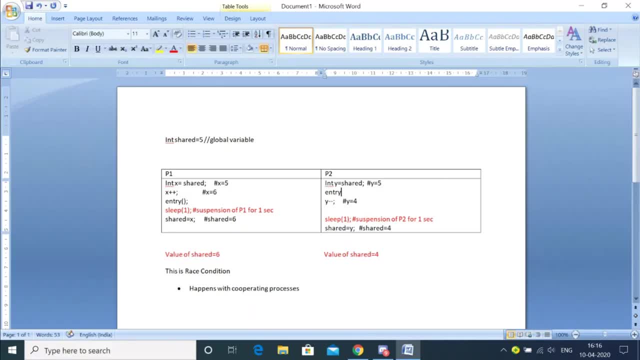 oh, sorry, Oh, I'm just showing what is the default code And I want to say: give me a text. I want to say, oh, I want to be in the code that I wrote. I want to be in the code that I'm. 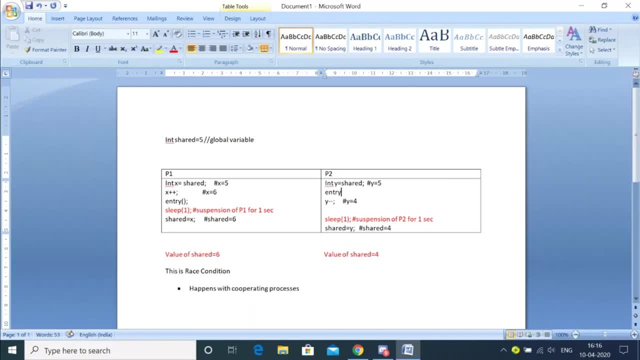 assigned. So what I'm going to do here is I'm just going to put this there. So let's say, here I'm going to say, okay, so this button, this is the code, this is the input loop that I wrote. 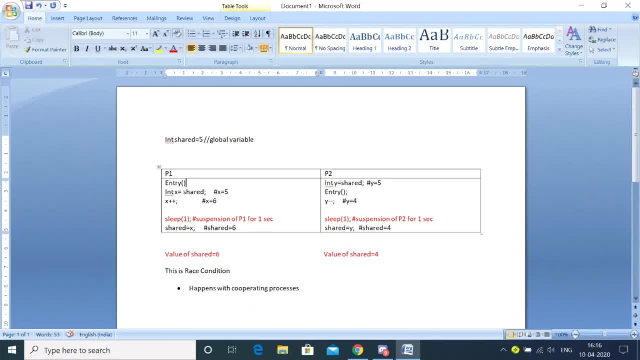 Okay, signal the operating system that the process has to be fed into the critical section. So once suppose, P1 is scanned. so what is it seen? Oh, it is seen that there is an entry function, or maybe an entry code is written. 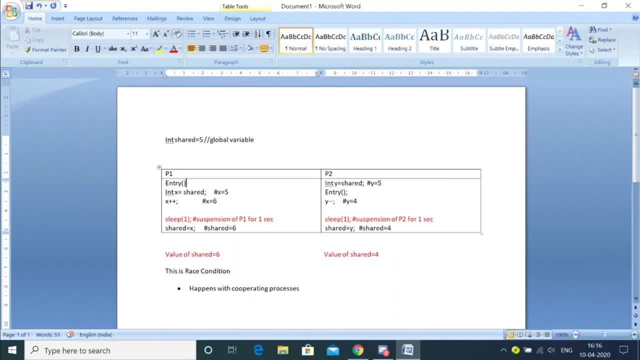 So the moment this is seen as a part of the instruction, it will be prompting the operating system that the process has to be. I mean to say the shared part of the process. the shared part of the process must be taken. okay to the critical section. 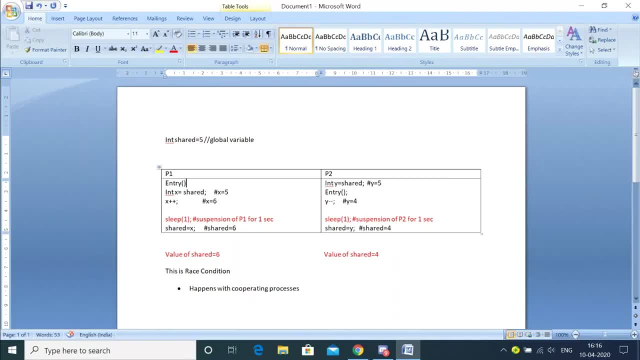 So that's why it is saying entry section. it is the part of the process, only, okay, which decide. That means it is a part of the process, means what It is: a code will be there for the entry section which will decide the entry of that process. 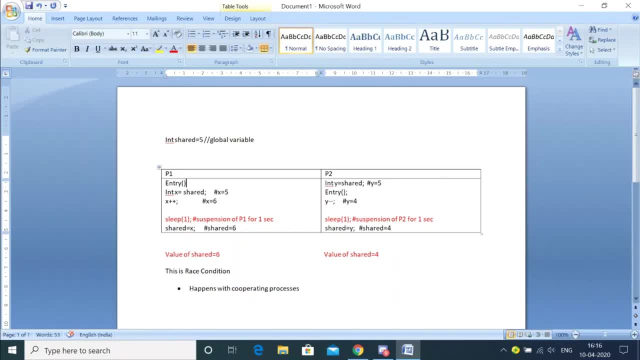 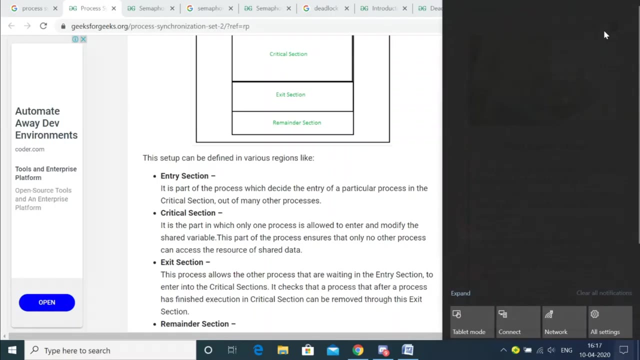 in the critical section out of many other processes. Okay, so once you have prompted in the code that I have reached the entry section, so automatically that process will be loaded in the critical section and will be executed. Okay so how long will it execute? 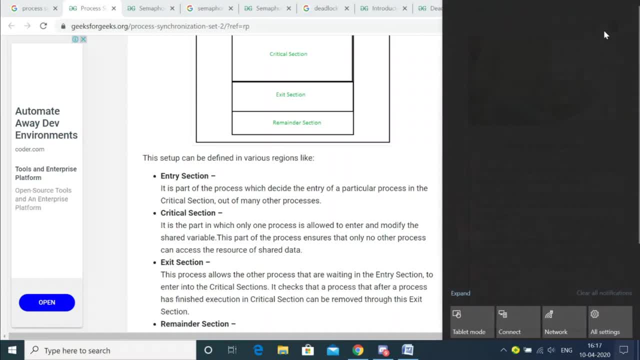 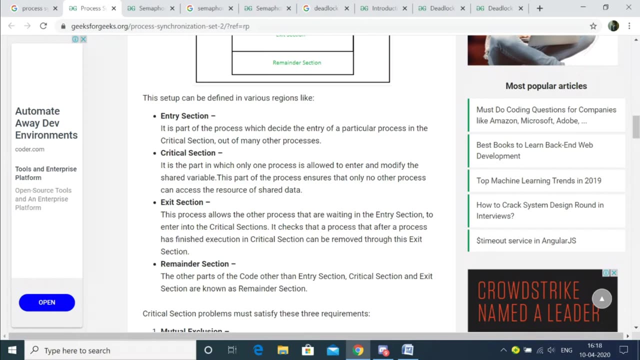 That is the question. okay, Once it is in the critical section, how long will it load? That is also a question. So it will be continuing until and unless it does not reach the exit section. That means once the shared part of the variable is accessed, manipulated. 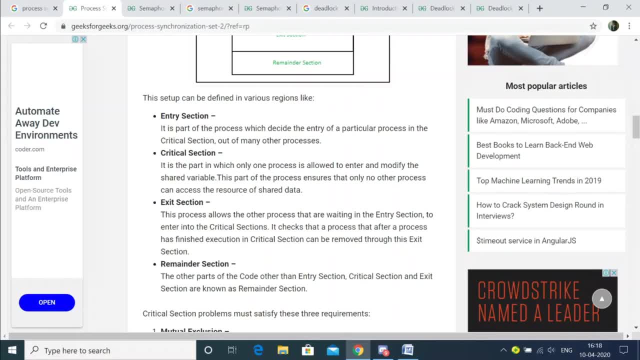 okay and updated. then after that there will be a code in the program only which will basically again prompt the operating system that it needs to come out. That means that process has to be released from the critical section. Okay, so once that exit section is encountered by the OS, 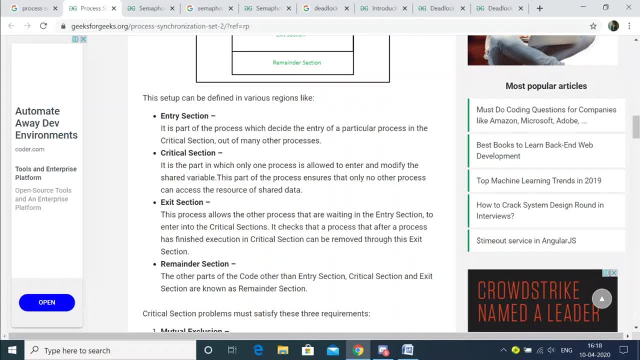 so that process is released from the critical section, making way for other processes. So once it is done it's work from critical section. it will come here into the exit section. That means it has finished the shared part of the program. 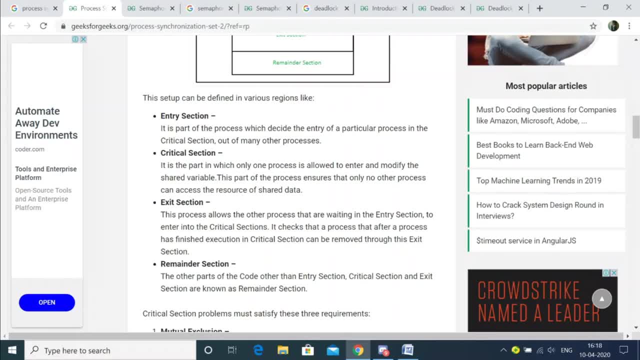 Now there will be a code in the program only which will say that okay, I have reached the end so I should be exiting. So once that process exits from there, there will be a remaining section. So what will the remaining section do? 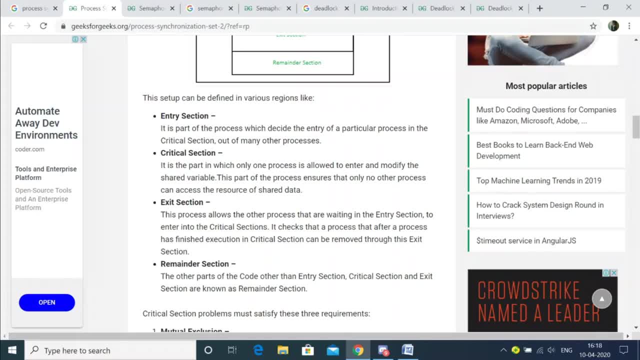 So it will keep that code out of the process, So it will not be needed to work. So what will it do? First of all, it will not be needed to work. So what we have is, first of all, it's a process. 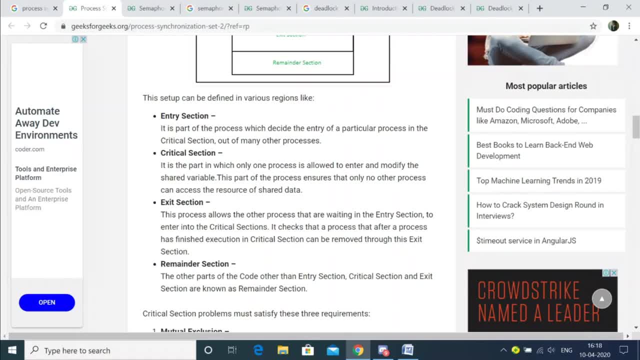 So then it's a co-operative process. In the process, you don't have to worry because the process is not affected by the other process. Okay, it's execution In co-operative process. there is sharing of resources, There is sharing of various devices. 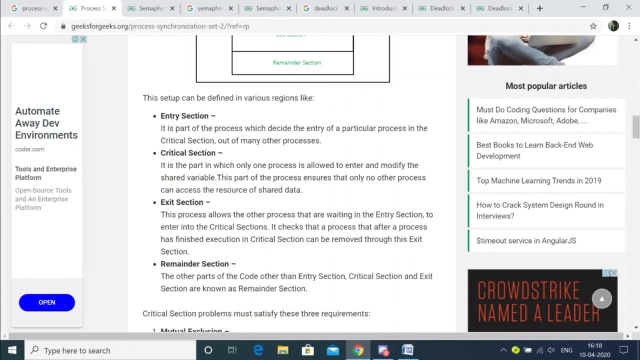 So in this case there is a need to have consistent data. So we see that we should not give the values of the code here Because it's in code here, but we should go there because there is no agreement on it. 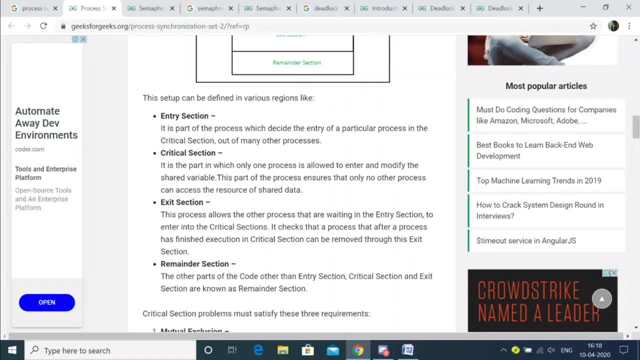 We should not decide right, Because vote will be racing, vote will be competing for proving themselves that they are right. Okay, so some of the operating systems may give us value six. Some of the operating systems may give us value seven. 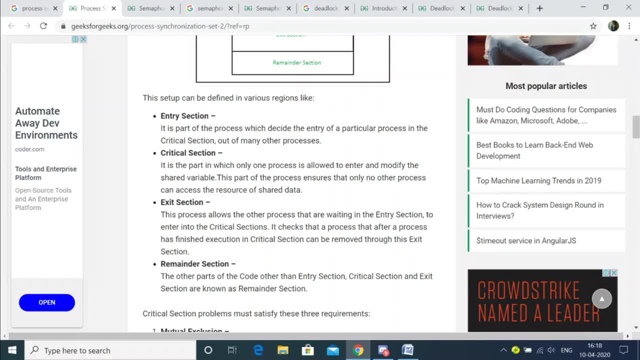 Okay. so some of the operating systems may give us value six. Some of the operating systems may give us value four. So in this situation, when both- the final output- is racing to prove themselves that they are correct, So we say that this is a race condition. 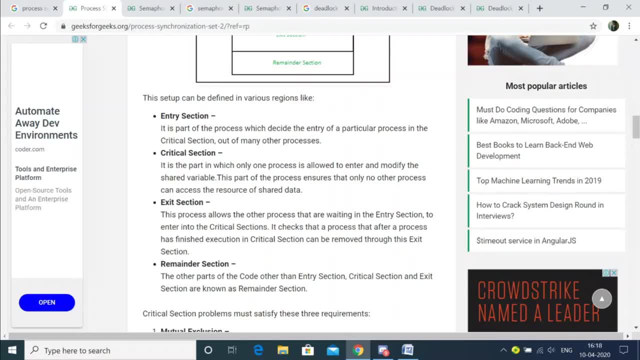 Okay, so it's, which is not good, because there is an inconsistency in data: Correct output was not produced. Then what do we do Then? in that case, we have to look for certain solutions. Okay, and this happens basically with co-operating processes only. 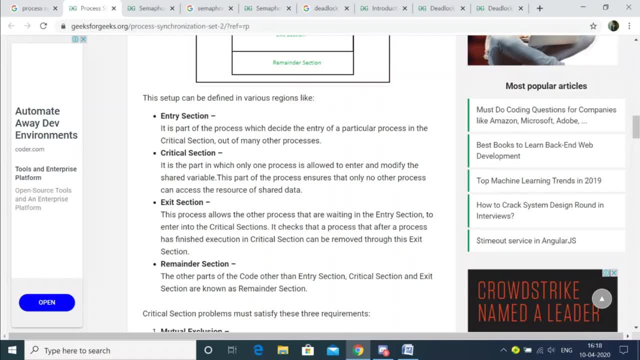 So to solve this we will use a concept: criticalization. Okay, there's such a one process to enter and fight the saying between Two processes. This is how one process enter: Okay, now you see that. See, you have to create a special data set. 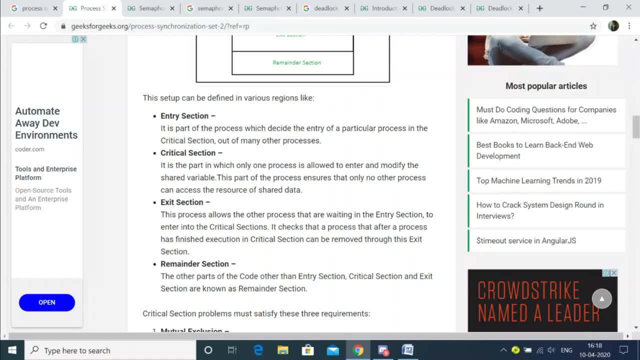 Now you have to create a set of essemi, So let's train the data. What you need to do is, first of all, to define a dominating function. How do we change the size of the GLORIA trusting Table? Is that like a very secure tele Saskatchewan say through, not Passست. 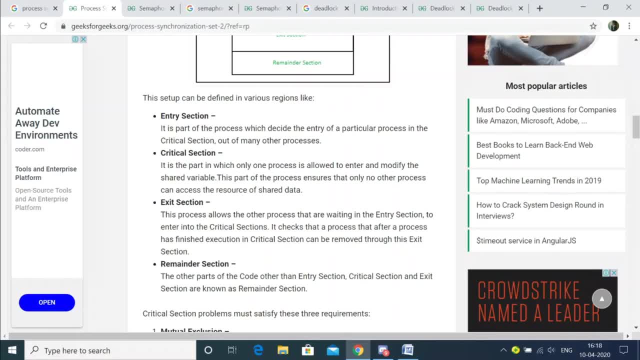 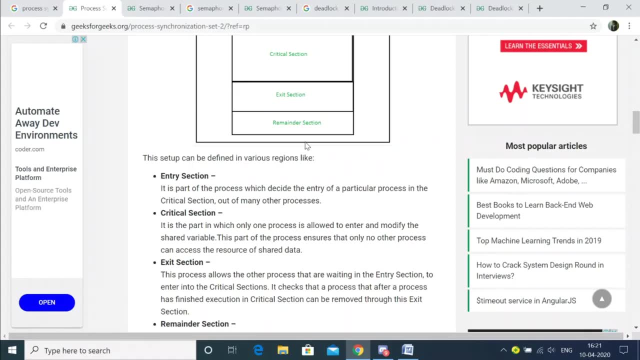 Is that like a very secure Palestinians Say, operation or manipulation? the shared data is done, then it can exit from that critical section and other processes can request. okay, now how this takes place: the request and the exit. okay. so what happens? in the c code only or in whatever language code you have written? 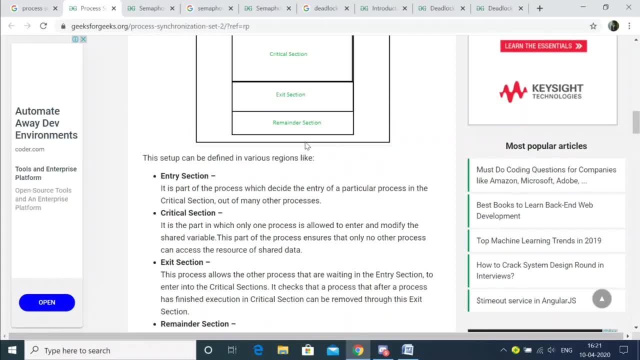 that code will be divided into various sections. one section is where we are writing the shared variable. that means the part of the c code where uh two, three processes are accessing that variable. then certain parts of the code will be there which has got non-shared portion. that means 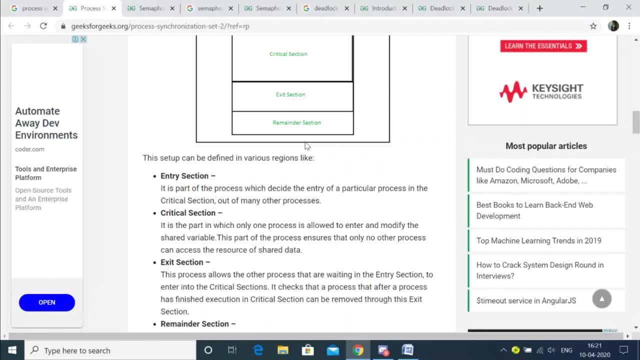 local variables only are there where it is non-shared. it is not shared between the other processes, so that doesn't matter, it will keep on executing. uh, you can say parallelly, because there is no dependency, so there is no problem. so one suppose we have reached a part of the 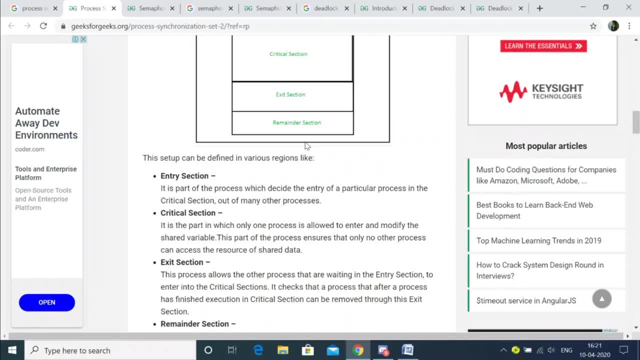 shared variable. it is not shared. it is not shared. So before that, only there should be a code which will tell the operating system that this process is basically ready to be put into the critical section problem. okay, So there will be a code in the entry section, okay. 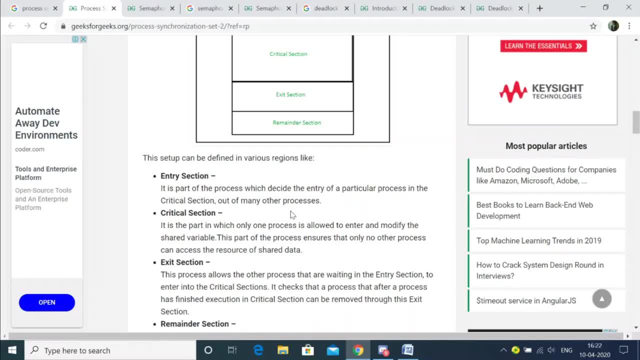 So there will be a code in the program only, which is called as the entry section The moment that code is scanned. okay, So it will be notified to the OS that now this process has to be put into the critical section If a situation comes like, for example, two of them are saying process P1 also versus P2 also. 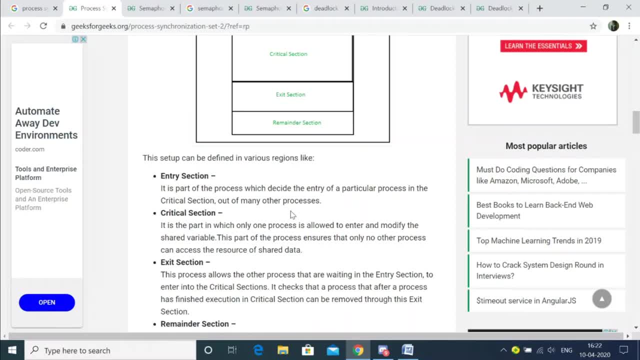 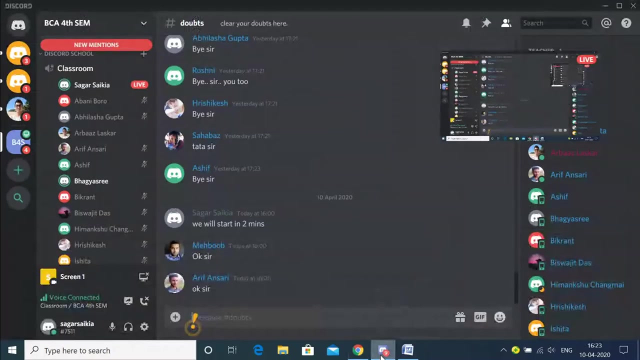 is it possible that both of them can be saying at the same time this one should be taken? Is it possible that both of them will be requesting that this entry section it has both of them has encountered. can that be possible? Can that be possible that both are requesting that it should be put in the critical section? 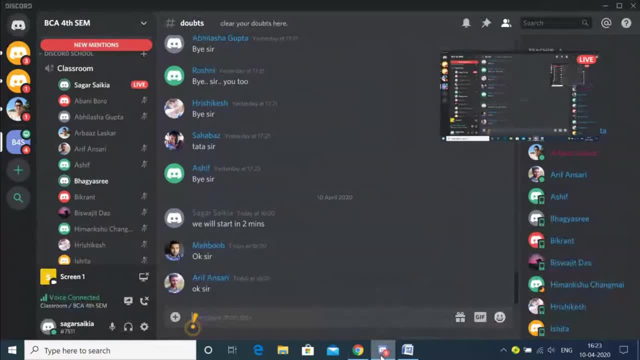 Can it be possible in case of any processor is running? It's not possible. It's not possible, Okay. Okay. So in one time, only one process only can be allocated to the critical section. okay, So that's why, according who is making the entry section request. 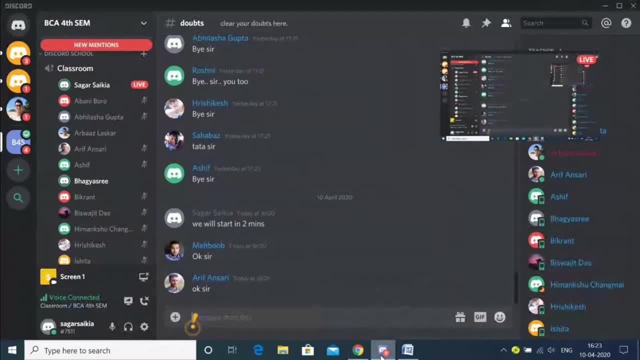 Based on that only, we are keeping the process into the critical section, So it will be executing, manipulating that data Once the data has been manipulated, updated. so what will it be doing? The next line of instruction is the exit section of the process. 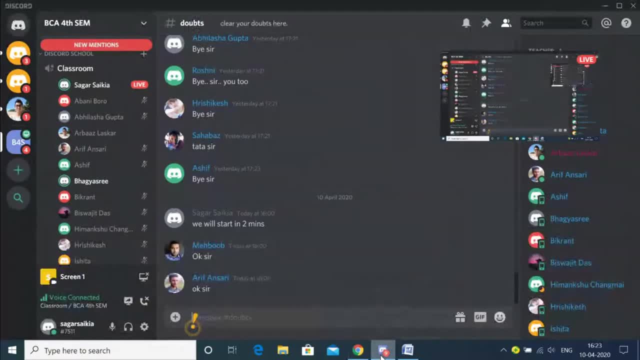 So that exit section will basically tell the OS that the process execution is done. That can be removed from the critical section. okay, So in remainder section, what will be there? The program is divided into three parts: entry section, critical section and exit section. 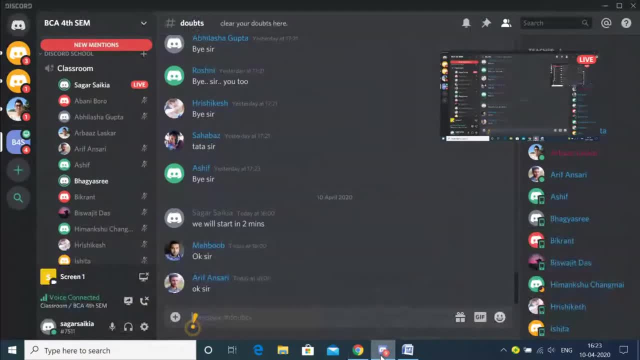 Entry section also, we have to write certain coding. Critical section also, we have to write certain coding. Exit section also, we have to write certain coding Leaving all this. whatever other parts of the program are remaining, that is the remainder section. 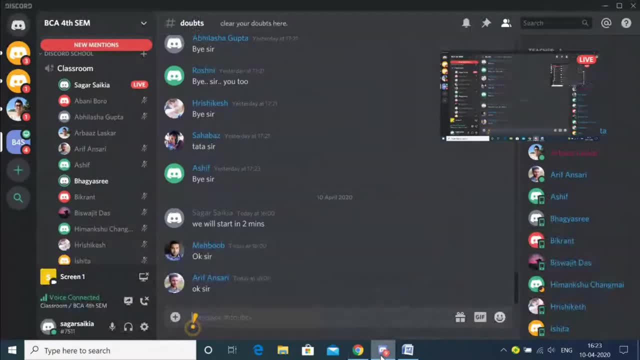 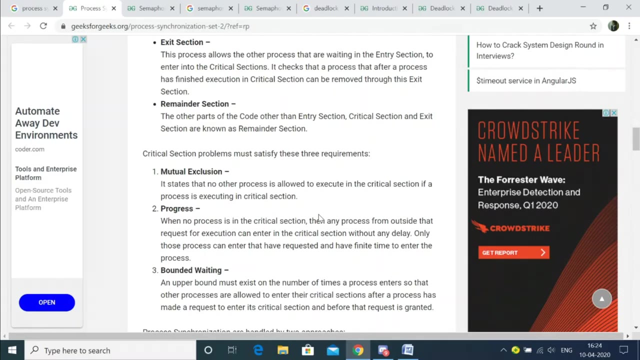 So the next line of instruction is the exit section of a program. That means one program has been subdivided into four different regions. Are you getting okay? Then certain factors that critical section must be satisfying okay. So first is mutual exclusion. 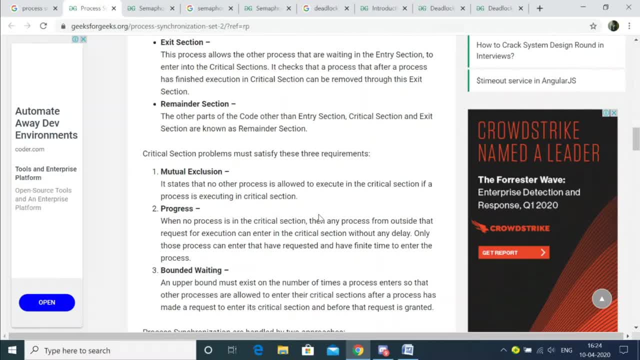 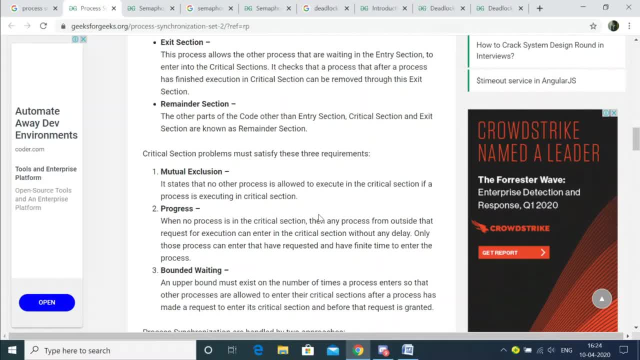 A process to execute in the critical section. if suppose some other process is already present there and it's being executed okay. So that's called mutual exclusion. That means, one process if it's already there in the critical section, then other processes has to wait until and unless that process is not. 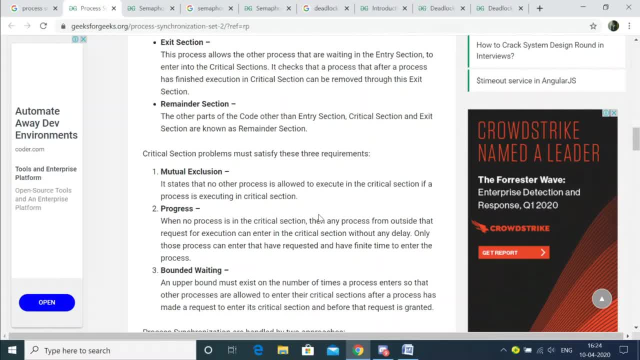 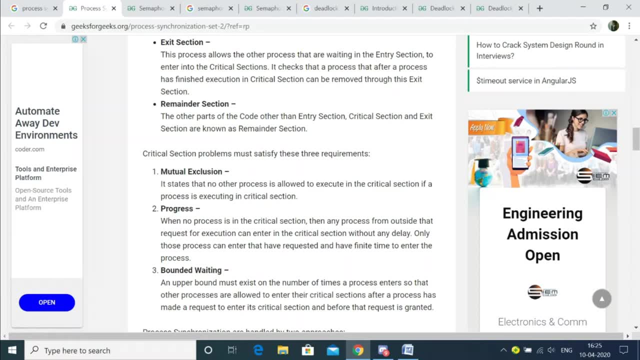 you're done and it's not yet, has not yet come out from the critical section. So that condition basically, is sort of your mutual exclusion, So that Всё is mutual exclusion. it's a progress, okay. so what does it say is when no process is in the critical section? 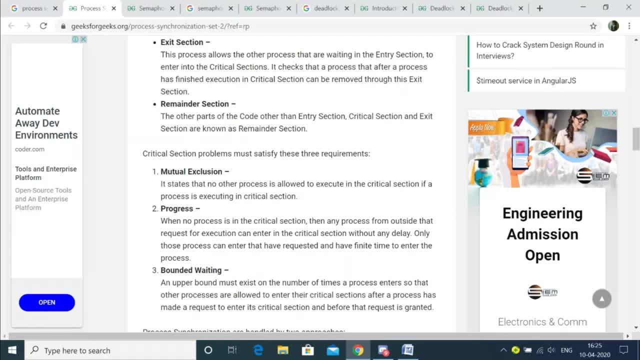 then when no process- that means no processes- are there, then any process from outside that request for execution can enter in the critical section without any delay. so suppose if there is no process at all in the critical section region, then it's fine, then whoever process will make. 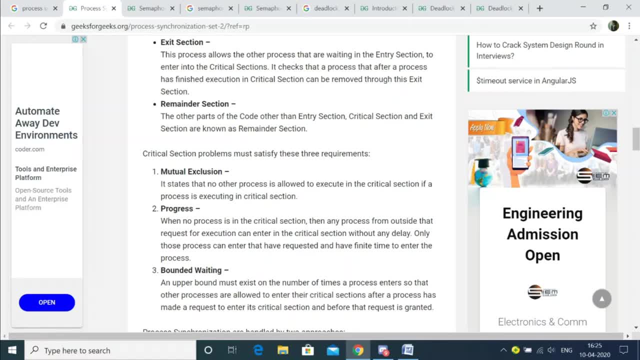 the first request, that process will be given the priority and can enter into the critical section. only those process can enter that have requested. that is clear and a finite time to enter the process. okay, so it's not that the process should take a very long execution period of time. 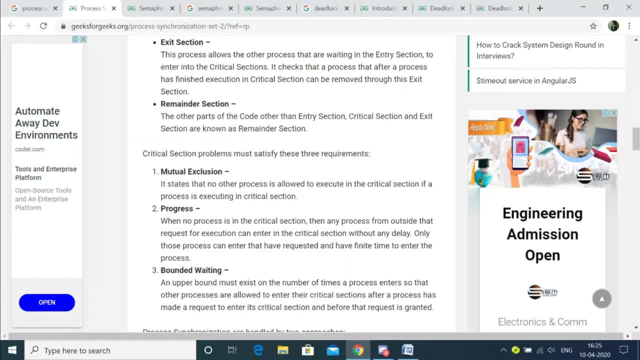 so that should be avoided, okay. so anyone who makes the first request and whose best time is the first time of the process, then it's fine. then whoever process will make the first request is pretty much reasonable. so accordingly, that process can be allowed to enter into the critical. 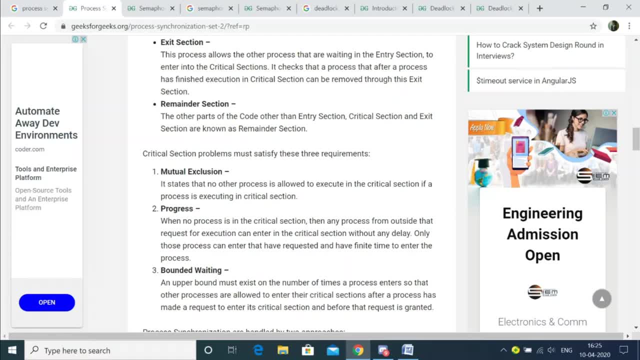 section. okay, so these are the conditions that critical section problems must satisfy. then another one is bounded waiting. so what happens is bounded waiting. an upper bound must exit exist on the number of times a process enters so that other processes are allowed to enter the critical sections after process is made a request to enter its critical section and before that request is. 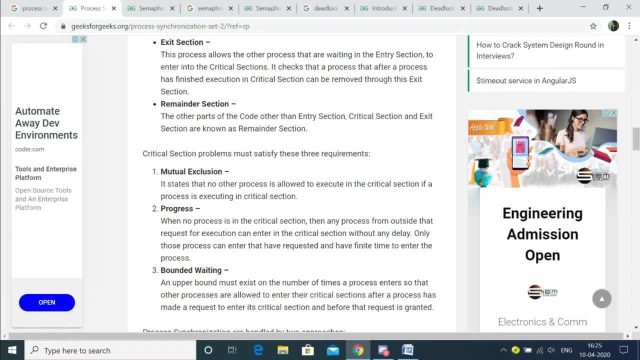 granted. okay, let us say, for example, we have to processes P 1 & P 2. okay, now let's say P 1 has entered into the critical section, it has executed and it has exited from the critical section region. now, who should have got the chance to enter the critical section? P to that, what has happened again? 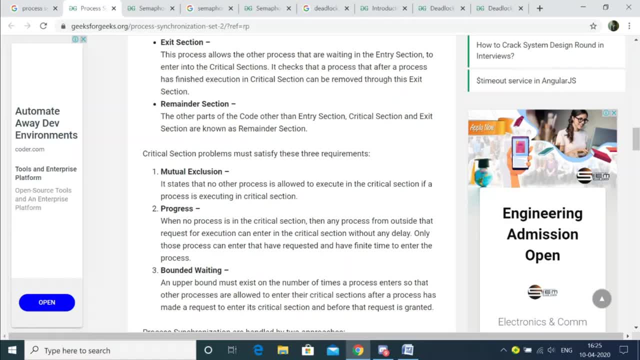 P 1 has entered, it has executed and the critical section region has gotten the critical section of critical section P 2. x which parallel as well, x which parallel Armenian, yani along the this new normal. but it is unable touate the total ponto at which another process enters into thewang tabio. 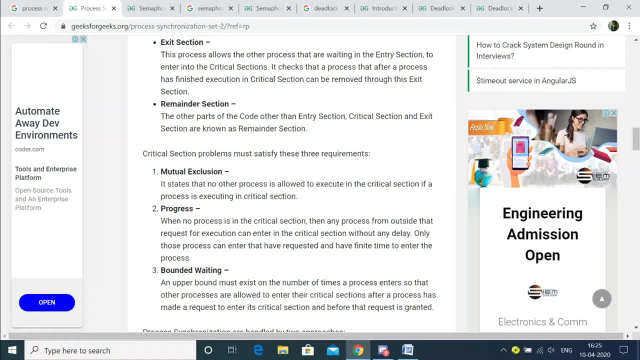 region and then it has exited Third time. also, only P1 is only getting the opportunity for entering execution and exiting. P2 has to wait For how long? it has to wait For an infinite number of times. So this kind of you can say anomalies should be avoided. 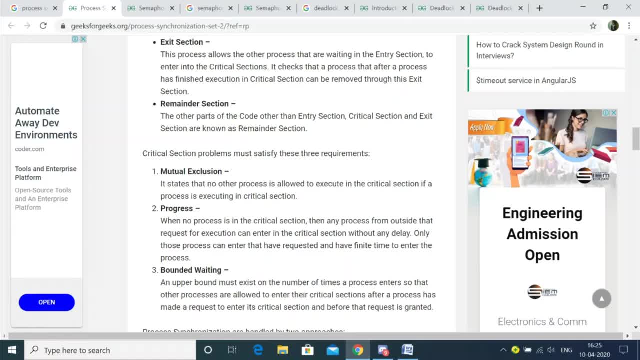 and while designing the critical section, coding, the programmer has to make sure that such kind of- you can say- improper distribution of execution of processes must be avoided. Okay, so that's why this is called bounded wait. That means a process can wait, but for 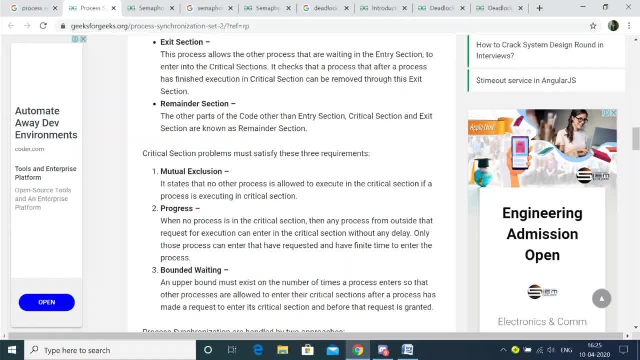 a finite number of times. It may also happen that P1 is given, It's okay. first, second, three times, three, three times it is given to execute. then fourth time P2 is given, then again six, then again five, six, seven, three times P1 executes, and then again for. 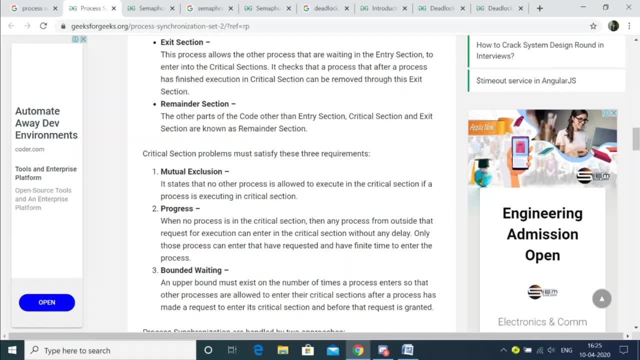 one time P2 executes. So finite time is okay. Three times P1, one time P2.. Three times P1, one- That way it's okay. Two times P1, one time- That way it's okay. But if it is wait for 20 units of time, 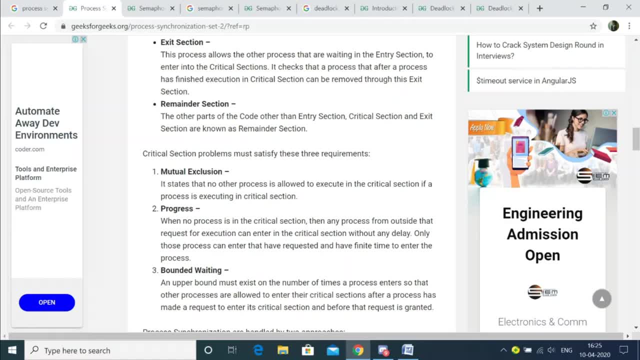 or if it has to wait for more, larger than that, infinite number of times, a hundred number of times, then only P2 will get the scope to execute, to enter. So this kind of problems should be handled by the programmer while writing the code, so that you can say: 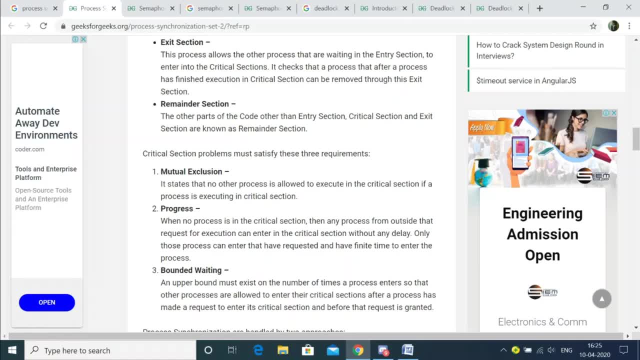 process synchronization can be Obtained. Okay, So any problem, you can write in the comment section Algorithms. I'll be discussing like separately all of them, because there are too plenty. So that's why I'll be discussing like in different class altogether, because I have 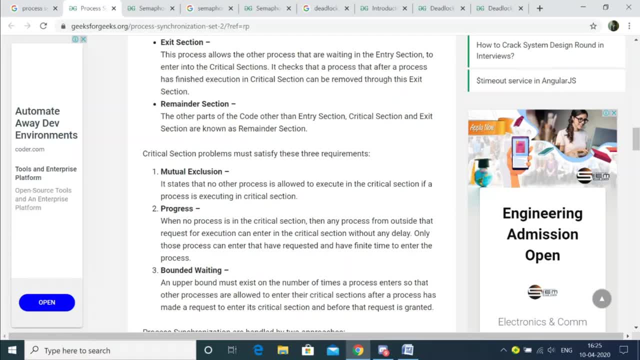 to make Like examples also in Word, MS Word. okay, So can I proceed towards the next topic? Okay, So next topic that we have is your semaphores. okay, So let us see the brief history first. 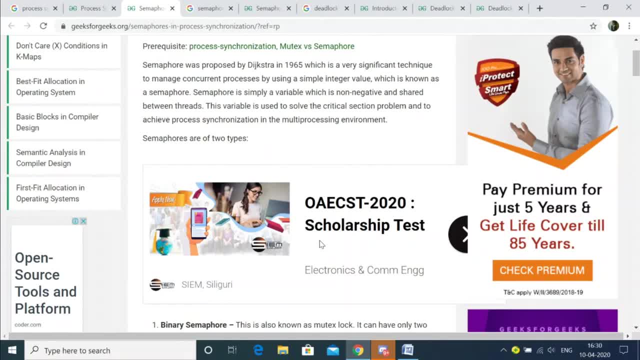 So semaphore was proposed by. So semaphore is just a value basically used to indicate that whether a particular region of the code is like ready for execution in the critical section, or whether it's not yet ready. Okay, So it is basically used in a multi-processing environment. 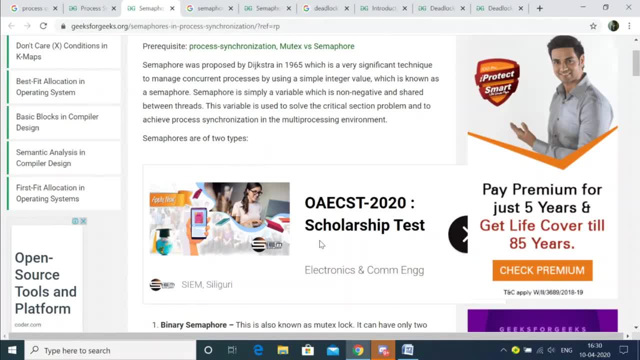 Now semaphores, as we said that it is an integer variable element, isn't it? It is non-negative, That means its value can never be negative. okay, It is used for mutual exclusive process. That means if one process is running, the other one should not be executing. okay. 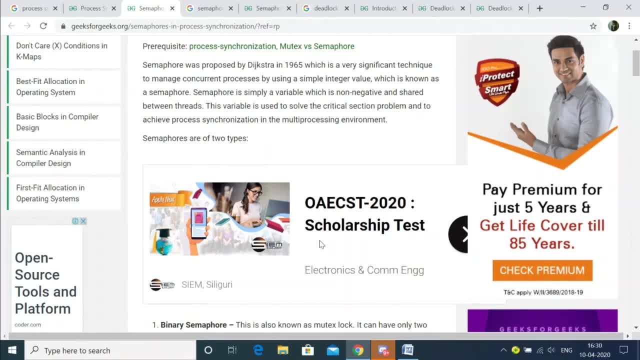 Used by only a cooperative processor. So, as per the theory, there are two types of semaphore. One is the binary semaphore, okay, And the other one is the counting semaphore. So binary semaphore, from the name itself it will have only. 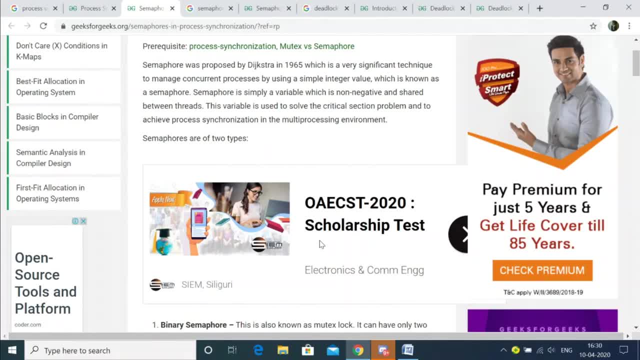 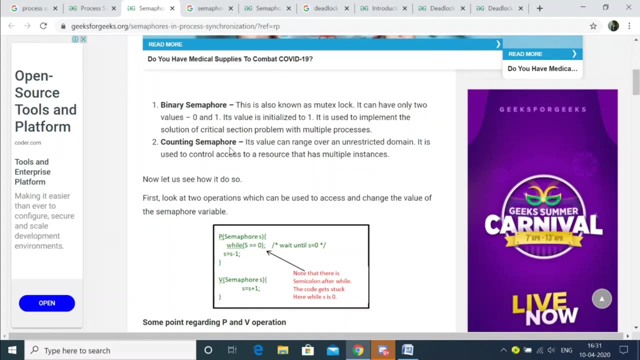 Its value is always initialized at the beginning to be one: okay, And this is basically used to implement the solution of critical section problem. if we have multiple processes, Okay. Counting semaphore: yes, Tell me. Sir Nihal has asked a question in doubts. 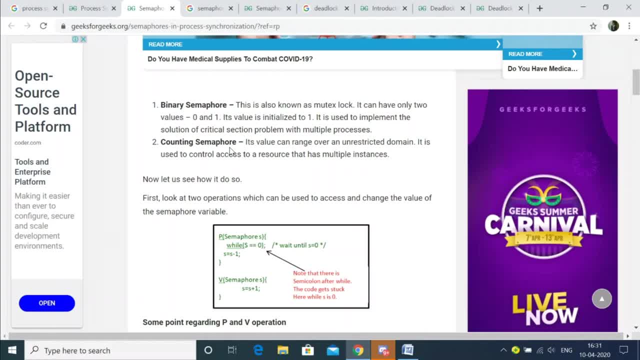 Okay, Let me check. Okay, Bounded again: no, All right, Okay, So when we talk about bounded weighting, okay, So suppose, for example, as I said, let's say we have two processes, P1 and P2.. 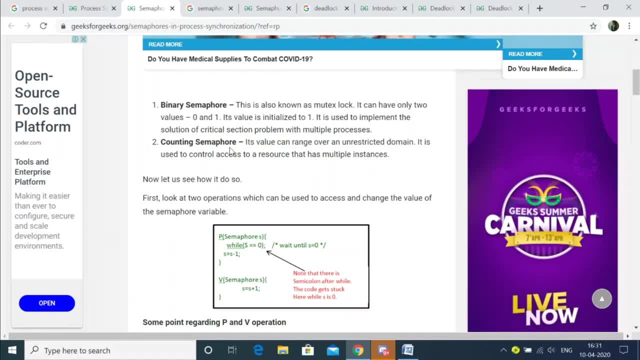 Okay. Now let's say, for example, if P1 has entered into the critical section, it has executed, He has done its work, It has come out okay. So P1 has done So. who should be given the priority next? 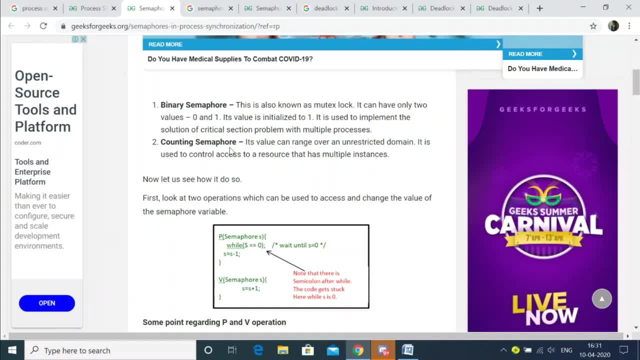 Should be given P2, okay, But what has happened? next time Again, P1 has entered into the critical section, It has executed its code and then it has come out. So third time also, fourth time also, it has been doing and this kind of repetition. 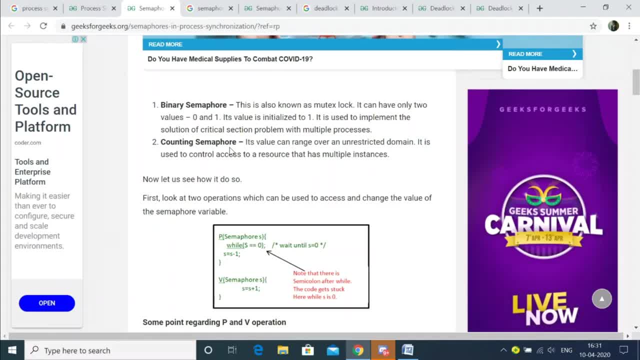 has taken place. Well, let's say, for example, if P1 has entered into the critical section, it has done its work- let's say 20 number of times, or 30 number of times- and it kept P2 waiting. 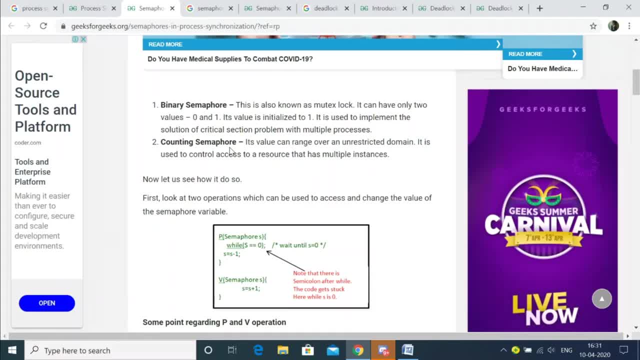 But this should not have happened, because whenever a particular process has to execute a critical section, maybe we can give him a second chance or maybe at most three chances, okay, But the other processes also should be given a fair amount of scope to enter into the critical. 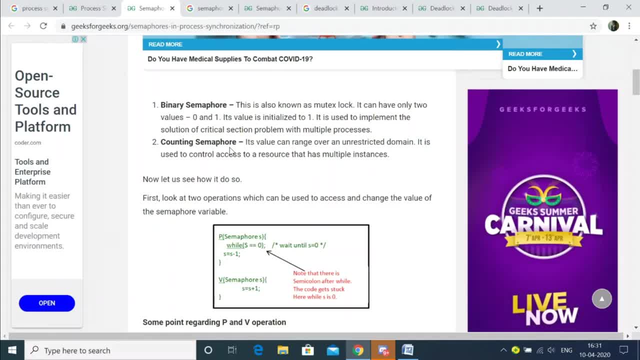 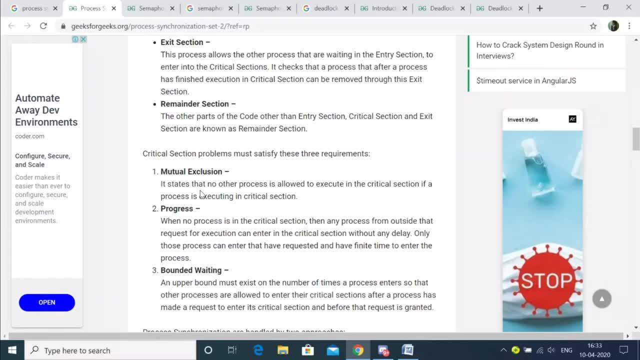 section and perform its work. But what has happened here is P1 has always, like, taken the opportunity And it is making use of the critical section. okay, So keeping P2 waiting, So this kind of like problem. basically we handle it using bounded waiting. 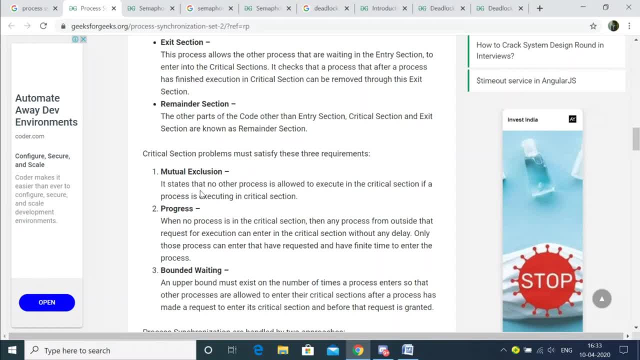 That means, okay, P2 can wait, but there will be a specific amount of time. Let's say, for example, P2 can wait, let's say, if P1 has executed for two times or three times, but there will be a limit. 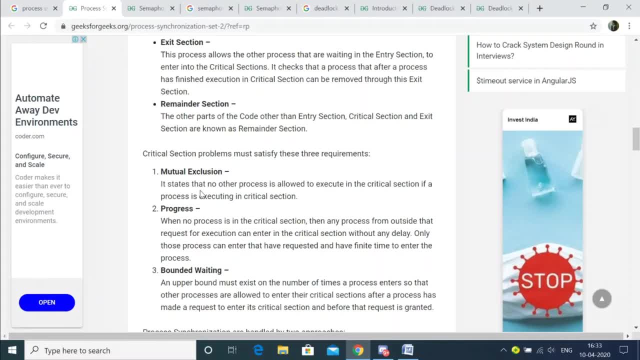 That's why it's called bound limit-based. okay. So let's say we can give permission that P1 can execute At most for three times. So after three you can say three times of usage of critical section by P1, then P2 will. 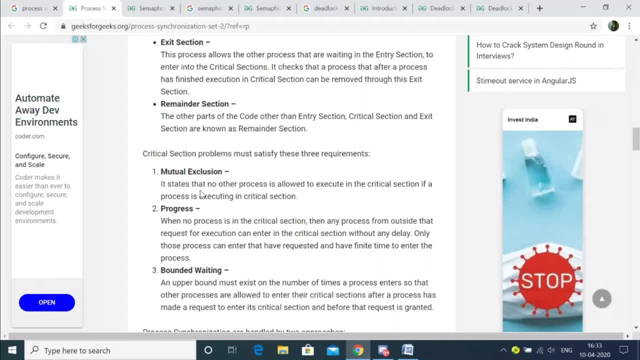 be given the scope Again next time three times. P1 will be using P2 that way, But it will not be that P2 has to keep waiting till when P1 will release the system. So it's not like that okay. 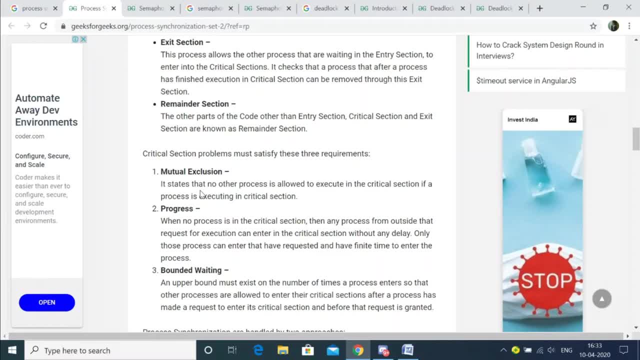 So this kind of- you can say- tackling of range, that how much one process can execute, okay, the critical section of a region, This is called your bounded waiting. So does it clear? Okay, so I'll just give this link: 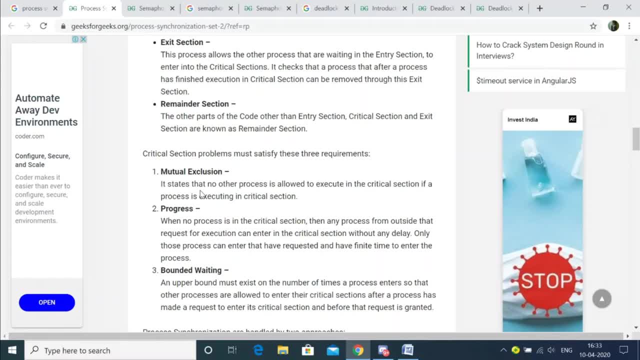 Okay, so I'll just give this link. So this will basically give you process synchronization and critical section. okay, Then next comes is the semaphore. So what is the semaphore? We have already seen it was proposed by Digixtra in 1965.. 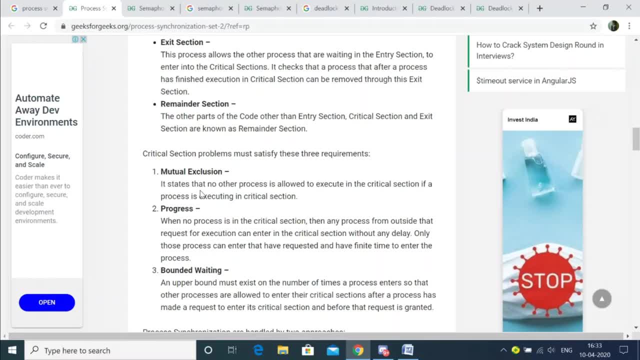 It's a method to manage processes which are running concurrently. It's a method to manage processes which are running concurrently by using a semaphore. It's a method to manage processes which are running concurrently by using a small integer value. The values are always non-negative and they can be shared between threads as well. okay, 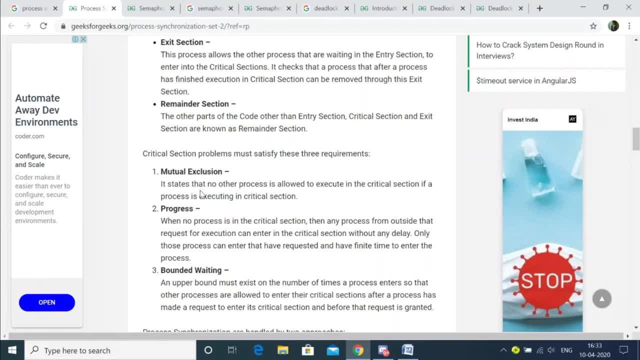 It is basically used to solve critical section problem. okay, So as we say that there are two kinds types of semaphore- binary and counting- So in binary, the value of these semaphores is zeros and ones only. okay. 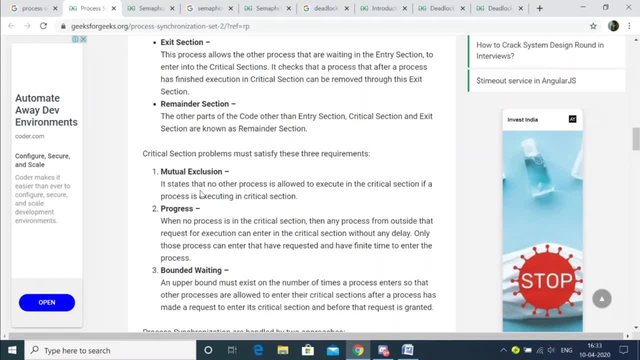 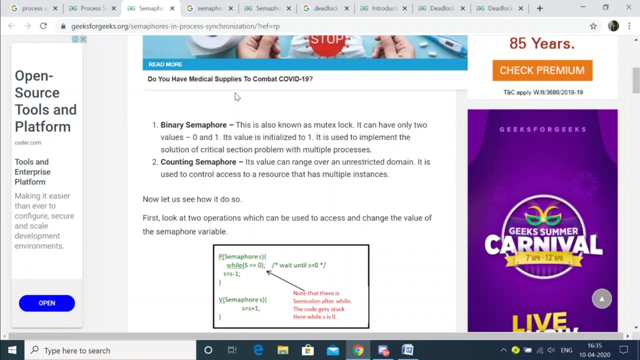 And its initial value is said to be one. okay. It is said to implement solution of critical section problem with multiplicity, So we will see how does it work? And another kind is counting semaphores, so its value can range over an unlimited domain, okay. 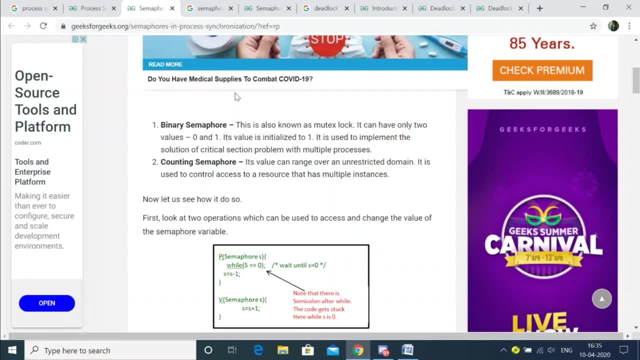 It's not a zero and one. it can be 999,, it can be three, it can be four, depending upon how many processes we have. So depending upon the number of processes that we have. so the value of the semaphore is kept, okay. 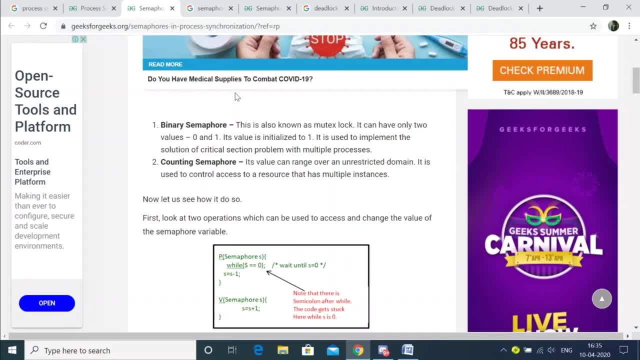 So it is used to control access to a resource that has multiple instances. So what does it mean? We may have one resource That, let's say, four resources- sorry, four processes- are trying to access. Here instance means process. 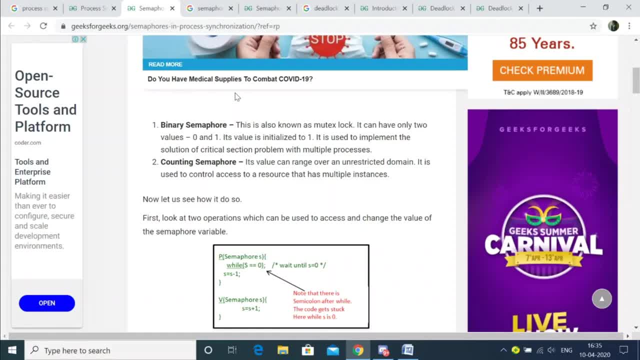 So that's what the meaning is. It is used to control access to a resource. So one resource can be available to one process only at one point of time. So if there are four processes which are trying to access the same resource, so here the semaphore value will be four. okay, 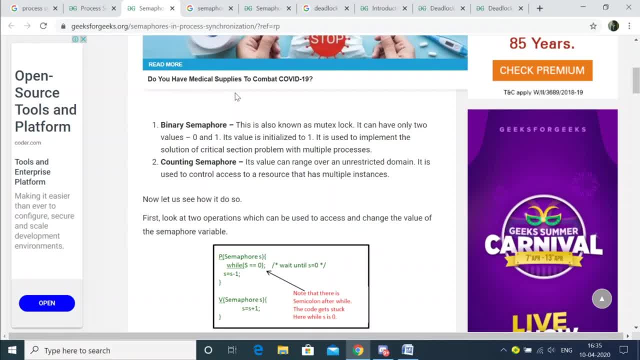 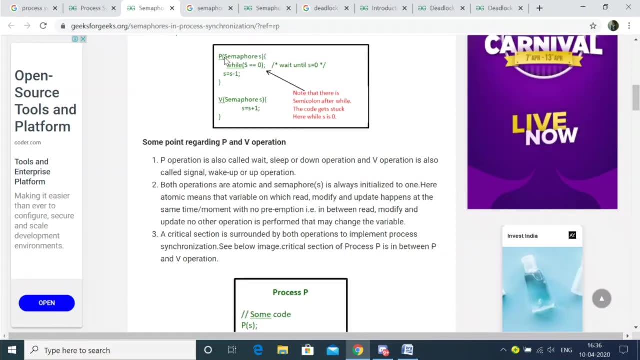 So let's say, for example, we are having here this process. So let's say we are having a piece of this code. So if you look here there are two sections. One is P, So P is basically the wait function, I can say the wait part of the program. 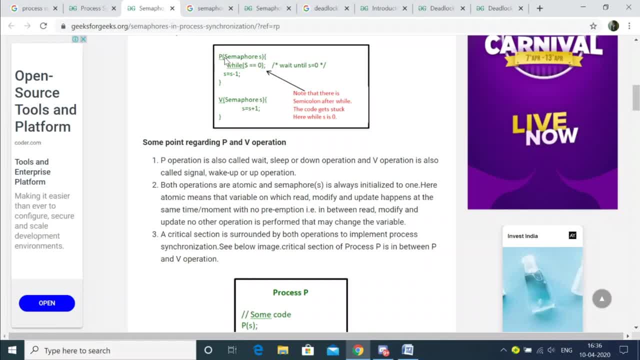 V is basically the signal, okay, So there are two things that we need to know. One is the P operation- also call us wait, sleep or down- And V operation is called as the signal or wake up or up operation. Both the operations are atomic and semaphore value. as we said, that it's initialized to one, okay. 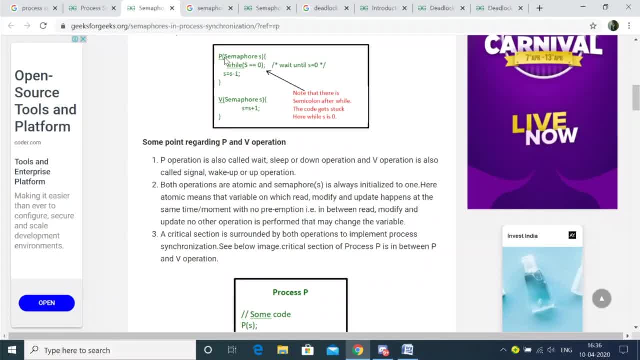 So when I say that the operations are atomic, what does it mean? Atomic means what That means, if suppose. let's say: if suppose a variable, okay, Suppose if it is in a write mode or read mode, okay, Suppose it's being. let's say, for example: 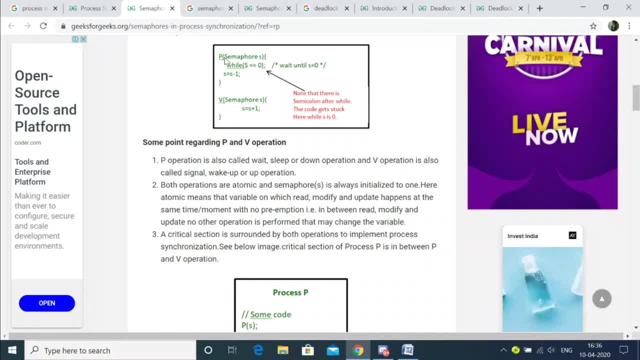 there may be some kind of operations that is being performed, okay, in a particular variable. Whatever the operations it may be, It can be write, it can be read, it can be append, whatever it may be, So that operation can be only one. 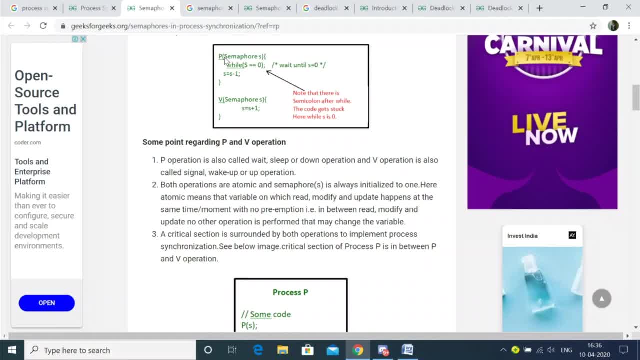 It may not, it cannot happen that multiple operations are taking place at the same period of time. okay, So that's why the thing they are saying is that the operations are atomic. That means, at one instant of time, only one operation is possible. 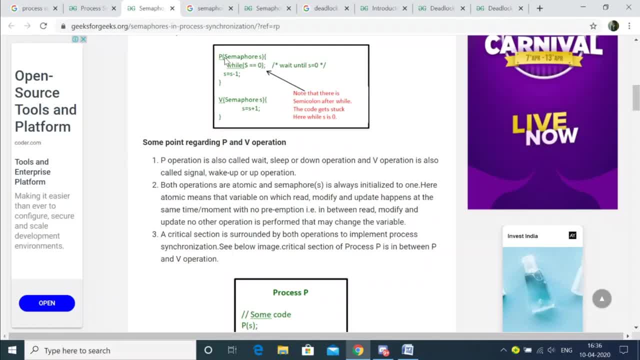 The operation can be any. It can be read, it can be write, it can be update, like what they have written here. okay, But no other operation will be. you can say, given the accessibility to change the variable At one point of time, only one type of operation is performed. okay. 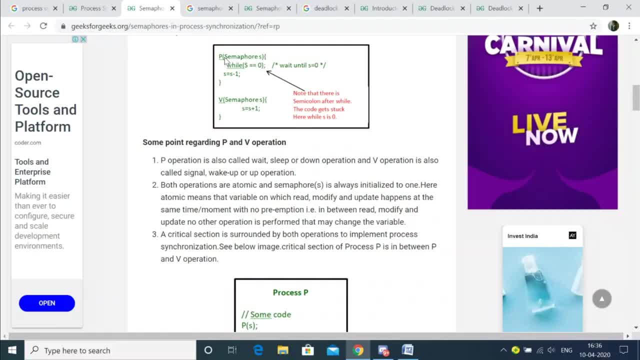 So that's what this is. one of the characteristics of semaphore: A critical section is surrounded by both operations. So, for example, we may have very big code, That part of the code of the C program which has the shared variable, so that will be entered into the critical section. 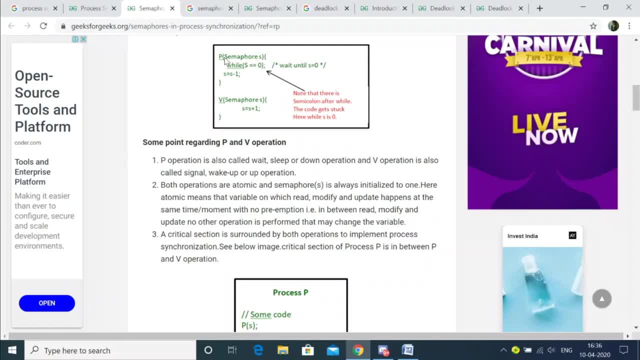 So a critical inside the critical section we will have both the operations. That means P also as well as V. P means the weight operation as well as the signal operation. okay, So let us say, for example, we are having here this block of block diagram. 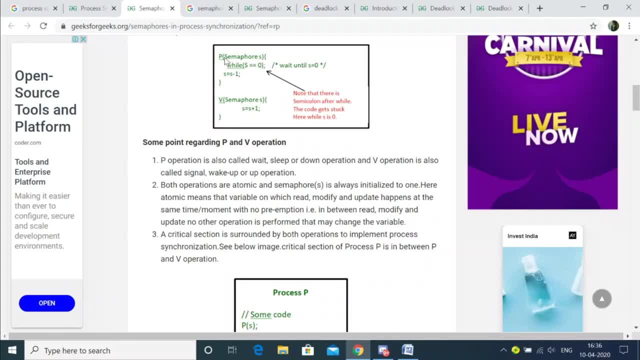 So critical section. It is surrounded by both operations to implement process synchronization. that we already know. okay, So in this image, what we are having, critical section of process P is in between P and V. okay, So P, this P, this P, this P, oblique like S, is basically the operation, the weight operation. 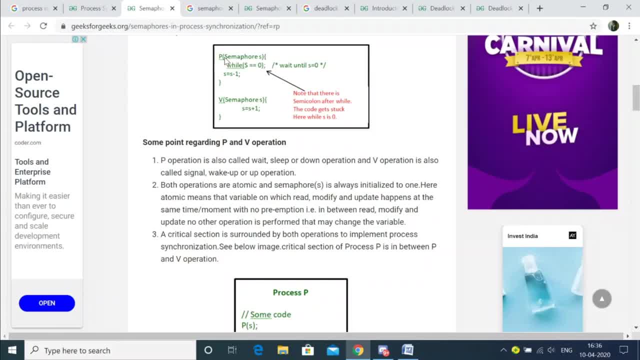 This P is the process P, this bold one. okay, This P and this PS is not same. PS is the which operation, the weight operation, And this P is basically this bold letter one P is basically the process P. 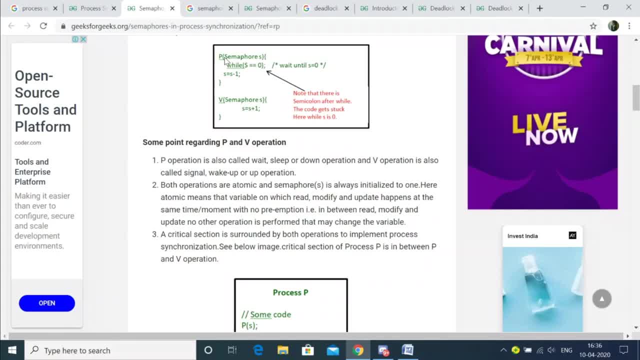 So this is the operation of the semaphoresis. okay, That is the difference. Then V is what It is, the signal. So let us see how it is being implemented. okay, So let us see how it implements mutual expression. 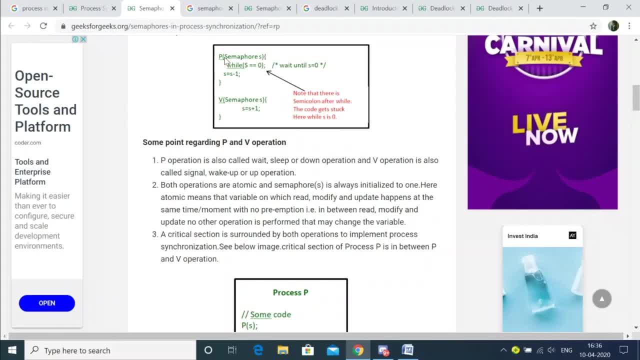 So let there be two processes, P1 and P2. And a semaphore S is initialized as one. So one thing we have to remember is that it doesn't mean that, for if there are two processes, then semaphore also will be two. 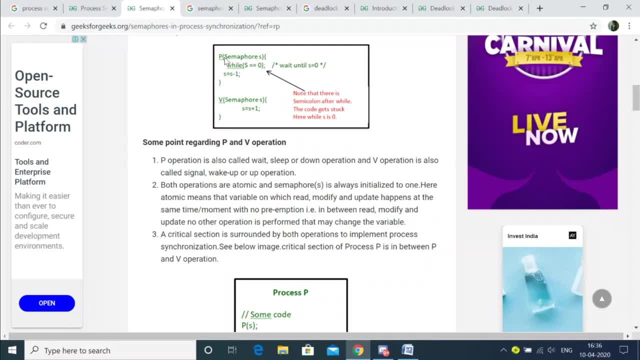 If suppose, if the two processes are linked together, if they are cooperating, that means they are sharing some certain variable, they are having certain common, then to maintain that synchronization only one semaphore is sufficient. okay, So now if suppose P1 enters: 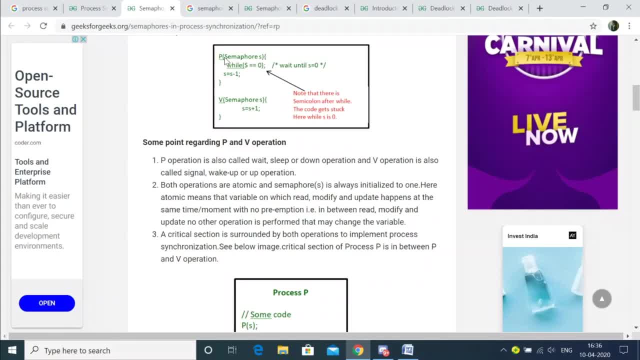 then the value of semaphore S will become zero. So what will it? what will this indicate? It will indicate that, if suppose P2 wants to enter the critical section, it cannot enter. What is the reason? Because it will see what is the value of semaphore. 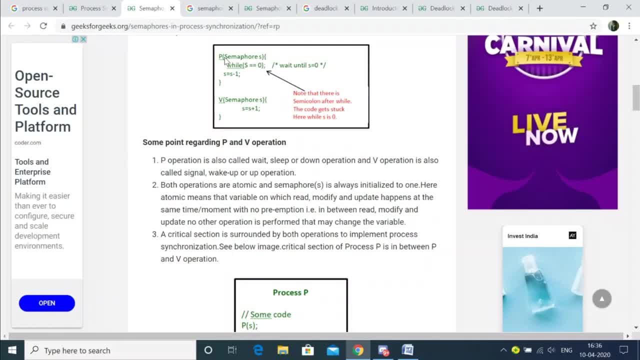 Oh, semaphore's value is zero. That means, if the semaphore value is zero, what will it indicate? It will mean that critical section is occupied by some process. That will be the signal which will go to P2,. okay, It has to wait until and unless the value of the semaphore becomes one or greater than zero. 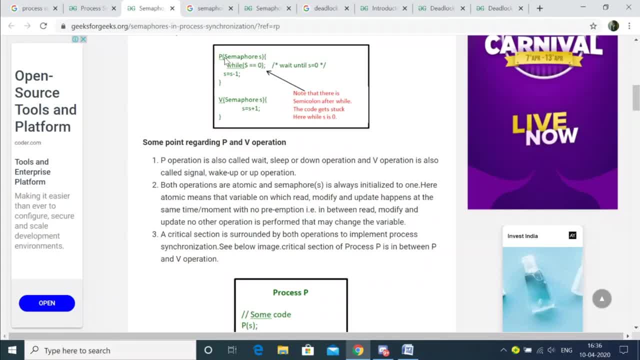 Because we know that the default value of semaphore is what? Once the default value of semaphore is one, means what? The critical section is three? There is nothing. Okay, once the semaphore value becomes equal to zero, then what message is sending to other processes? 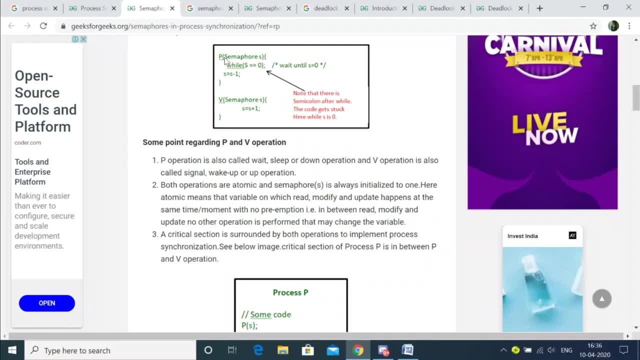 It will be sending the signal that no, we have to wait, because semaphore value- meaning semaphore value being zero- it means that some process is already there in the critical section. So we will not be able to enter, Because in the critical section only one process can enter at one time. okay, 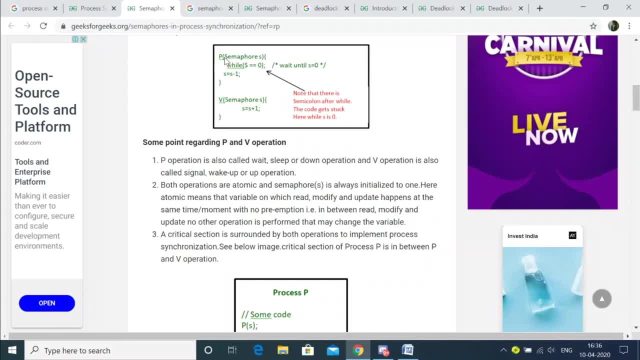 So that's why P2 has to wait until and unless the value of that semaphore changes to something else. That means greater than zero, Because semaphore value can never be negative. so it has to be greater than zero. So that's it. So this can only happen when the process P1, which is there inside the critical section, will leave it. 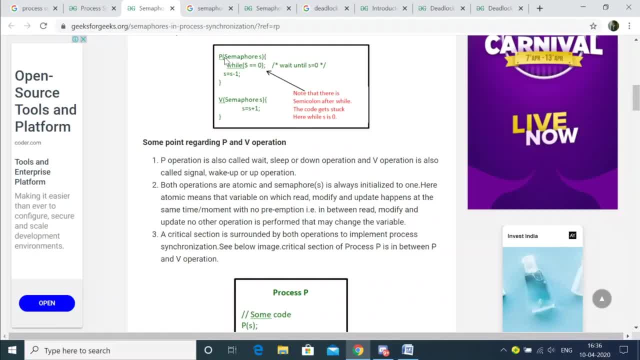 So once it leaves or before it leaves, it has to notify. So how will it notify? It will call its operation V. It will call the operation V. So V is what It is the signal That means. it is the signal which will tell the other processes that it has released the critical section. 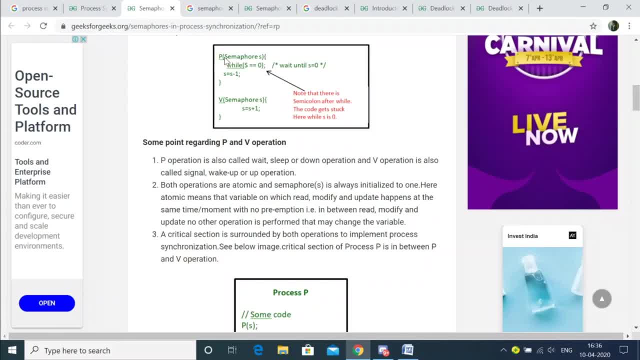 Okay, so this way the mutual exclusion is So whenever, suppose here in this block diagram also, they have said we have different kinds of situations. First situation is, let's say, P1, P2, both have not entered. 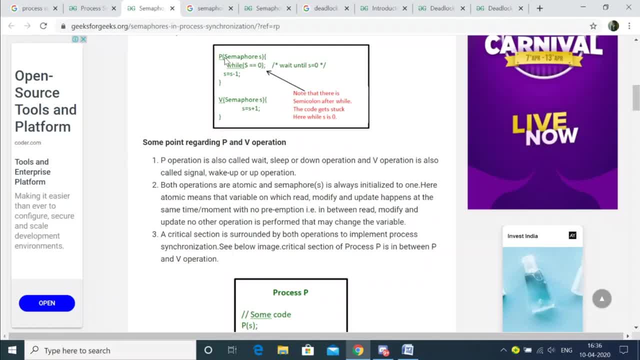 So by default the value of semaphore will be what One? only because no one is there Now if P1 has entered into the critical section, so automatically semaphore value will be zero. It will keep track of that one. So if P2 wants to enter, it will check. 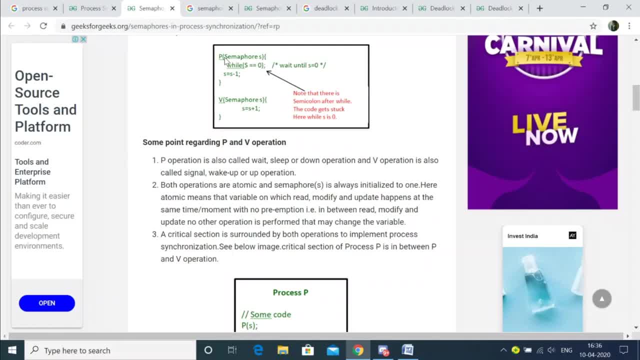 Let me check semaphore value. what is its value? so it will see. okay, semaphore is zero, that means someone is there, so i cannot enter. then next time again, uh, let's see, for example, uh p2 again, if wants to, uh check that whether it is free or not. so it will again look back. it will do a look up. 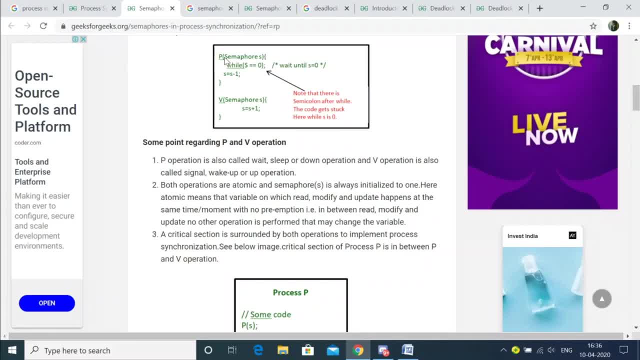 whether i can enter or not. i can still not enter, so the semaphore value will be still zero, so p2 will be restricted. then the fourth time, if, once p1 has finished execution, it has come out it has given the signal v also, v signal also is generated, that means it has released. 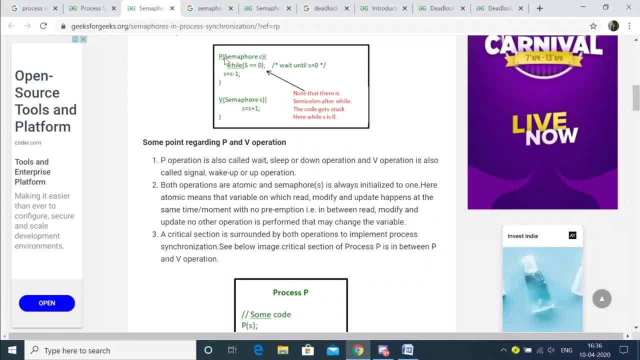 the critical section area. and so what will happen? this semaphore value will be updated. so again after some time, when p2 will do a lookup, it will see: okay, s is one is zero. that means now i can go to the critical section. okay, so that is how a binary semaphore works. now one more thing: you 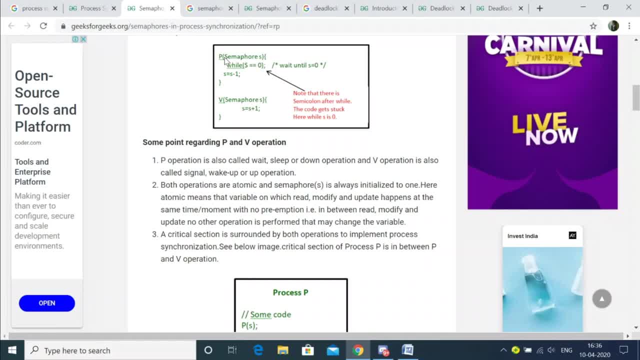 have to remember. it's not that p1 only can enter first, p2 also can enter. so if p2 is entering is entered, then semaphore value will be changed. it will be zero. so if p1 wants to enter, that time it will. it also has to. 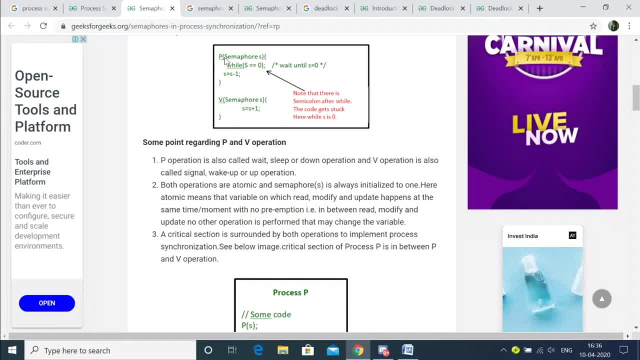 cross-reference the semaphore value. so if the value is zero, then even p1 has to wait until and unless p2 has finished, and once it has finished, so that semaphore value is updated, then when these, uh, these signals will come into play. this, um, which are the two signals? oh sorry, 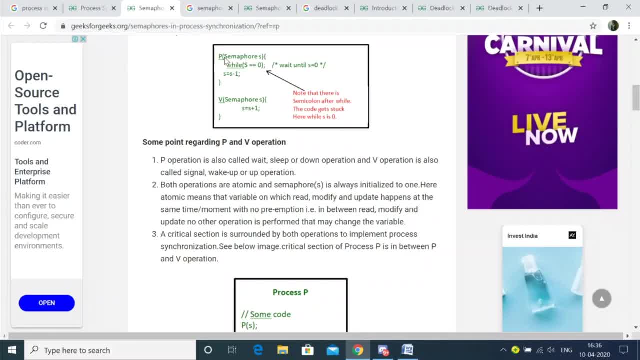 operations: uh p operation and v operation. p operation will take place once uh before uh the process is just about to enter. okay, so that means this operation will basically uh make others processes aware that you have to wait, or you have to sleep, or you have to rest or whatever you have. 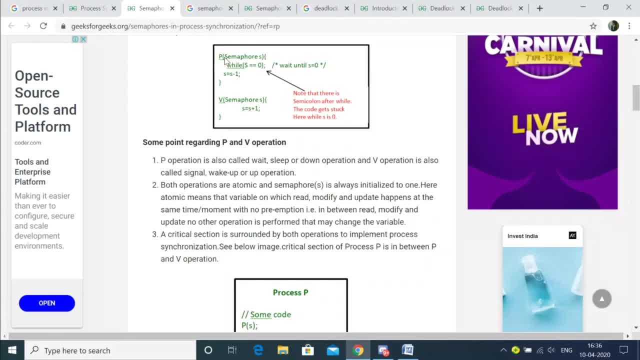 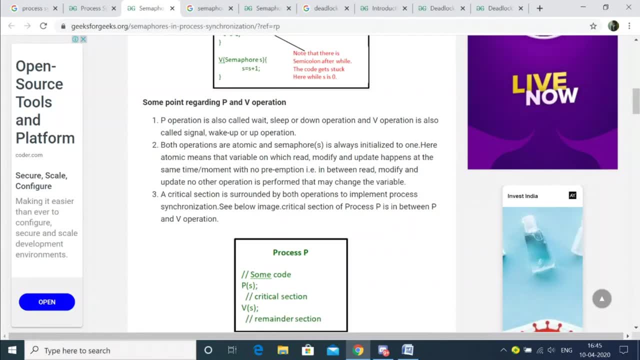 to be down, okay, you have to think. and v operation, basically once the work is done inside the critical section and after coming out, then it can send the uh signals, okay. so it's a kind of an operation which basically it's basically for notification purpose only to the other cooperating process that they 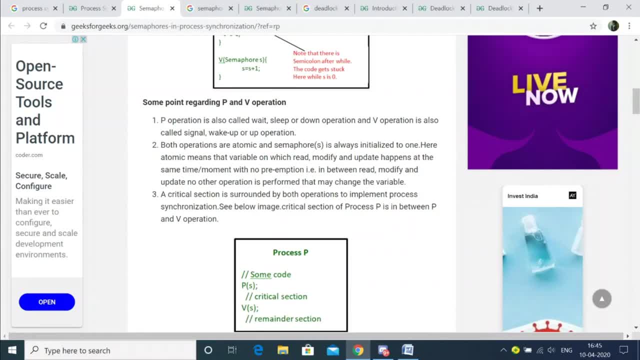 can start. okay, then another uh one uh semaphore was. uh, what kind of semaphore was there? i think it was the counting semaphore, okay. so this kind of semaphore, the binary uh semaphore, is okay for, let's say, when you have processes, uh, lesser number of processes, okay, that time you can change the values, okay, and it's much. 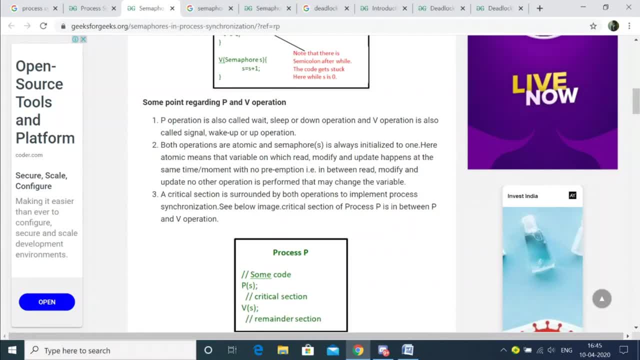 more efficient. but let's say, if we are having a situation like there, there is only one single resource but the number of processes is four, okay, but that time that binary may not be very efficient, so we have to go for a counting semaphore. so here, what is the situation? where we have a 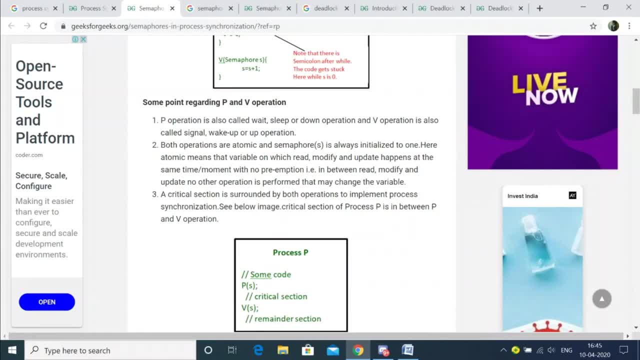 semaphore. okay, so what is the only difference? the difference is that we initialize the value of the semaphore as one and the rest of the working is same, only as binary. uh, semaphore, okay, so as value will be taken depending upon how many number of processes are there. okay, so whenever process 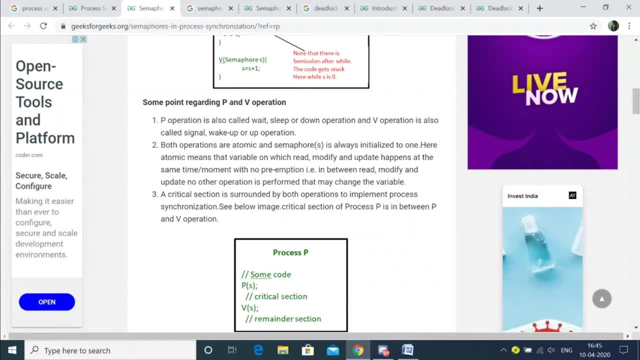 wants that resource, it calls p or wait function, and when it is done same thing, it will release v or signal function. so if the value of s becomes zero, then a process has to wait until s becomes positive. for example, suppose if there are four processes: p1, p2, p3, p4 and they all. 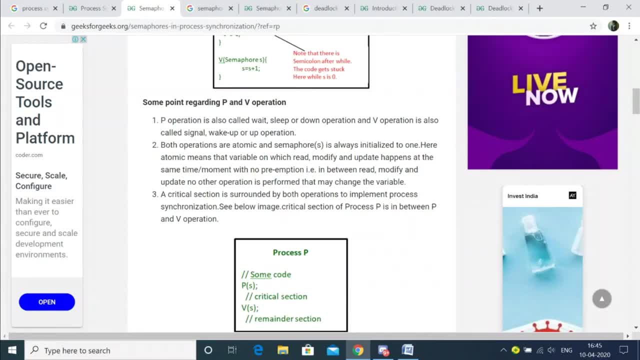 call wait operation on s. if another process, p5, wants the resource, that it should wait until one of the four reprocesses called signal function and value of the semaphore becomes positive. so same thing, only if suppose we are having, uh, four processes here. okay, let's say 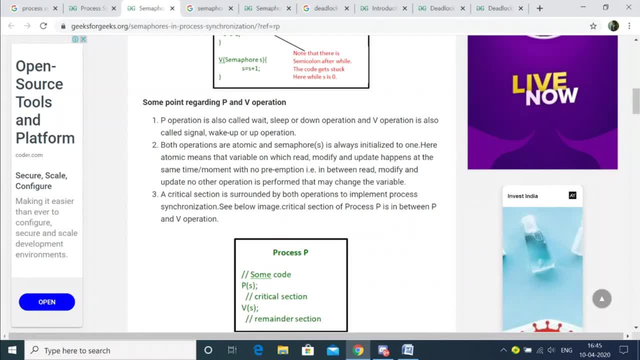 for example. so the value of this process will be how much four? now suppose if one more process comes and it wants to access that resource. so what will it do? it cannot access until and unless the value of the semaphore becomes less than four. okay, there it was. 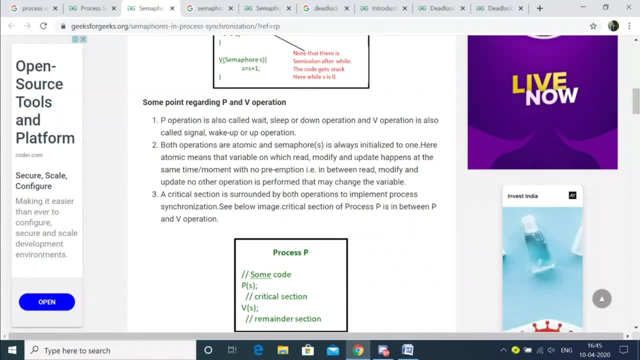 uh, less. i think it was between zero and one. one was for empty and zero was for, um, this thing, what is it called uh for? a for the process which is there in the critical section. so in this case, it will not check for zero, it will just check whether, uh, the process is, let's say, lesser than. 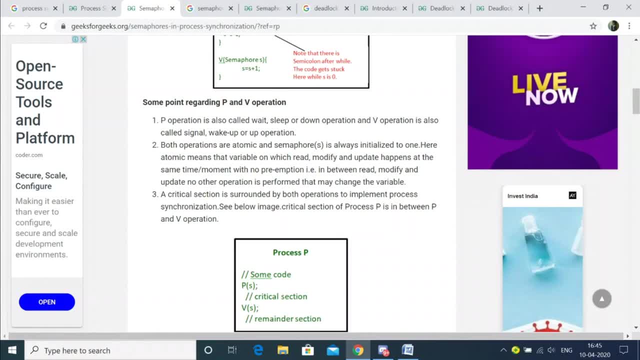 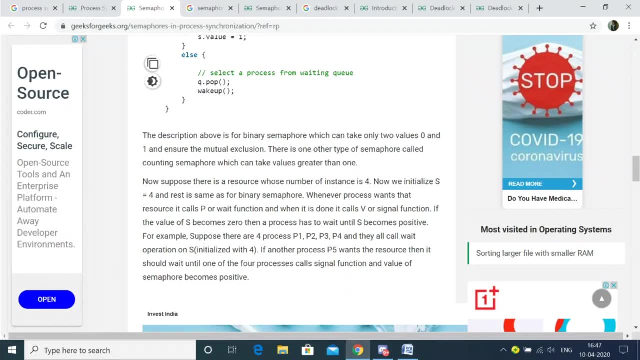 the total number of process. let's say, uh, four processes have, uh, our four processes are there and all of them have called for uh uh, the s operation. so if another process wants the resource, then it will have to wait until one of the four processes will call the signal function. 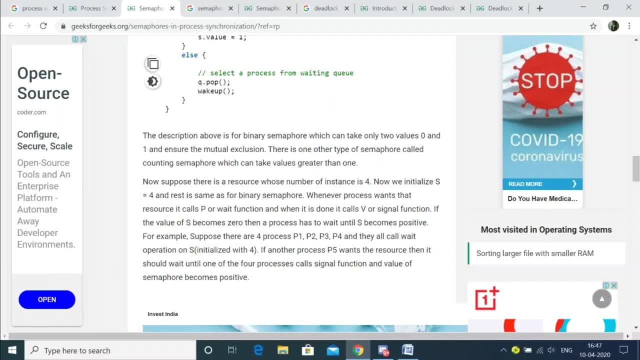 and the value of the semaphore will become positive. okay, these things are not required. okay, one thing, uh, this is important: advantage limitation. sorry, what is the disadvantage of a semaphore? one of the biggest disadvantage of semaphore is priority inversion. so what do we mean by priority inversion? suppose? 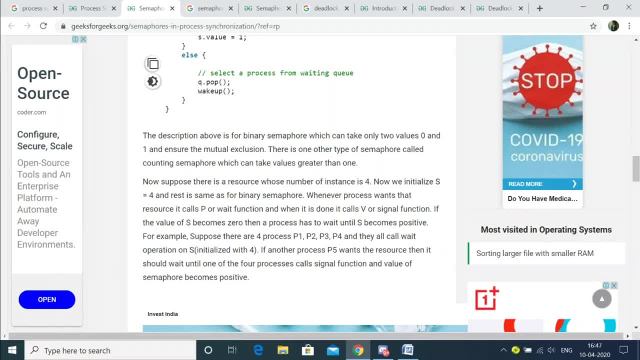 when we have a low priority process, okay uh, which has owner semaphore and let's say a high priority task has to be executed first, so the semaphore then cannot decide like which one to give, because once you are implementing a semaphore, then your priority semaphore has, we sorry, a low priority. 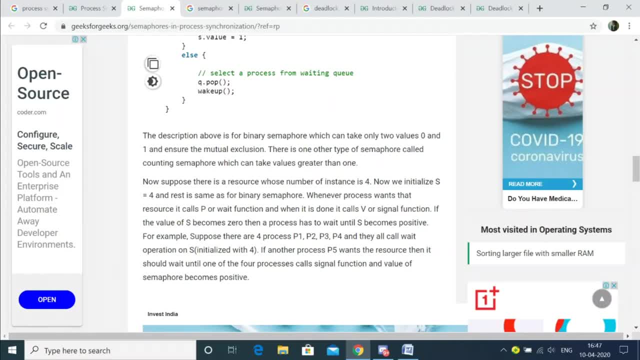 process has requested. okay, and once suppose, if, uh, you have given that low priority process to enter into the critical section- and it's a high priority process request that we are, i want to do- it cannot make a decision, then we cannot do anything. why? because it is all dependent. 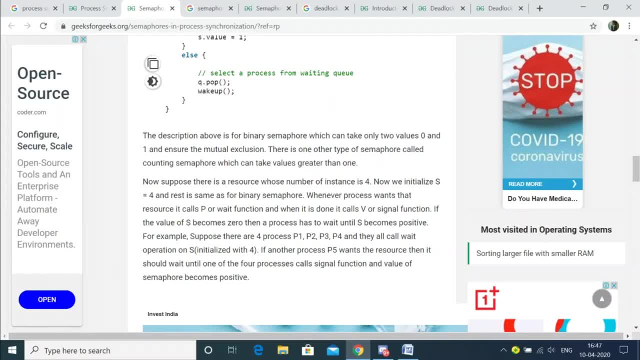 upon the semaphore value. the moment the value of semaphore is uh, you can say one, that time only we will be able to. we i mean to say, uh, i'll pick in another process. so here the priority basis of processing does not take place. so this is one of 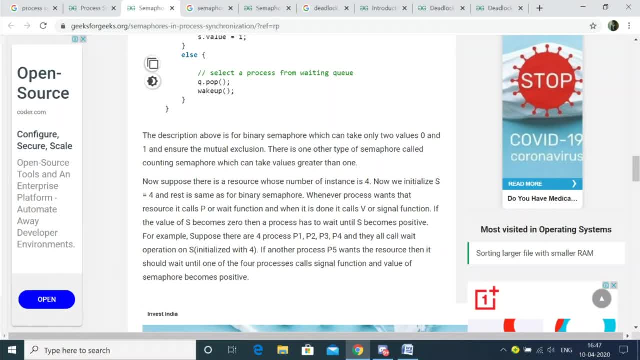 the biggest disadvantage. okay, then there is a chance of like resources utilization also, because every time the os has to keep a lot of track of the calls, of the notifications, like the weight and the other signal as well. so these kind of for a big kind of uh program or a piece of code, or if 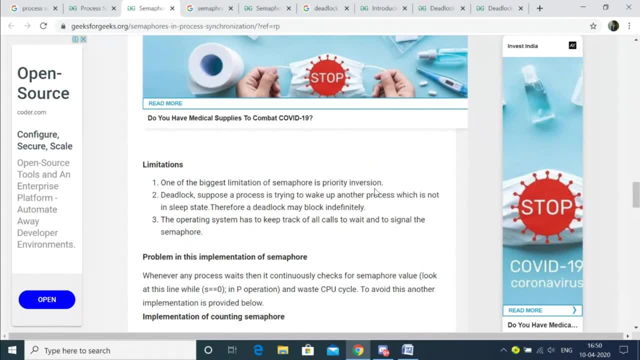 we are. if suppose multiple uh processes are there in a system, okay then that time maintaining these kind of notifications is little bit uh. you can say time consuming, resource consuming for the os. so these can be certain uh limitations, uh, which may be uh there, another one may be. it may so happen that let's say, for example, two, three processes there. 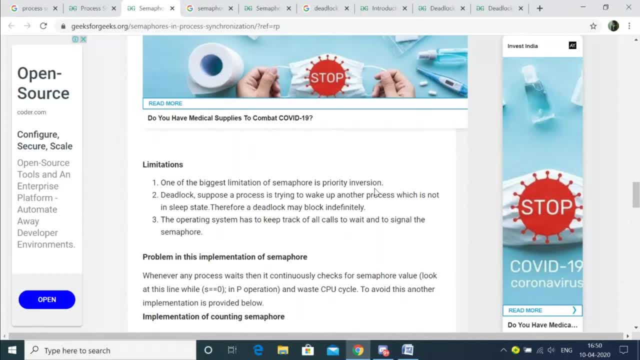 okay. so let's say, one process is trying to wake up, okay, another process, but that process is in sleep state, that is not in the active state, so it will try keep on trying to uh, uh, like that. okay, i am done, you can come, but ultimately that process has. 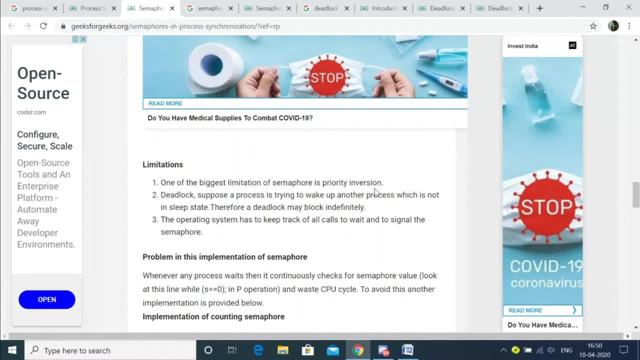 not come to that state, or maybe it is. it will not execute. certain issues. have a happen that it has been. it has gone to the sleep state, so, as a result, the system will come to a halt and there may be a deadlock as well. okay, so these are the issues that may be there with the 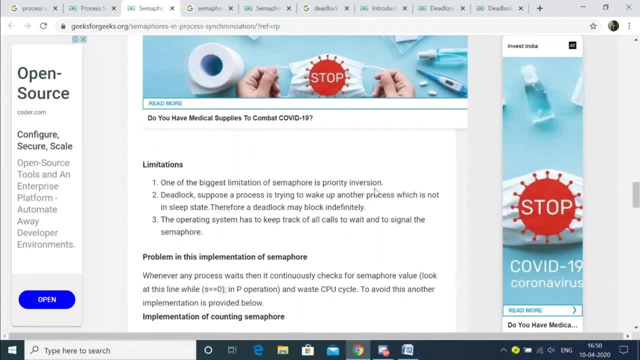 semaphore, i think it's only No. in counting semaphore, the value is not 1.. In binary semaphore, the value is 1.. In counting semaphore, basically, the value of the semaphore will be dependent upon how many number ofs will be there. 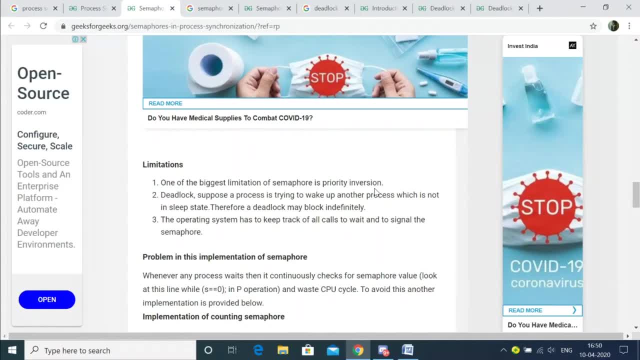 For example, if we have 4 number ofs, so that time, let's say, one of the processes is executed, So what happens? Okay, So suppose one second Example: we have a resource, So here the value of the semaphore will be 4 in counting process. 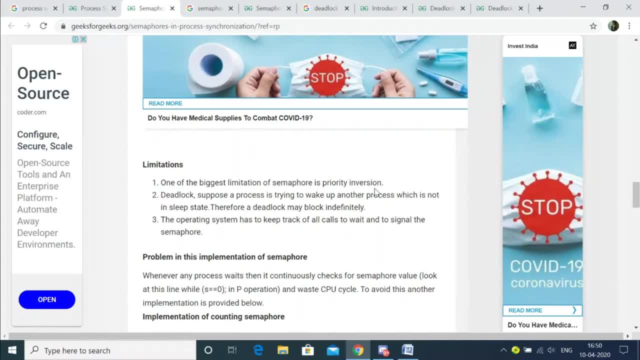 The value of the counting semaphore will be equal to the total number of processes, The working binary semaphore. So whenever a process wants that resource it calls p or weight function, And when it is done it calls v for signal function. So same way, only in the above one also. 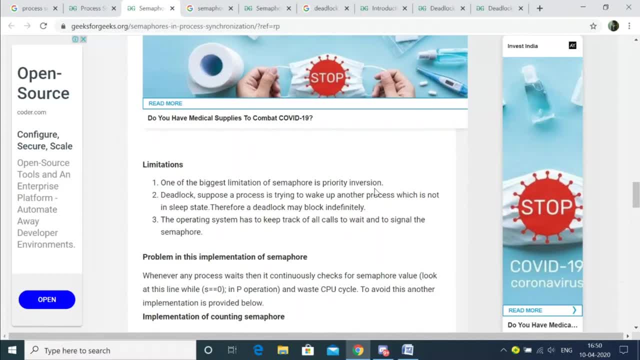 If suppose one process wants to make use of available resource or data or whatever It may be, it will first generate a notification. That means that p will notify to all that you all have to wait, And once it is done then it will generate another notification. v. 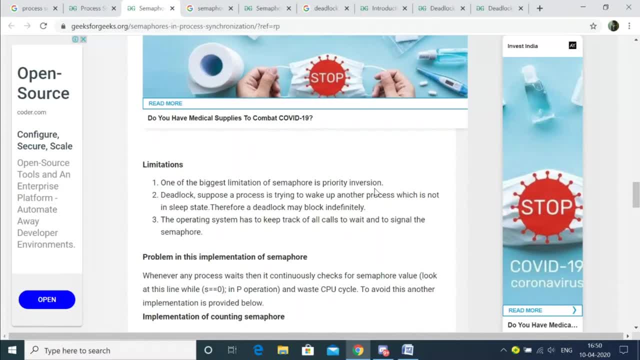 That means a signal function. It will tell that I am done with the critical section. You can come Now. if the value of s becomes 0, then the process has to wait until s becomes positive. So if the value of s becomes 0, then a process has to wait. 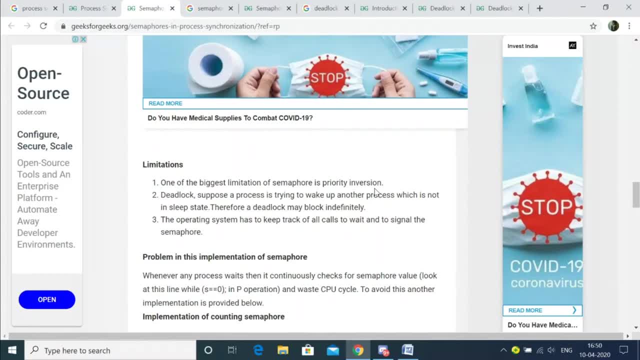 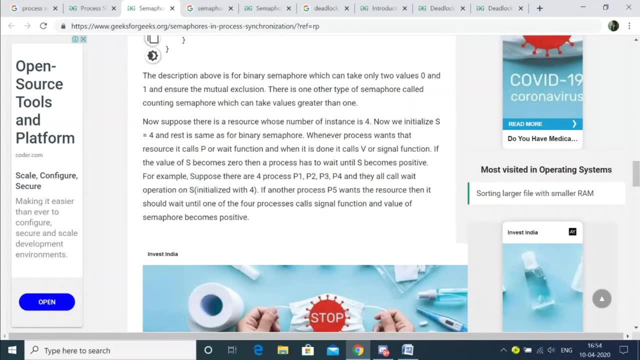 until s becomes positive. okay, let's see. for example, suppose if there are four processes- p1, p2, p3 and p4- and they all okay, this, what is it saying? is that, suppose, if we have four processes, okay, so, uh, one has executed, so initial value was four. okay, so after one has executed, then 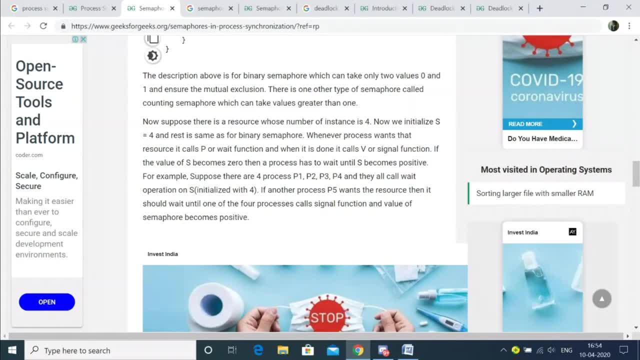 there will be a decrement in uh process p2. it's like they're maintaining a kind of q structure once p2 has uh. like they have maintained a kind of an order: p1 has requested first, p2 has requested second, p3 has requested third and p4 has requested for the fourth. okay, so p5 has not. 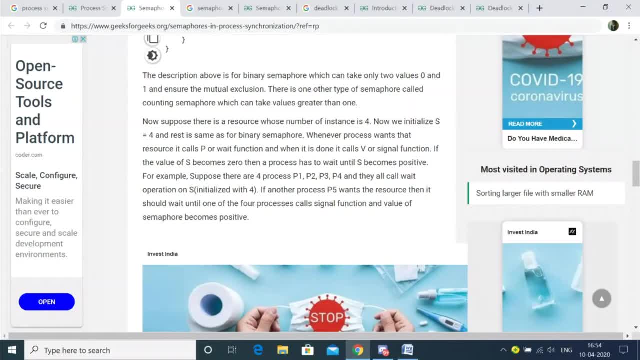 come only as yet into the system. so that's why the value of semaphore is how much? four, now p1. once it has, uh like, entered into the critical section, the semaphore value drops. it becomes three. okay, so p2, p3, p4. okay, p5 has entered, okay, but p2, p3, p4 has already issued the signal. that is, which signal rate? 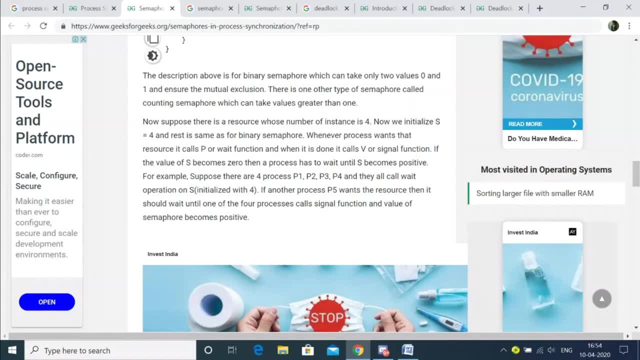 signal. okay, in order. p1 gave first, then p2, p3 and p4. now can p5 be given the critical section? no, so till when it it will not be able. it will not be able to access the critical section until and unless the semaphore value becomes equal to zero. and when will the semaphore be? 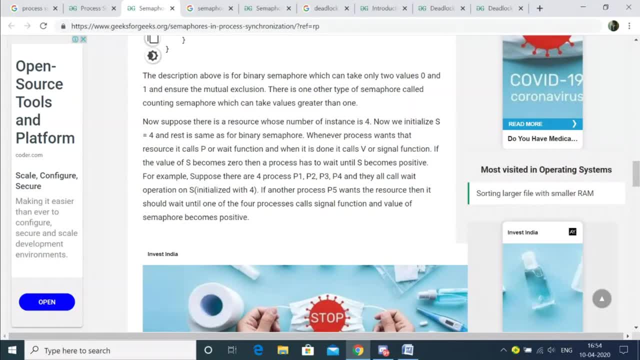 available becomes equal to zero when each of the processes has executed, because with first process being executed from four, we are having p2. when it will be executed, it will be one unit less, p3, one unit less and ultimately, with p4, the semaphore value will drop to zero. so once it is dropped to zero, 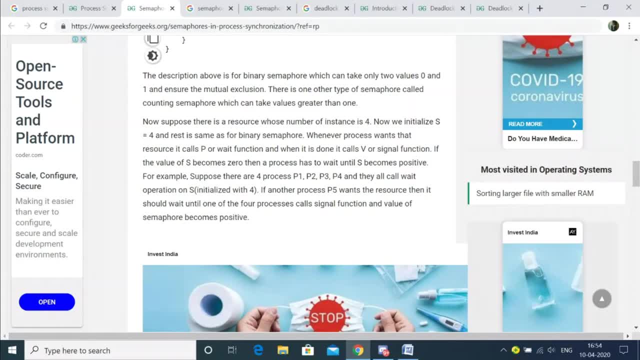 then we can give the allocation for p5- here the assumption has been taken that they have already uh given the request for the semaphore value- and then we can give the allocation for p5 here. the but one thing you need to be aware of is that when a second turn by t4 comes next, 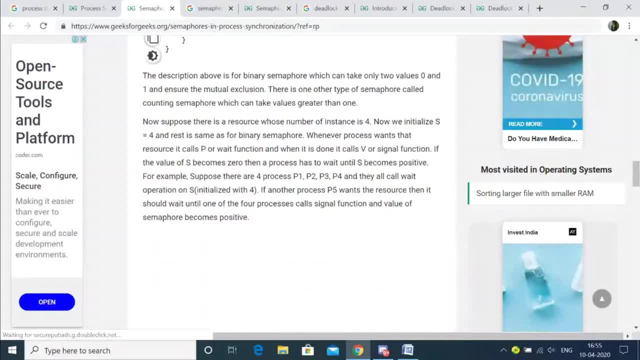 the sting will even increase and then die because what I have done here, let's False Никง Image. Anyway, P2, P3,, P4, it's fine, They know like which one will go accordingly. But for a new processes, enter the system altogether. 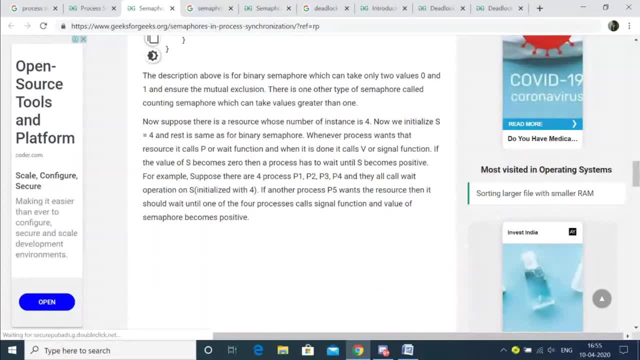 it has to wait until and unless the value of that semaphore becomes equal to zero. I hope that it answers Anyone else. Okay, did we talk about deadlock before? No, sir, Okay, Okay, So deadlock is also one of the most. 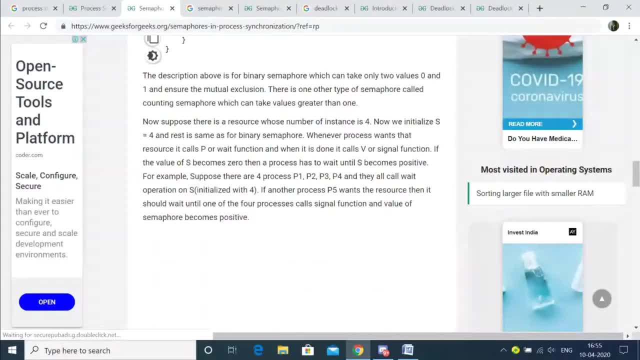 important part of operating system and process synchronization. So from the name itself, deadlock, that means certain thing has been locked, It has come to a standstill, Okay, Nothing is, everything is blocked. you can say Okay. So deadlock is a kind of a situation or a problem. 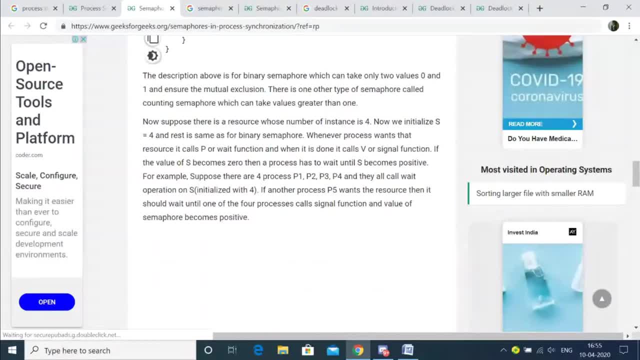 you can say, where there are a set of processes which are blocked, They are unable to execute, They cannot go further, They cannot come out of that kind of blockage. Okay, Because each process is holding certain resource and waiting also for some other resource acquired by some other process. 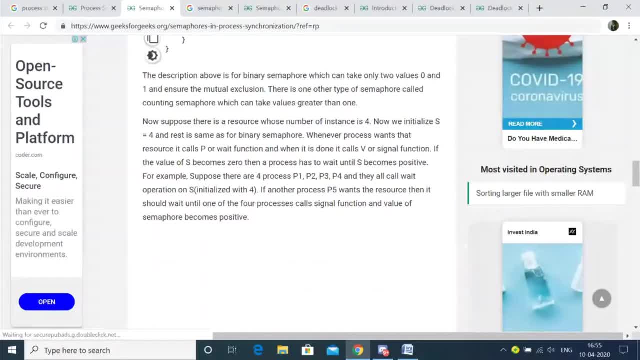 Okay. So in a deadlock situation, what is happening? A process will have a resource, but it is also, at the same time, expecting or requesting a resource. That resource- again, it is being allocated to some other process, So it becomes a cyclic nature. 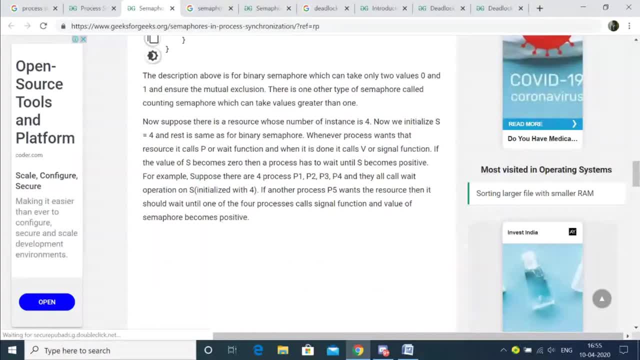 Okay, It has come to a standstill. So consider an example. Let's say when two Trains are coming towards each other on the same track and there is only one single track, then what will happen? None of the tracks, none of the trains will be able to move. 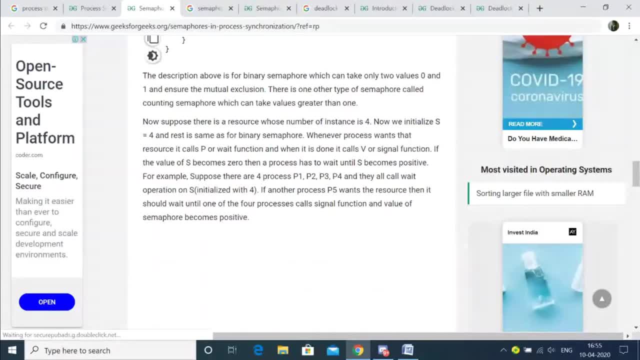 Okay, Once they are in front of each other, can they go back? No, Can they move forward? No, it's not possible. So such a situation is your deadlock in real life situation. So below is kind of a diagram, if you see. 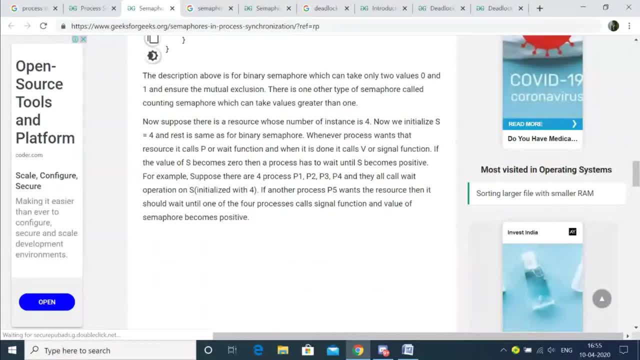 So this is the complete deadlock situation. So we so here. let's say, for example, we have a process one, process One is Uh, having a resource, uh one. that means resource one is given to process one, but process one still wants something else. 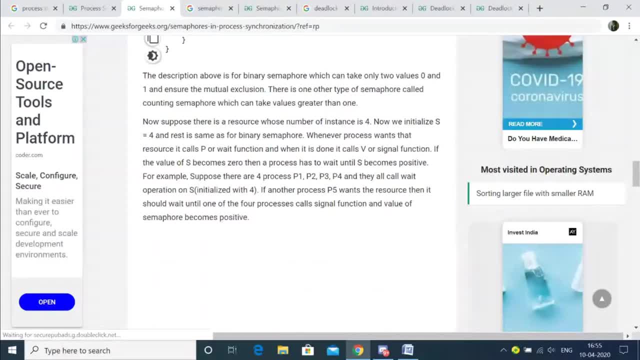 So what he wants? he wants the resource to similarly process to what does it have? uh, like having. for the resource two is being allocated, but process two is not happy. He wants resource one as well. So, despite their having the resources, they are still looking for some other resource. 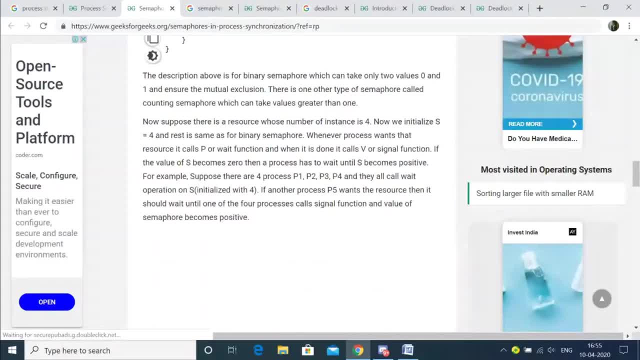 So, ultimately, what has happened? it has come a deadlock, the cycle is cyclic pattern which is unable to break. So this is waiting, This is a sign, This is waiting, This is a sign Okay, So they are unable to do the work. 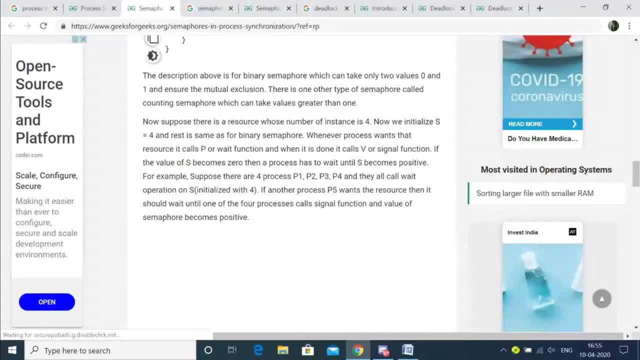 Okay, Now, in which kind of different situations we can have uh a deadlock? Okay, So these are the various uh situations. One is: uh a mutual exclusion. Deadlock can arise if following four conditions takes place simultaneously: 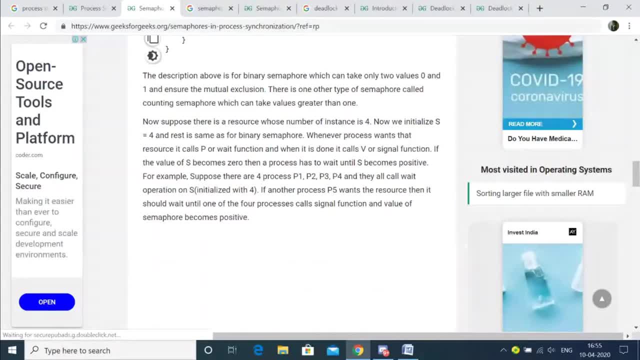 Okay. So if each uh of the conditions uh take place at the same period of time, then We say that deadlock is happening. So first is mutual exclusion: one or more than one resource are non-shareable. So only one process can use at the time one or more resource. one, one or more resource are non-shareable. 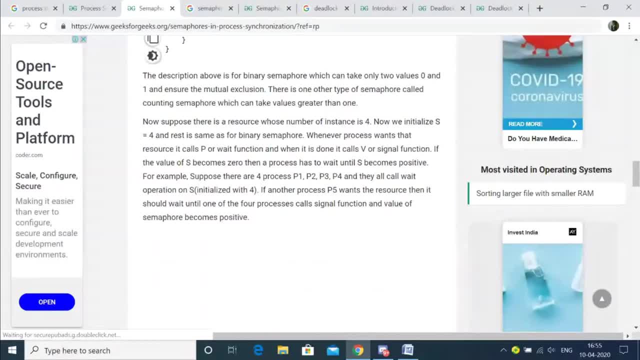 That means we are unable to share the resource, Like, for example, here. this resource is share is given only to here. Okay, It's not shareable, though It's requesting, but it's not shareable, right? You suppose, had it been, this resource was common to this. 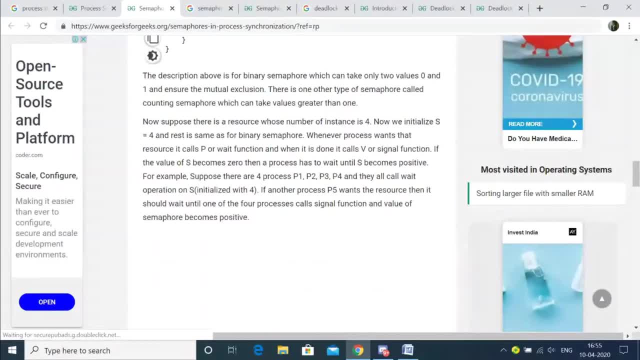 Both the process then this cyclic pattern, we would not have got Okay. So that is one of the major point here. Mutual exclusion is not with regards to process, here It's with regards to resource. Okay, Hold and wait. So this is all same. like diagram, a process is holding at least one resource. 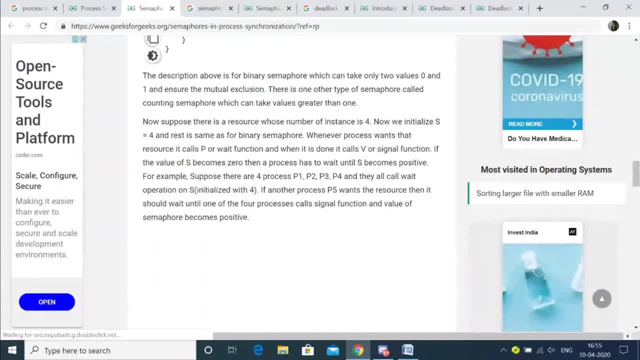 It is getting one resource. It is being allocated, but still it is waiting for some other resource also. Okay, It's not happy, So it has to hold. It is holding one resource, Like resource that he has got, but at the same time he's waiting. 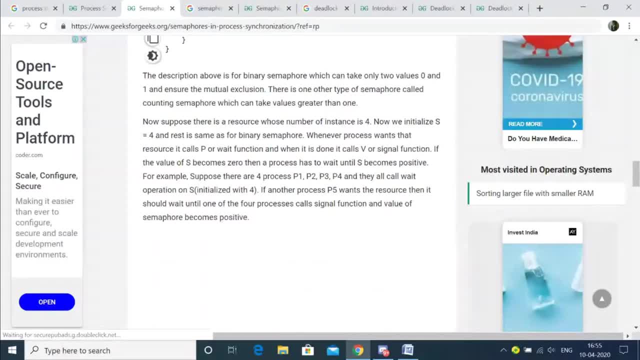 for some other resource also. So that has become like a hold and wait. It is holding the current resource and it is waiting for some other resource which is not available. Then no preemption. That means a resource cannot be taken from a process until the 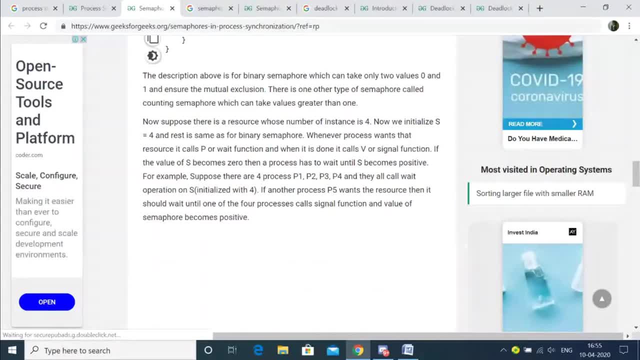 process has itself released the resource. So what has happened? Resource doesn't have the power to come out from a process. The process has to release. So, ultimately, what will happen? That resource will remain unavailable Until and unless the process doesn't wish to release the resource. 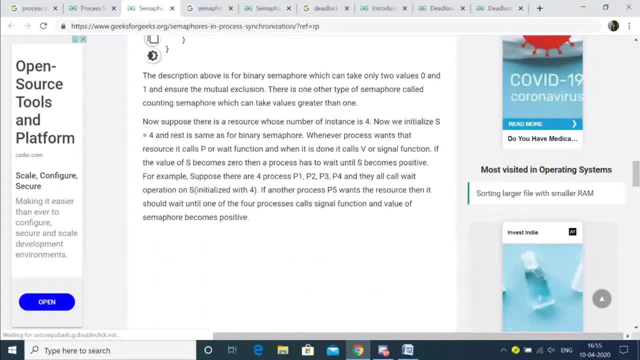 So this is also one of the dangerous condition for a deadlock to occur. Then circular wait. So you suppose we have a series of processes which are in circular pattern, So that indicates deadlock, Like for example, here we are having only two processes. 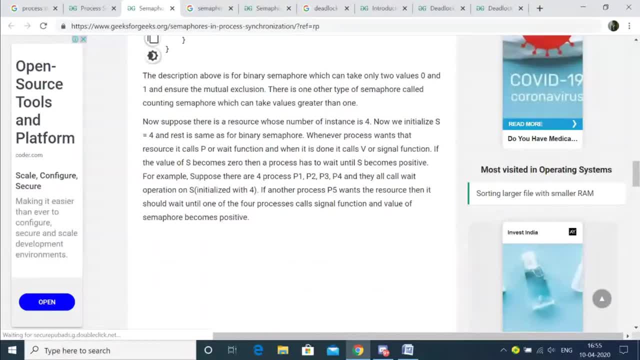 So this actually shows you a condition for deadlock. Okay. So these are the four conditions that we are that we have to be very careful that we should not allow it to happen, Because any of the conditions, or if all the conditions or any one condition also, if it takes place, then the chance of having a deadlock- okay, it becomes very, very strong. 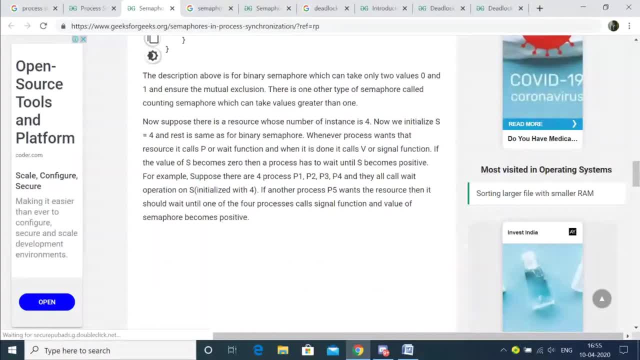 Okay, So how are we going to handle the deadlock? So here I think that Banker's algorithm comes, So maybe tomorrow I will do that algorithm. I think there was a lot of requests also regarding that algorithm, So maybe tomorrow hopefully. 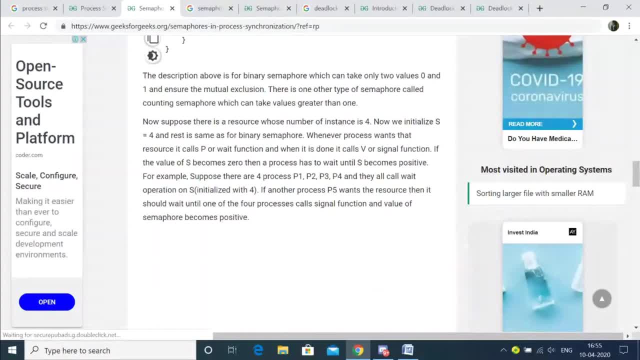 Okay, So what are the various methods? So there are three ways to handle a deadlock. One is deadlock, prevention or avoidance. Okay, So what does it mean? Prevention means what Means the concept is something that we will not let only that such kind of possibility to arise. 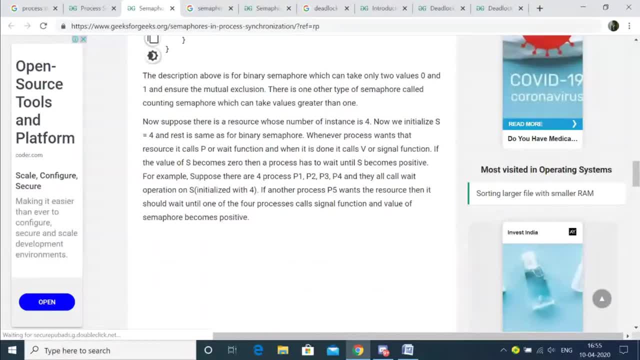 Okay, Avoidance means we will maintain certain strategy, certain means or certain algorithm. We will design Such that we will try to avoid if certain such kind of situation arises. Also, we will try to counter that one. Okay, So one very popular algorithm is the Banker's algorithm. 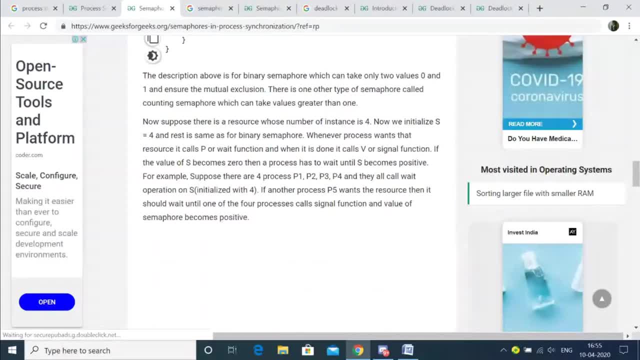 Okay, Which is being again designed by Digistra, Okay, In order to avoid deadlock. So questions may come that write up algorithm designed by Digistra for deadlock avoidance. So they may not ask you directly that it is Banker's algorithm. So you have to be a little bit. you have to understand, okay, the question. that another one is deadlock detection and recovery. 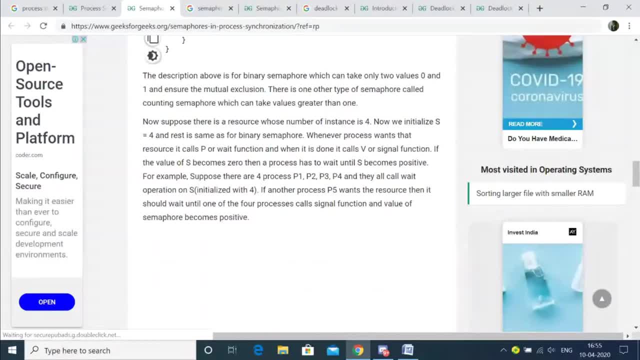 So what has happened here? We are not taking prevention, We are letting it to happen, Uh and. but we have certain measures like how we can recover from that situation. So what do we do? There will be certain kind of measures of how we can uh know that the deadlock has taken place. 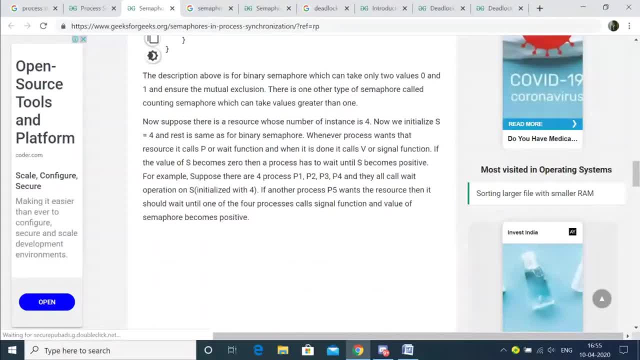 If the deadlock has taken place, then there will be certain recovery mechanisms, Yeah, Yeah, And then those mechanisms we will be able to come out of the deadlock, Okay, And one is like the most, uh, the rest of the red, which generally we don't follow. is that not the deadlock? 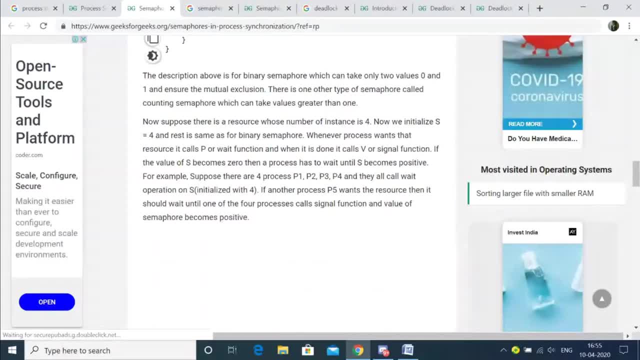 Let it happen. Okay, So this, uh, so what do we do? If suppose the deadlock, if the system comes to a standstill, it's not working, We just reboot the system. but basically we, we do it in windows and Unix, but for multiprocessing or sorry for yes, for. 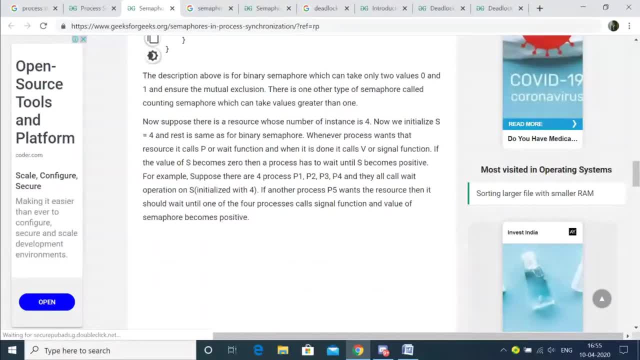 multiprocessing, or for, let's say, you are a system And we need to fledged the usual Uh and uh uh, you know, uh uh, safe, safe systems which are very much critical in your uh scientific approach. 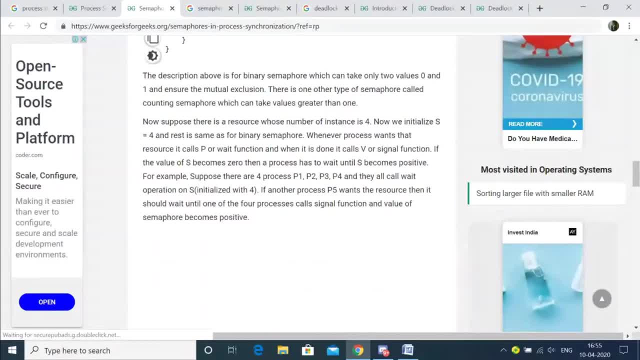 So that time we can undo, we have to avoid such kind of uh issues. Okay, So, uh, first one, that is the deadlock, uh prevention. So we already know that. what are the characteristics for uh or uh, the characteristics that uh, we can have that lock? mutual exclusion here. mutual exclusion means 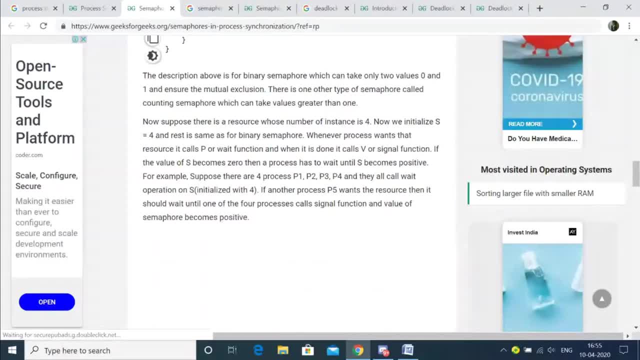 this kind of deadlock situation may arise. hold and wait means what a resource is being held up by some process- okay, and that process is waiting for some other resource- okay. so what has happened is it is holding also certain allocated resource that is being given to him at the same time. it. 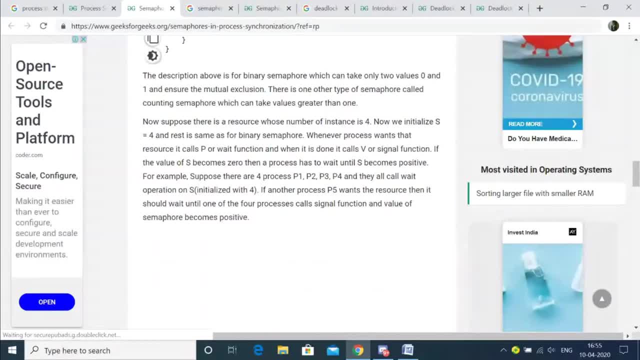 is waiting also for some other process. so, as a result, what has happened? it is in a standstill position. no preemption means. let's say, for example, a deadlock has taken place but the resource cannot come out on its own. the process has to release the resource from the system. 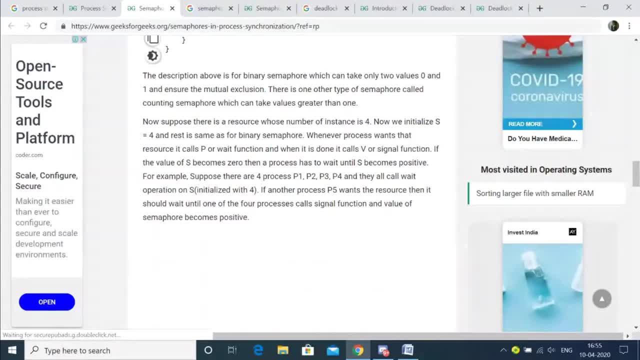 then only the resource can be free and that resource can be allocated to some other process. but in this kind of situation resources are, like you can say, dependent upon the release of the process. until and unless the process doesn't release, the resource cannot come. so this again. 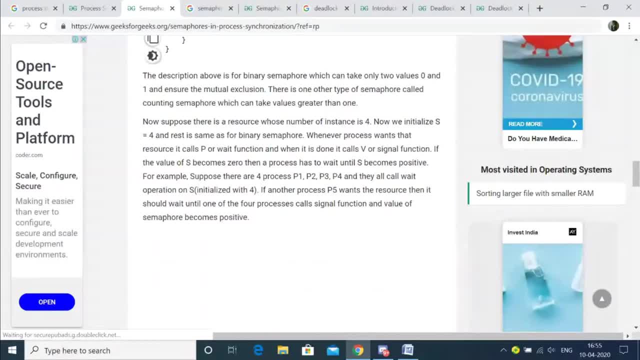 it's a no preemption. that means there can be no interrupt in between you, okay. circular wage: that means all of them are waiting in a circular structure. it's a cycle. once the cycle is there, then we say that deadlock has taken place. okay, so, as we said, that there are. 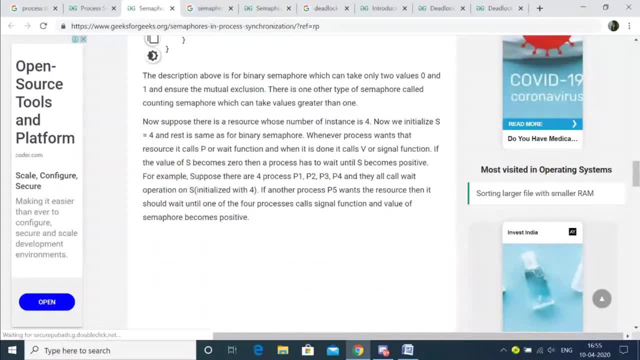 various mechanisms of how we can handle deadlock. one is the prevention. that means in beforehand. only we take certain measures through which we can eliminate deadlock. so one is that eliminate mutual exclusion. so it is not possible to dissatisfy the mutual exclusion because some resources, such as 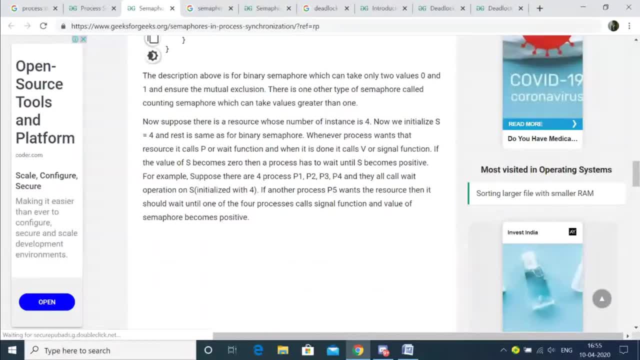 the driver and printer inherently non-shareable. so it's okay, for certain things which are non-shareable we can make them non-shareable, but for the ones which are shareable, we can definitely. for the resources which are shareable, definitely we can share it through a via different. 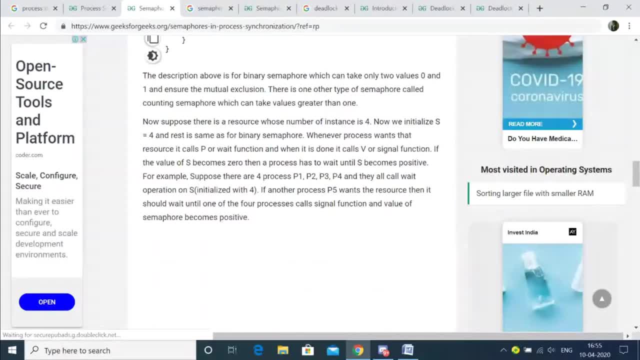 processes, okay for different. then another one is: eliminate, hold and wait. so allocate all required processes to the process before it starts execution. so we are not waiting that beforehand, only which process will be given or which process has to wait. what we will do, we will allocate all the required process resources. 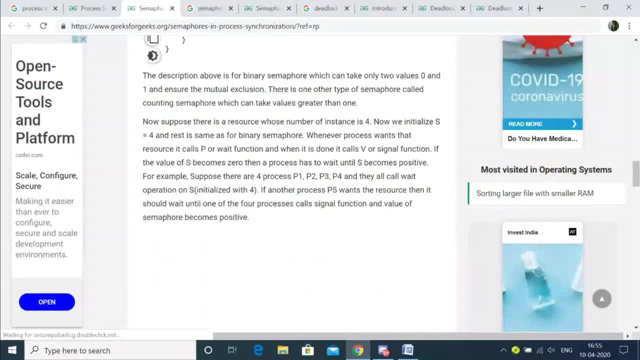 to the or to a process before the process starts its work. okay, this way, hold and wait condition is eliminated. okay, for example, if a process requires printer at a later time and we have allocated printer before the start of execution of its execution, printer will remain blocked till it. 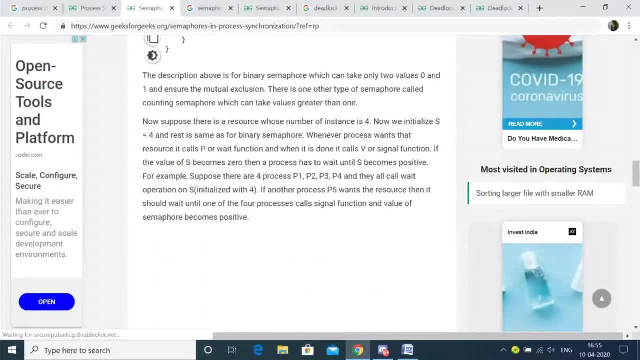 has completed its execution, the process will need and make a new request for resources after releasing the current set of resources. okay. the solution may, however, lead to starvation, okay, so what has happened is we will make a situation such that, until and unless a process is has not. 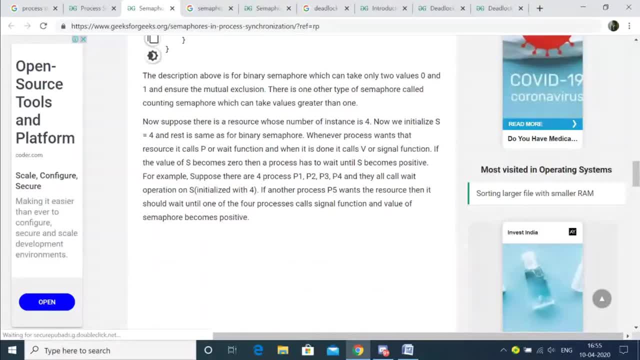 you can say: released a resource. he cannot request for anything or refresh resources. let's say, for example, one resource is being allocated to a process, okay, so that process is holding the resource, but it cannot, uh, request for a new resource. that time it can. it can request a new resource, or only when it has released. 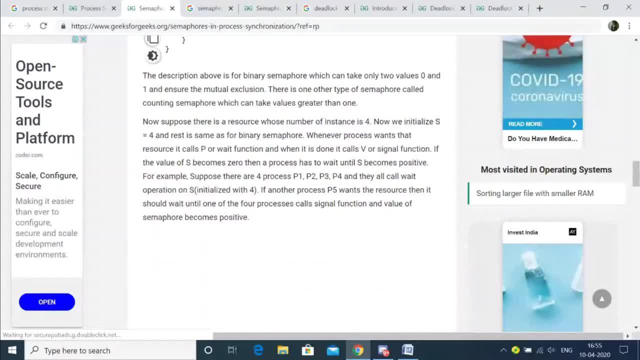 the current holding resource. so ultimately that hold and wait condition is removed. but one thing they have said is that there will be starvation. that means what the process has released, the resource- not be any resources available at that time, because all the resources may be allocated to some. 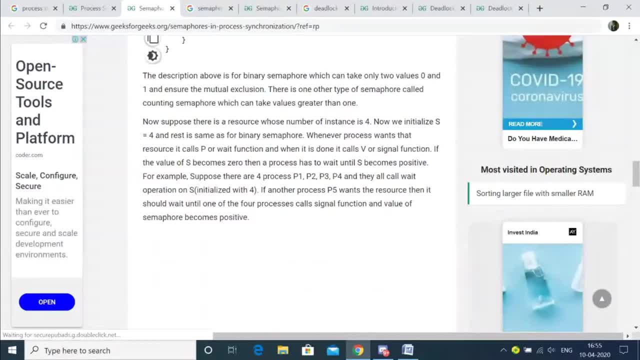 other processes. so that may be one kind of challenge, okay, and another thing is that we may, let's say, for example, the process has not started its execution. okay, yeah, it has got the uh allocated, it has already been allocated the resource, okay, but uh, okay, one thing: allocate all required. 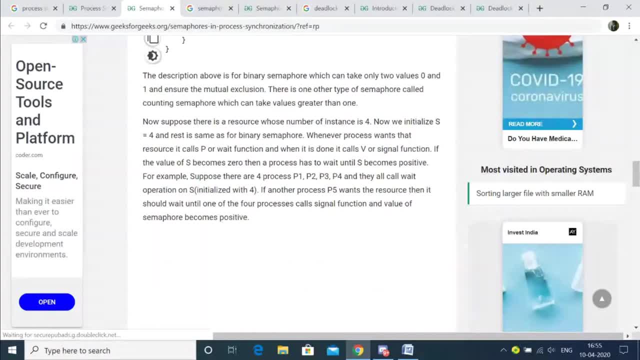 resource to the process before the start of execution. okay, so we are allocating the resources to the process before the process has started to work. okay, so this way what will happen? hold and wait condition is eliminated. that means to one process we are giving directly allocating many resources. so ultimately, what what will happen is that process will basically consume. 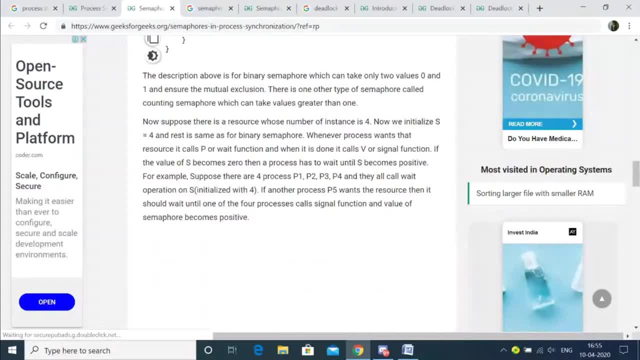 all those resources and other processes will be. we cannot uh direct the uh request because here, what are we doing in uh, in this uh deadlock prevention? once the resource is allocated, that resource cannot be requested by any other process. that is one of the most important thing. if one of the 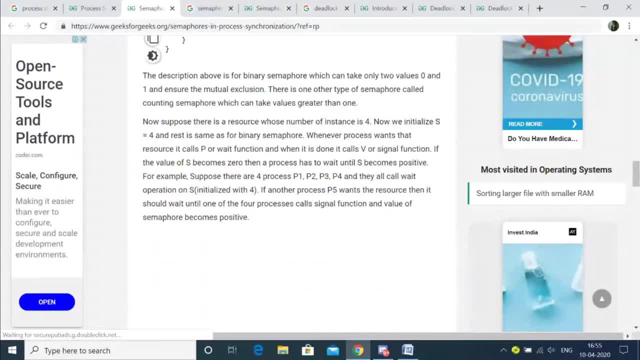 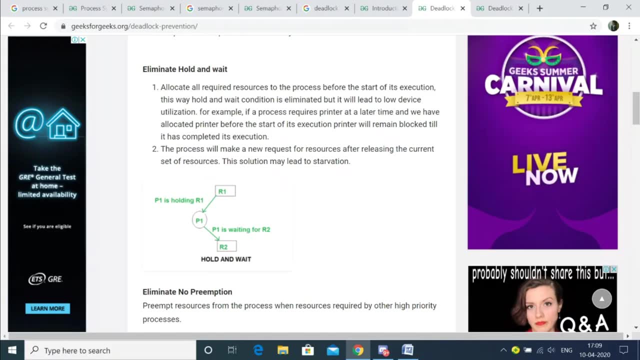 resources. or if let's say two, three resources are allocated for to one process, then those two, three processes resources cannot be requested by any other process. so there is no hope and wait. it is given. so once it is given means others cannot shout that. give it to me. 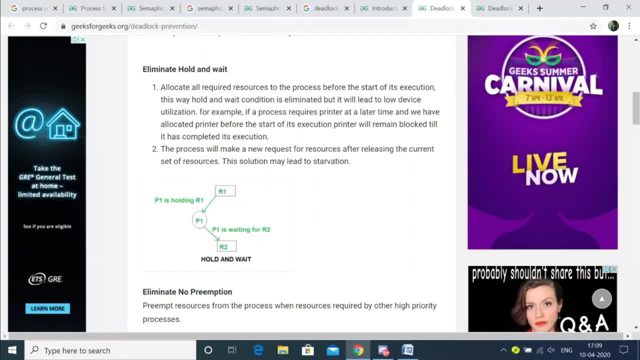 they. it will be with that, with that process, until and unless he decides to release them. so let's say, if that one process has occupied four resources, so all four will be with him, but others- they have to mean keep quiet, they cannot request. so there is no hold and wait, there is no waiting. 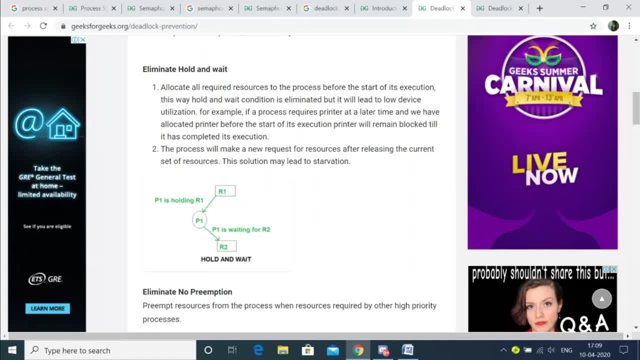 here. so once it starts releasing, then after that others can give a request and accordingly they will be assigned. eliminate, no preemption. so in the earlier case we have seen that once the resource is allocated we cannot break it or interrupt in between. only there is no priority inversion. as we said, that means if a higher 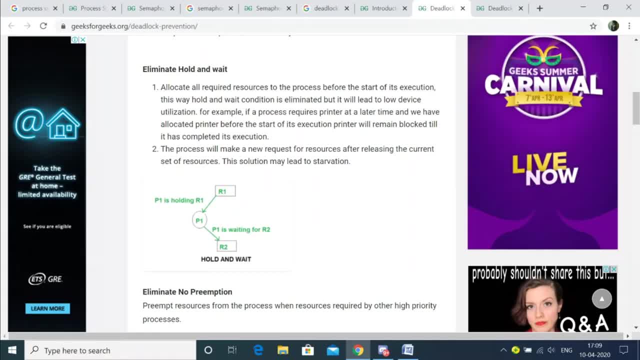 priority process comes. then we have the higher priority process. also has to wait until and unless the resource is released by the process. but in this case and eliminate no preemption. we can preempt, we can stop in between, release the resource and give it to the other process. 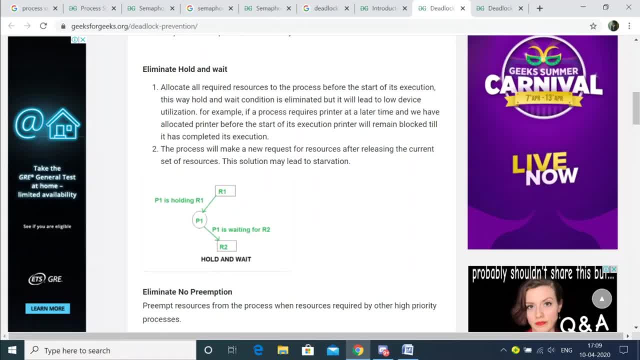 the high priority process. so how will the os know there will be some priority number? okay, that the os will be fixing. so accordingly, the operating system will check if, even if, suppose, one resource has been given to a particular process but another process comes and that process is holding a higher priority than the current one, then immediately the resource will. 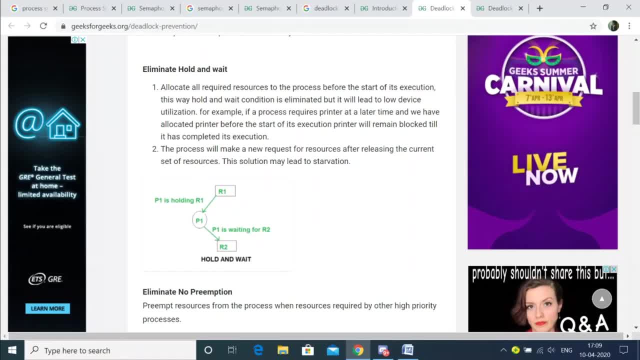 be truncated and given to the higher priority process. so there is a breakage. okay, according, then eliminate the circular weight. okay, so each row here they have said only each given a specific numerical number. so accordingly that process can request the resource in the increasing or decreasing order of those numbering of processes. okay, 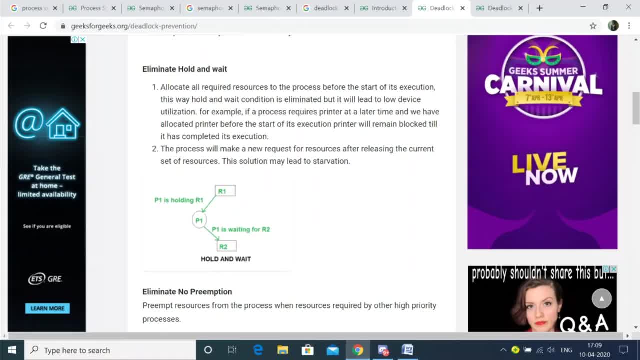 deadlock avoidance. uh, there is an algorithm that will be there, so tomorrow probably i'll do is a very big one you have to. okay, Industrialless, um, so yet not except check. yes, i did give assignment, but yesterday, uh, i asked the class that, Uh, should i, uh, do i mean to those areas, right, others they requested, like they asked the other. the other tomato is some type of askew. 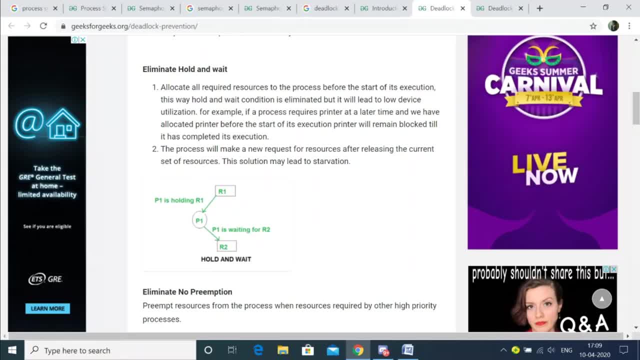 asked me that can we do it again, those algorithms and process synchronization? so hence I did you okay. so another one is the last, like deadlock detection and recovery, and the recommend section. okay, like there are many materials in it, but I'm trying to make it as simple. 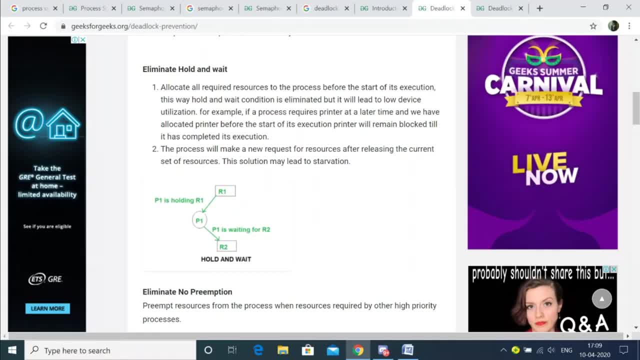 as possible, because these things are very technical, if you have seen also, isn't it? so that's the thing, like I am trying to make as more much as simple. there are many numericals also. we will be dealing with algorithms in questions also they are, so that's why, first you, 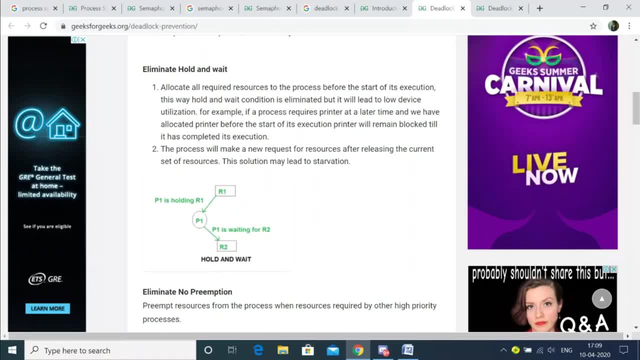 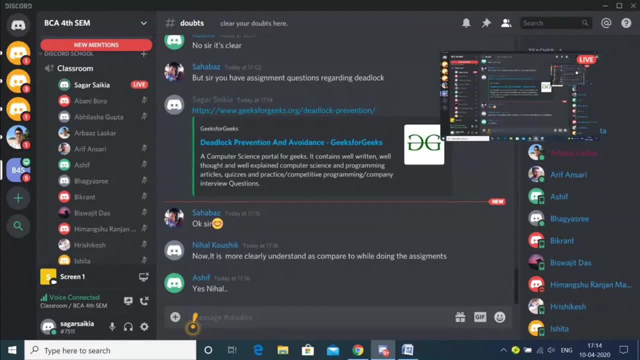 have to know the theory, how it works, and then you have to know the okay, what is the main concept behind? so, accordingly, you will be able to answer. so let us finish this today, and then we can stop. it's very small, only will be done. so the last one is: that means deadlock. 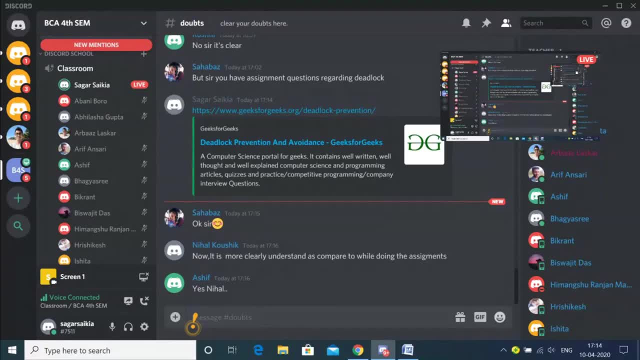 detection and recovery. that means deadlock has occurred, we have to detect it and then we have to recover from that portion. okay, so from here certain question comes. like you have to draw resource allocation graph. that means through that graph you have to find out whether the deadlock has taken place or 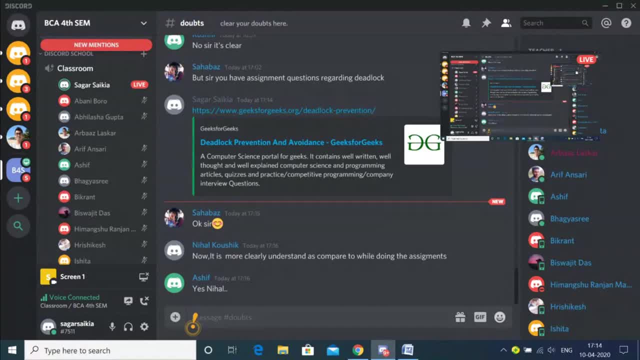 not how to draw the graph. again, there is an algorithm, so we will be checking in other classes. okay, so let's say, for example, in this diagram, how do we know that deadlock has taken place or not? so in this case, for deadlock detection, we can run an algorithm to check for cycle. 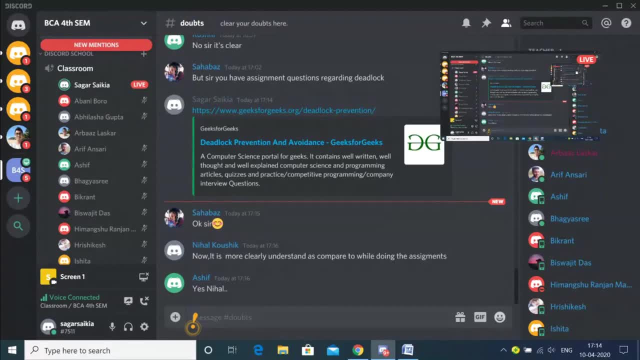 in the resource allocation graph. so presence of cycle in the graph is sufficient condition for deadlock. so do we have cyclic pattern here? yes, we do have. if you look it's complete cycle see. it's going on and on. there is no break. where it will stop we? 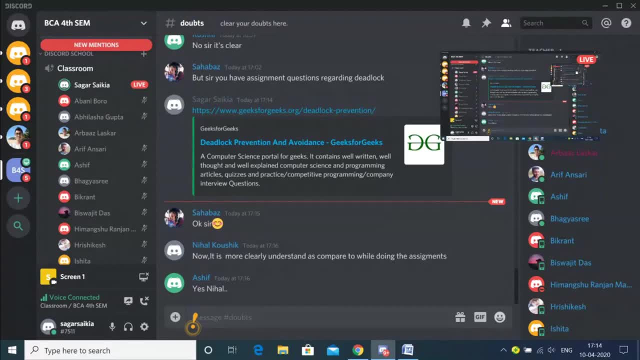 don't know. okay, so such kind of condition would it take occurs, we say that deadlock has occurred. so how to drop this graph? also, I will teach. okay. so in the above graph resource one and resource two have single instances. that means the resource one is having one. 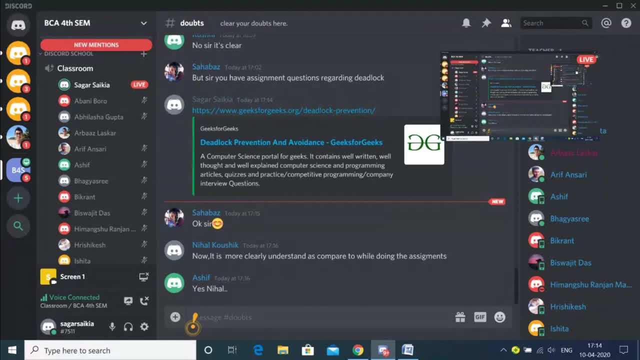 instance process one, and resource two is having another instance, process two. so once i see here what is the cycle here? the cycle is: r1 is going to p1, p1 to r2, r2 to p2, again to r1. so from where we started we are coming back again. so here we say: 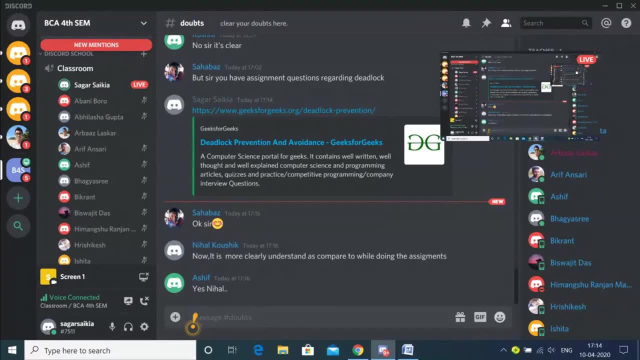 that the deadlock is confirmed, then there may be, there may be multiple instances of resources. okay, so detection of the cycle is necessary, but not sufficient condition for deadlock detection in this case. the system may or may not be in. deadlock varies according to different situations. okay, so if suppose we are unable to get direct cycle, then also there may be deadlock. but whether it is there, 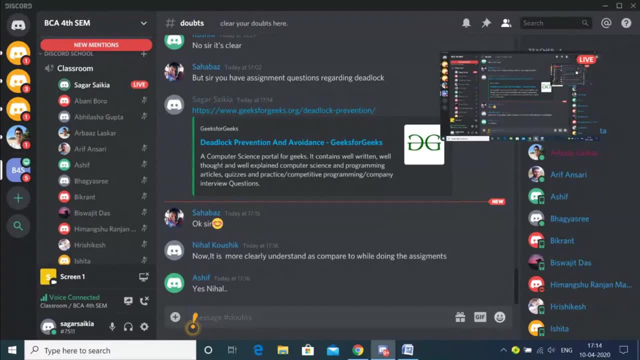 or not, that we we will not be able to say with certainty. okay, but if there is a cycle, we can say that a deadlock is detected. now, if suppose certain situation comes up, then how do we do? because dealing with deadlock is very much time consuming, even space also, like we have seen. 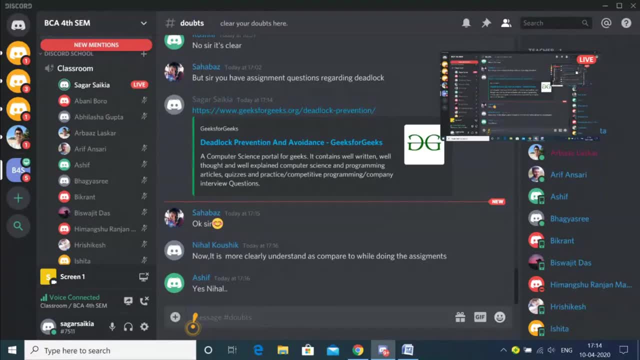 maintain the various information. keeping track of all this information is very much time consuming, even to space consuming as well. okay, so there may be two things. one is killing the process altogether. that means kill all the process, okay, which is involved in the deadlock, that cycle. that cycle has to be finished. so how will we finish? we 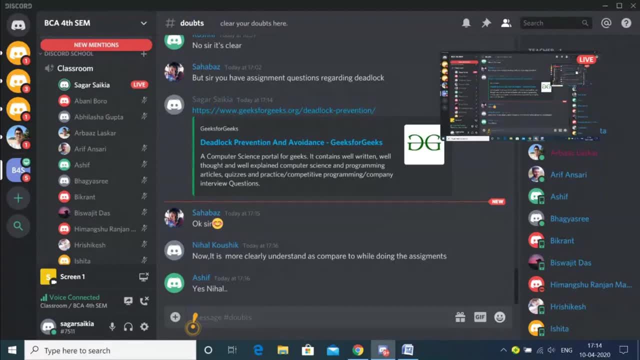 have to kill all those processes which are responsible in the deadlock. that means, whoever processes have formed the cycle, kill them. okay, so killing process one by one. after killing each process, check for the deadlock again, keep repeating the process till the system recovers from the deadlock. so what has happened? what we need to do is: if suppose the deadlock has happened. 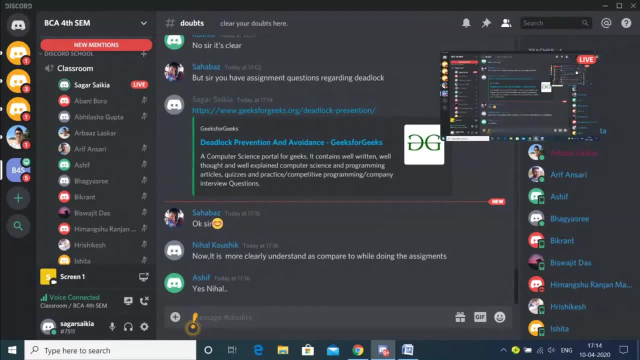 we have to check for which program. basically this, uh fix. i mean to say we are unable to do any work, so we have to kill it. we have to keep on killing one by one till the system regains back. that means it can do its work normally. resource preemption: okay, so resources are preempted from the processes. 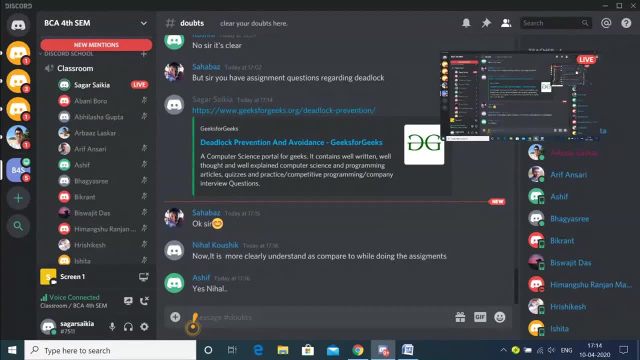 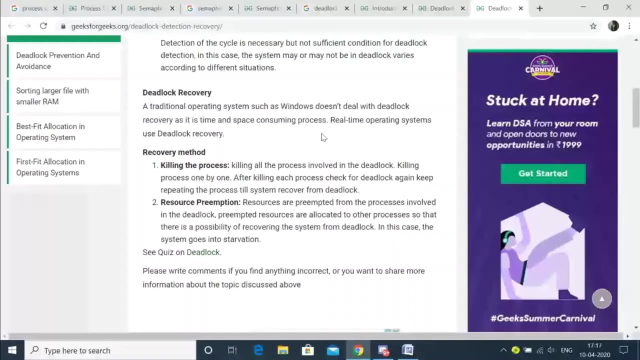 involved in the deadlock preempted resources are located. okay, so here in this case, what do we do is is: can we have like resource preemption? that means, if a process, let's say in this case um this, because this resource was requested for p1, so what we can do, sorry, sorry this. uh, who? yeah, sorry, process, one was requested for requesting. 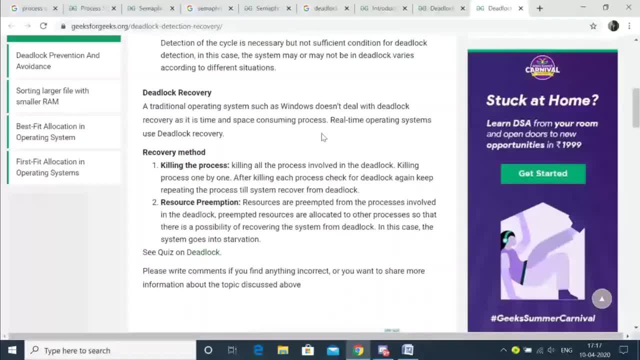 for resource two. so because of this also it is creating a deadlock. because of this resource also is creating a deadlock resource one. so can we remove this resource two and whoever wants it, who wants it? process one wants it. so it's okay, remove this resource two from process two and 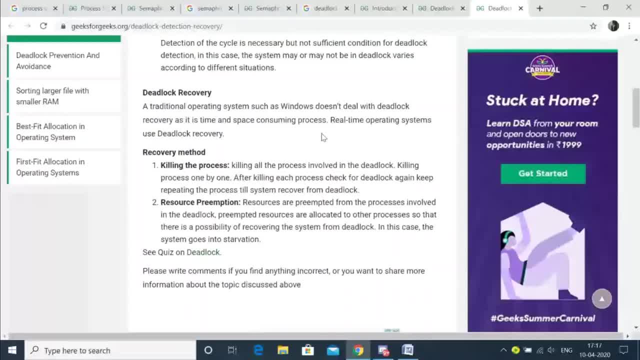 ultimately remove this one, this arc, you break it and ultimately link an arrow to the deadlock. from resource two to process one, that means we are giving resource two to whom to process one. so that way, resource preemption, that means we stop wherever the process is getting the resource we. 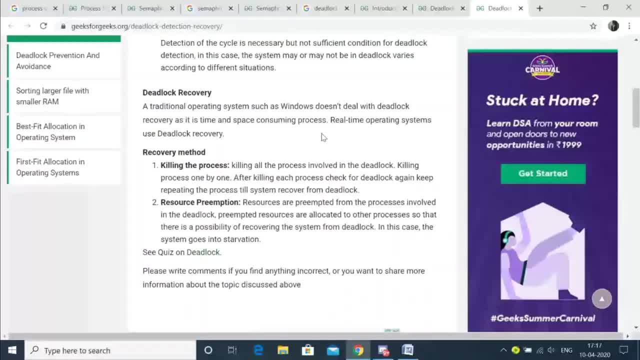 take it off that resource and give it to some other process, so that way that cycle will be broken and finally we will be able to end this deadlock. so any questions? hope. my classes it is helpful, i don't know, but my classes it is helpful, i don't know. but 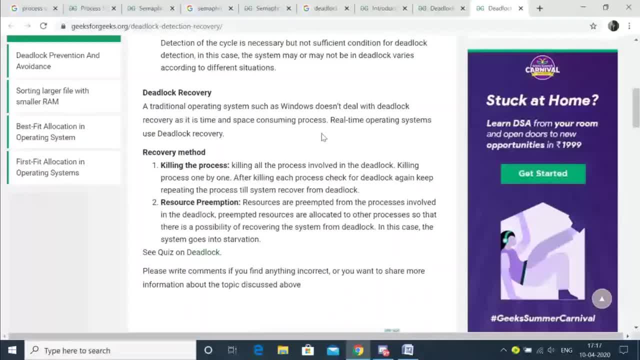 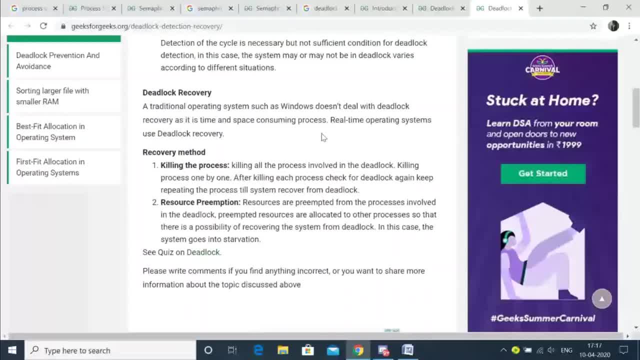 that one maybe till when it reopens, so that one maybe till when it reopens, so that one maybe till when it reopens. so maybe the non-verbal communication again You.